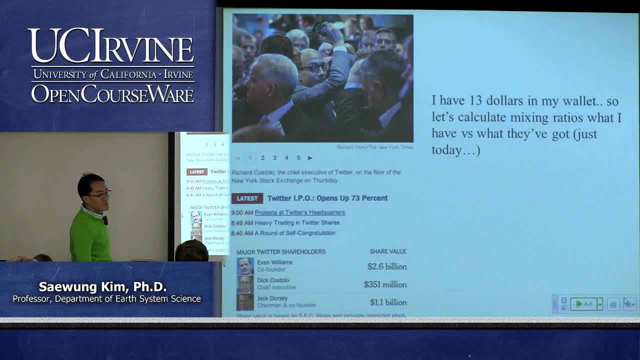 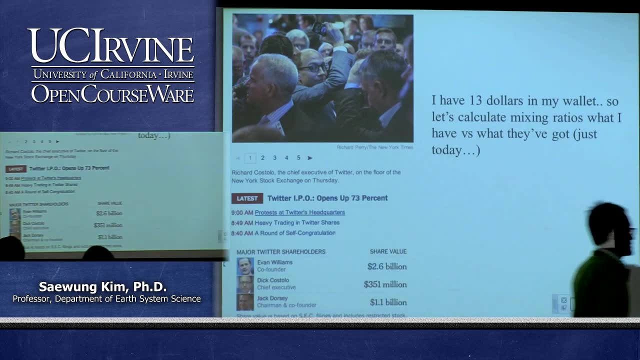 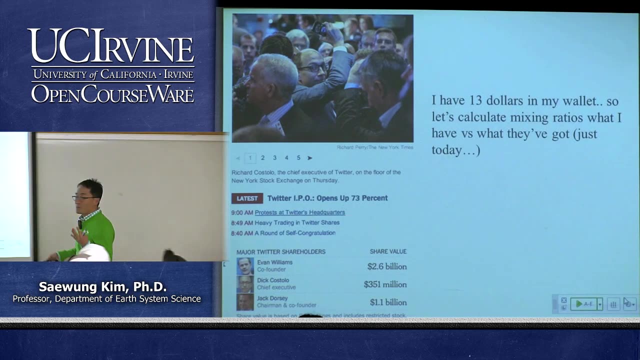 So they got just today this much of money And then I opened my wallet and then take a look at how much cash that I have. I got, yeah, $13.. So this is, by definition, you can just think of this as the number, density, number of the molecules of air in given volume. 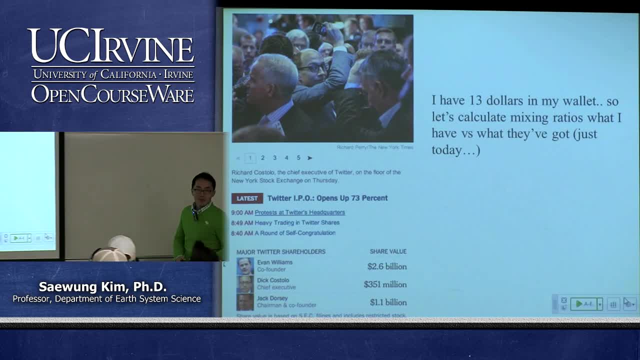 okay, So I will try to calculate mixing ratio of my tiny tiny of money. Okay, So, basically, I got the number density in this amount of money compared with this big money. okay, So that's billion and that's million, right? So this guy right here? co-founder of Twitter. 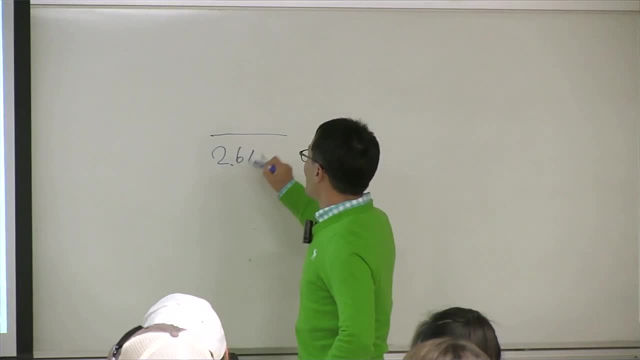 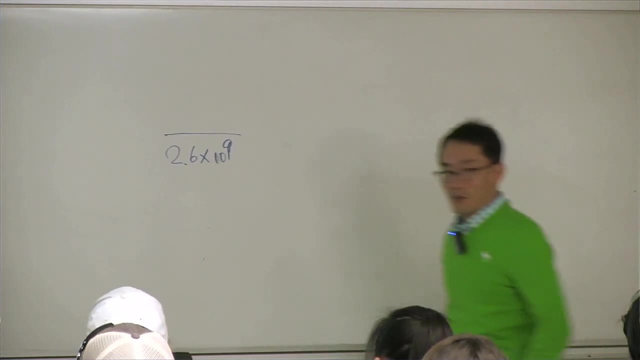 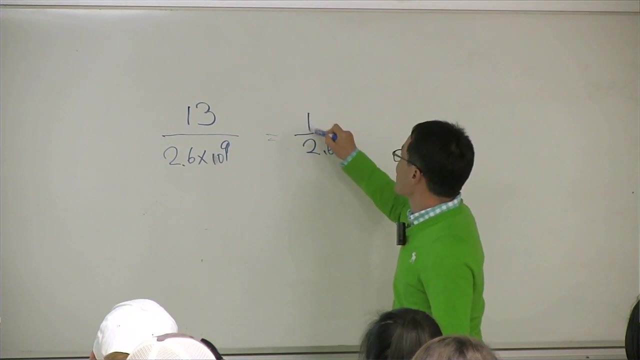 got how much money? 2.6 x 10 to 9,, by definition, billion Dollars today. how much? I have 13,, right. So 2.6, 13, 10 to 9.. All right, 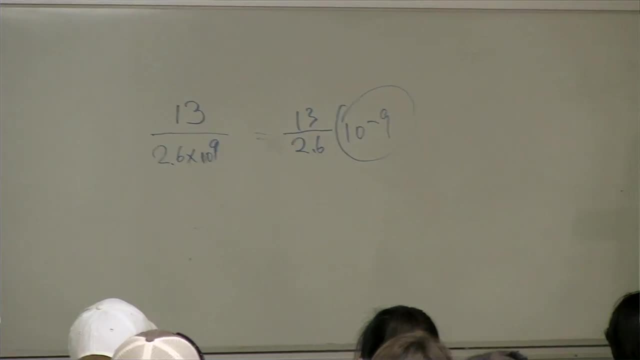 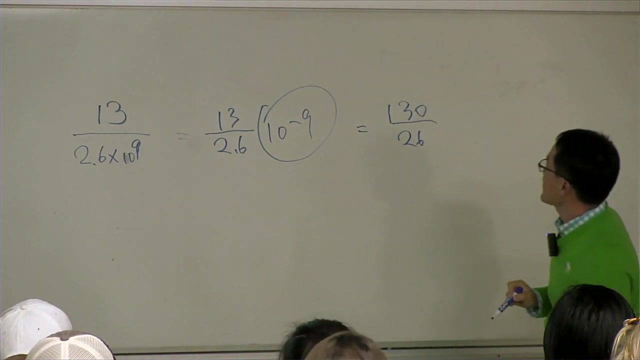 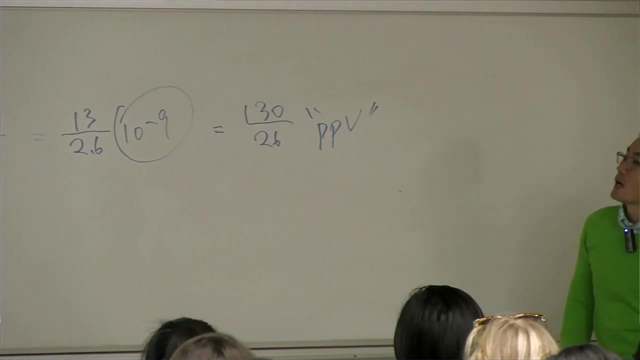 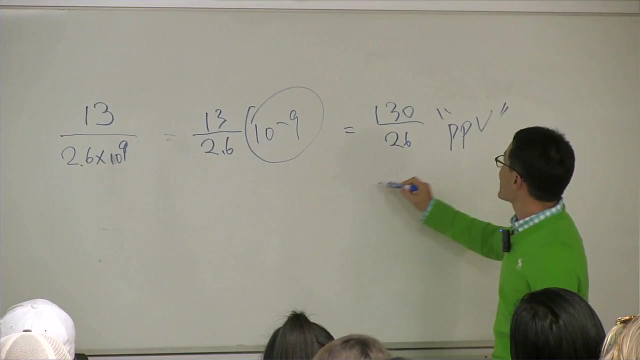 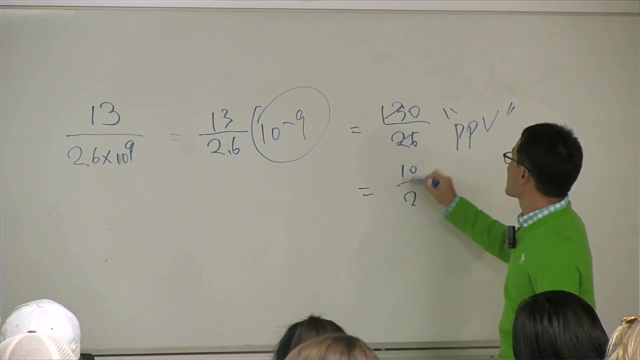 All right, but that's, by definition, parts per billion, right? So let's see 26,, 113, and then we can just call it PPV here, If we assume dollar is the molecule. so what is this thing? So this is basically 13,. 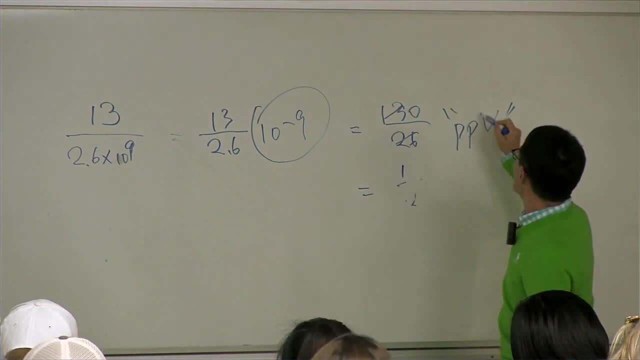 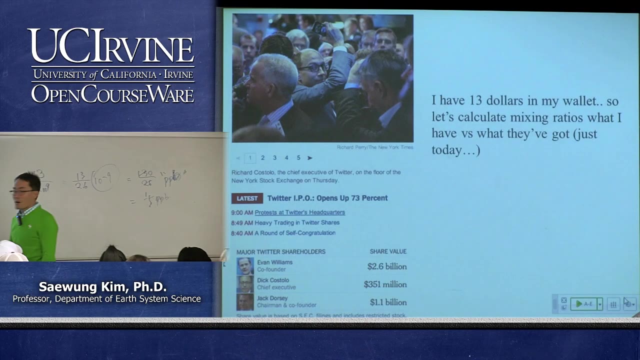 so basically five PPV. So if you assume, then dollar bill is their molecule. compared with this guy's just today's income, the money I've got in my wallet, is five PPV. Okay, So how about this guy, this smiley guy right here? 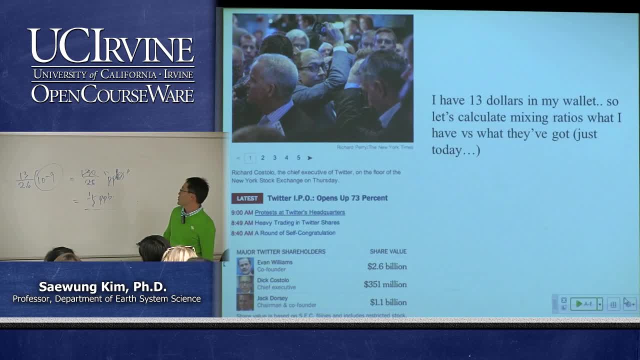 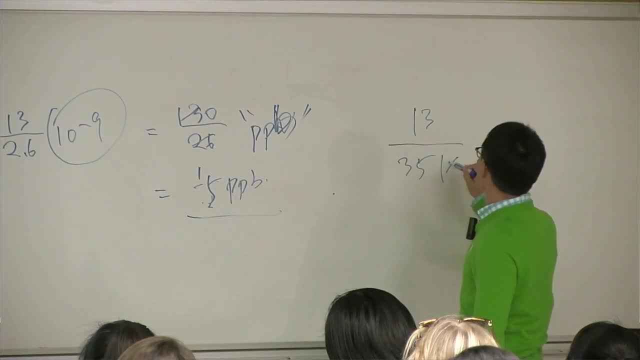 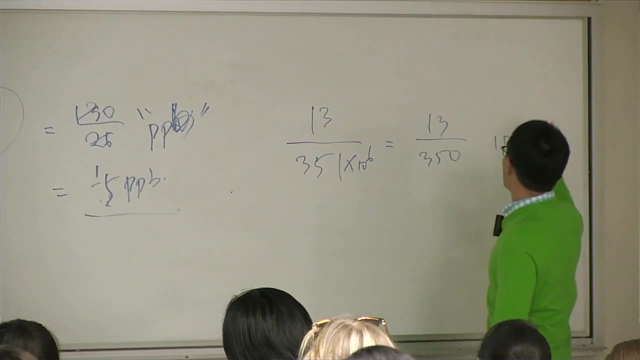 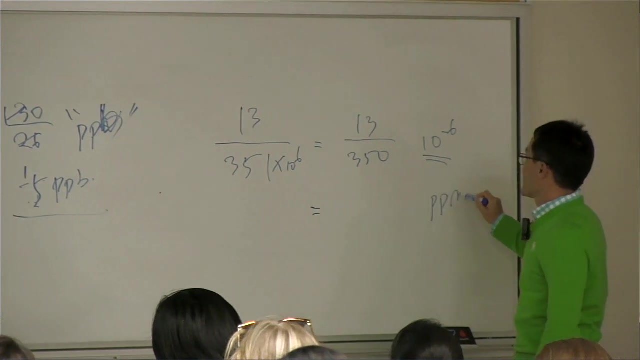 He has under $351 million today. So 351 minus 13, 10 to six. So 350, 13, 10 to minus six. So that's, by definition, PPM. right Now I need a little help here. 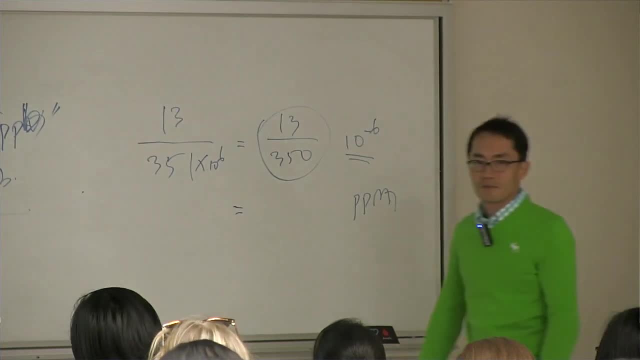 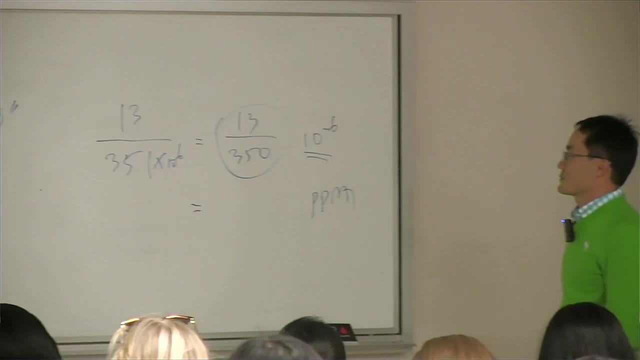 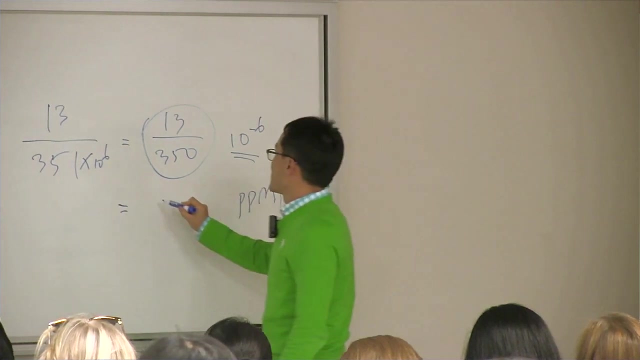 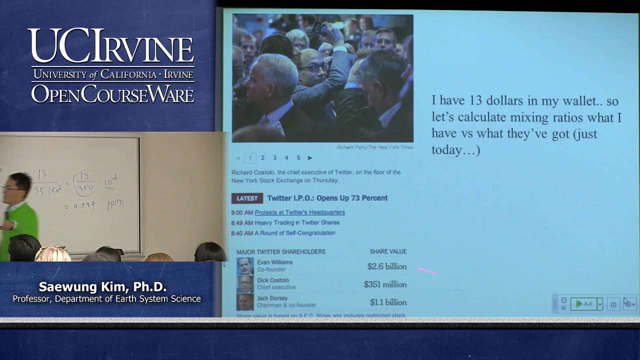 What's the number? Anybody has a calculator, a computer: 13 divided by 350? 0.037.. 0.037 PPM, right, Compared with this guy right here. So basically what it can do even is that, basically this is. 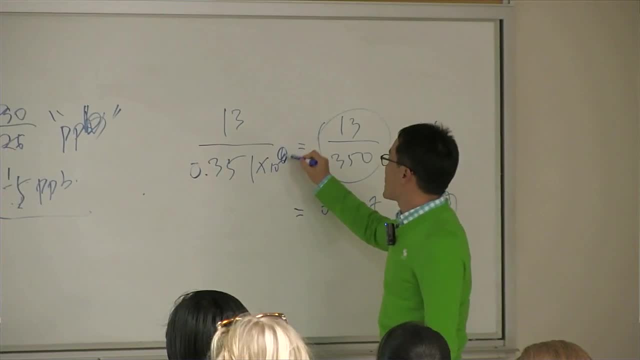 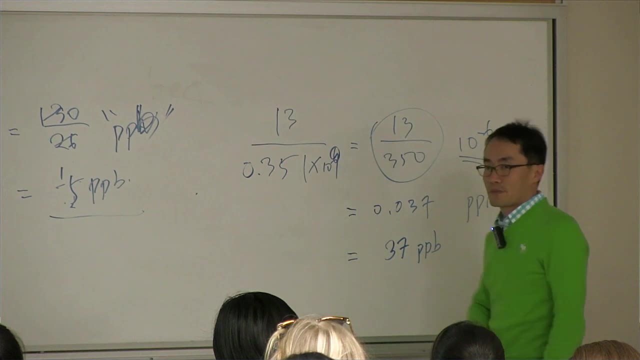 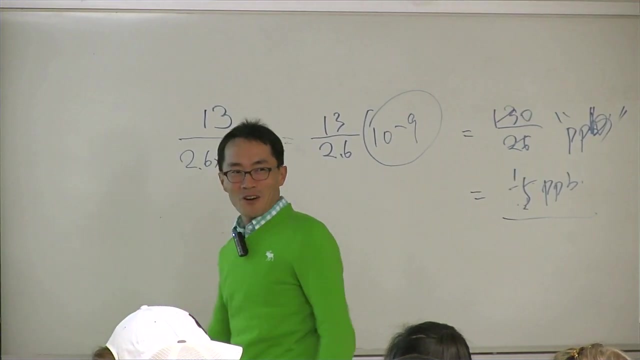 0.351 times 10 to nine, then this is going to be 37 PPV, right? So let's get into some science part. So you guys are very excited when I talk about money. and then let's get into a molecule part here. 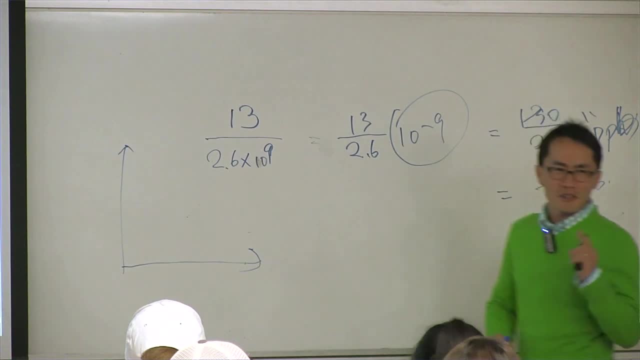 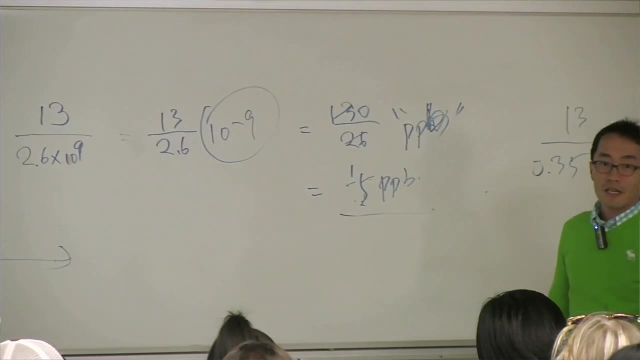 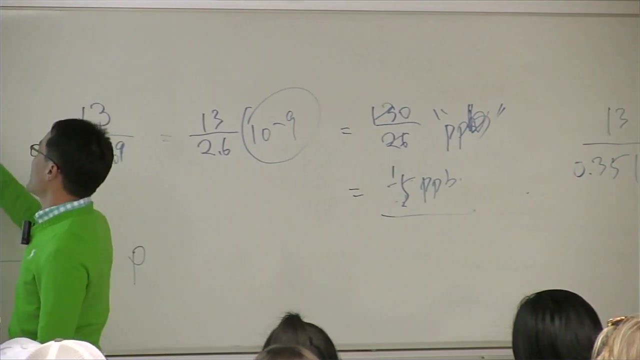 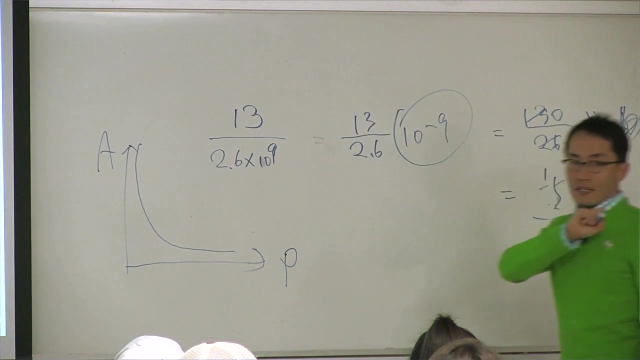 So we talked about. so I think one of the exact question was about: what is this? What is this? So we talked about why EPA regulate ozone concentration in mixing ratio, not number density, right, So pressure and altitude. And then we know that pressure decrease exponentially. 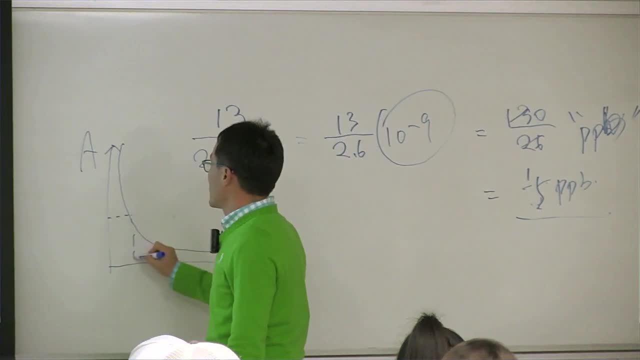 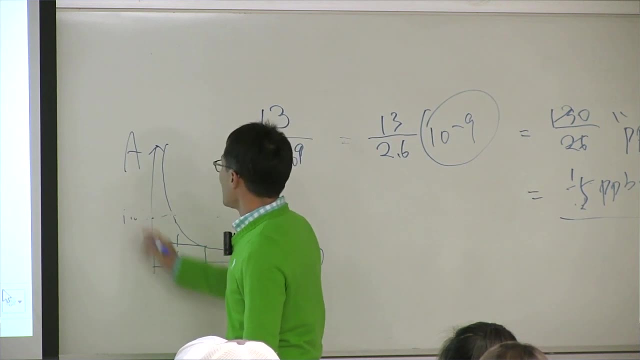 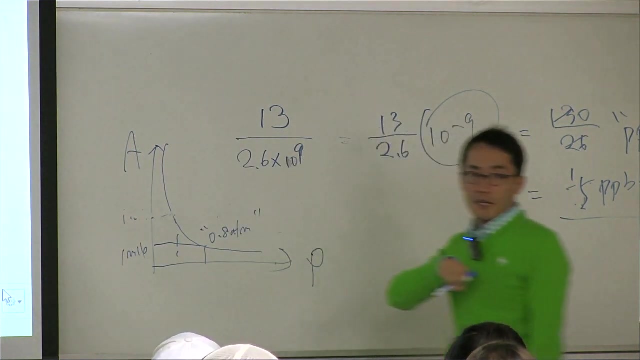 as you go up high, right. So that's why in Denver, which is one mile altitude, has about. it shouldn't be about here. this isn't right. It goes higher. one mile of altitude has 0.8 atm, so it's 80% of air molecules in given volume. 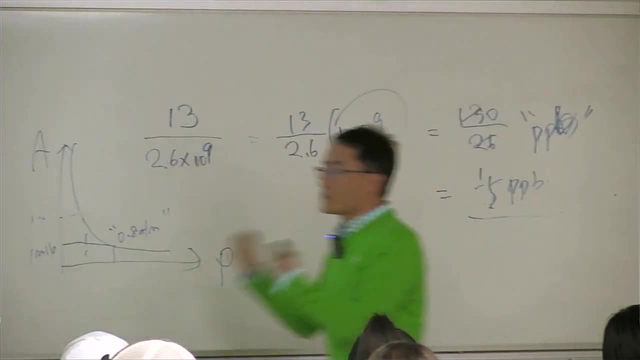 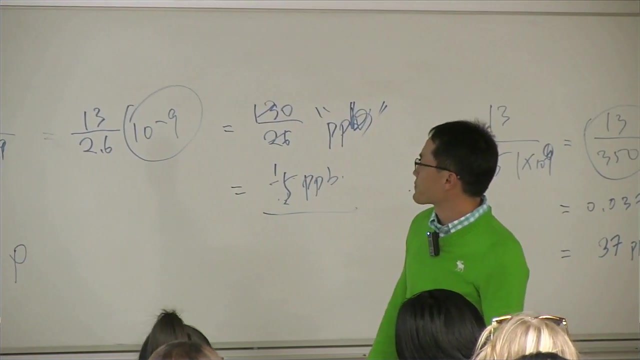 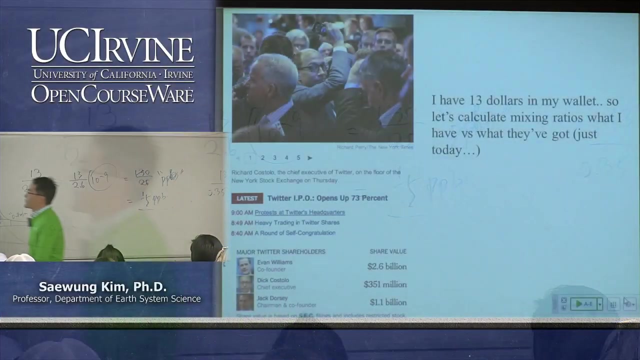 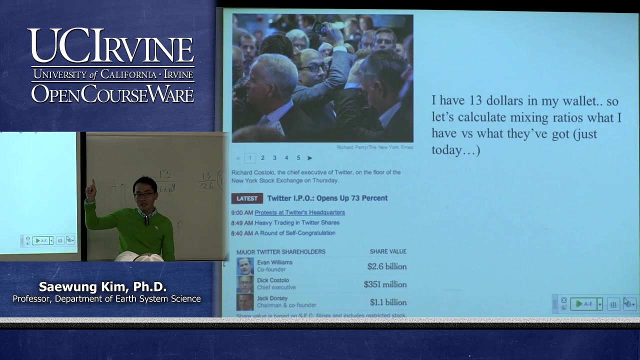 So basically you can think that different places has different pressure. so to compare evenly, we need to use this mixing ratio scale to kind of leveling the different number of air molecules compared with my tiny, tiny amount of money that's sitting in my wallet. 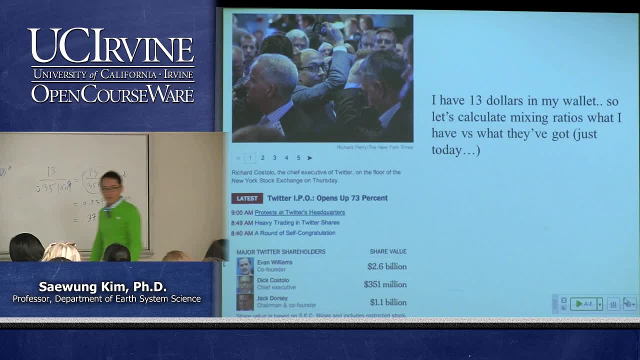 So that's the main reason. Is that this money analogy make you help to understand? Do you understand better in terms of mixing ratio, Or it just makes you even more confusing? This is better Or worse, I don't know. I was trying at least. 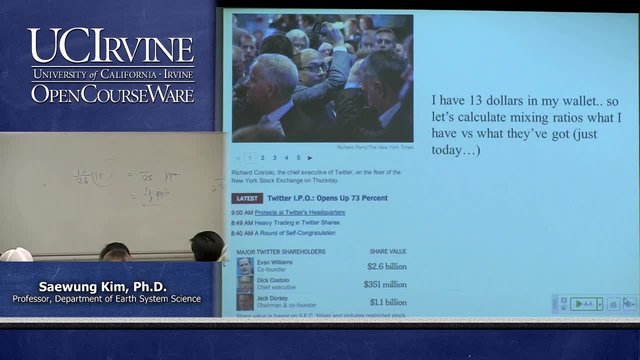 So that was the answer. And then I got a question about that. is there still we can review the midterm? Yeah, sure, until end of the quarter. I'm willing to review your midterm Midterm if you visit my office during the office hour or by appointment. so come see. 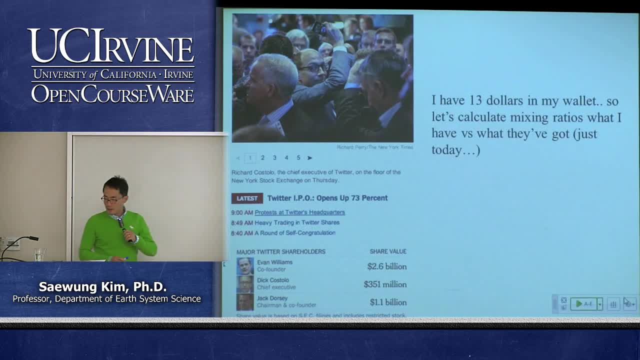 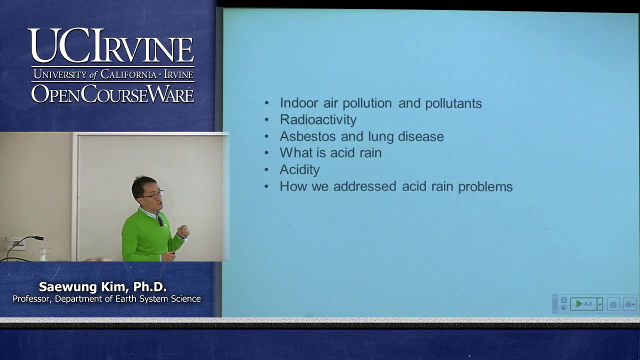 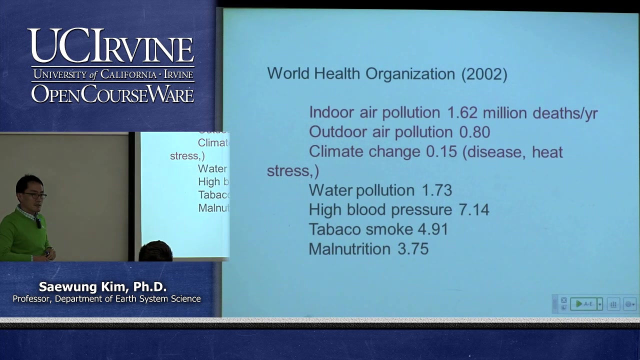 me. if you have any question about your midterm, all right, So let's go at. let me try again. So today we'll talk about indoor air pollution and acid rain. then why we are talking about indoor air pollution? Okay, So if we take a look at statistics and global statistics, then the casualty, the death. 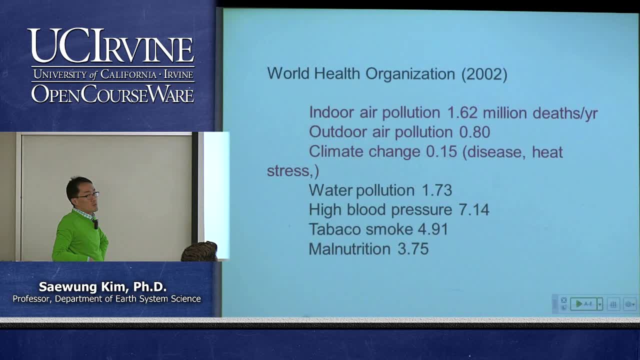 from indoor air pollution are far, much larger number than the air pollution outside that we have discussed so far. Even compared with the climate change, that's far much more larger number in terms of number of deaths per year. So that's very vital part of the air pollution to understand societal, societal implication. 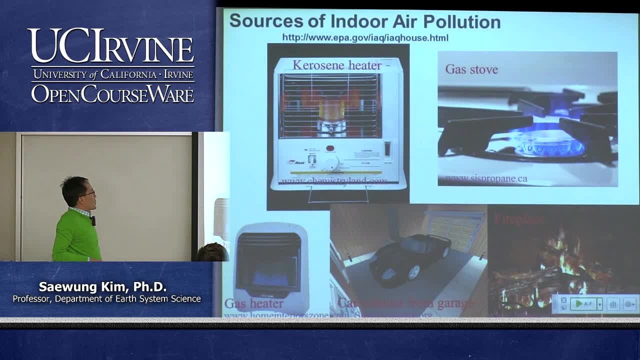 of the air pollution. So there's a couple of figures, photos about this, all burning parts you tend to keep inside of your house. So basically, running engine fireplace, this gas heater and the gas stove and then this kerosene heater. 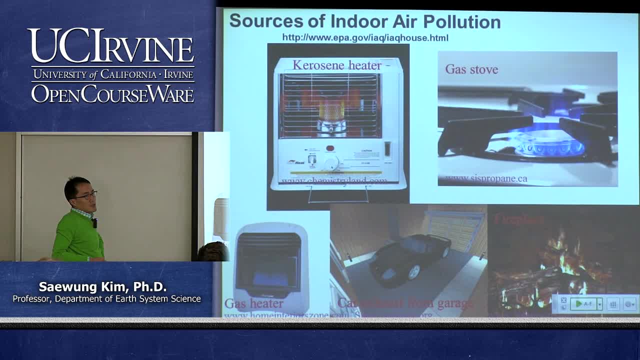 Okay, So what kind of gas species this burning process can emit? you think, in terms of air pollutants, Carbon monoxide, Carbon, what Carbon monoxide? Yes, that's carbon monoxide. So that's basically all this thing using organic compound as a fuel, right? 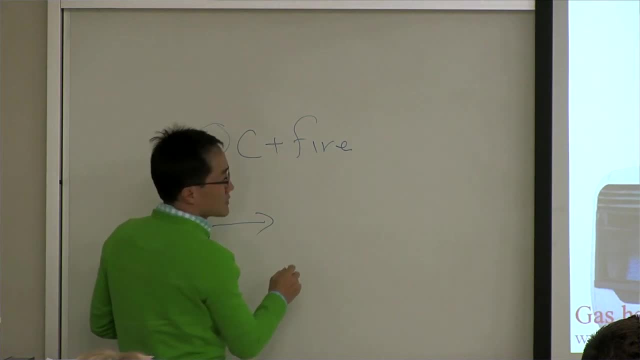 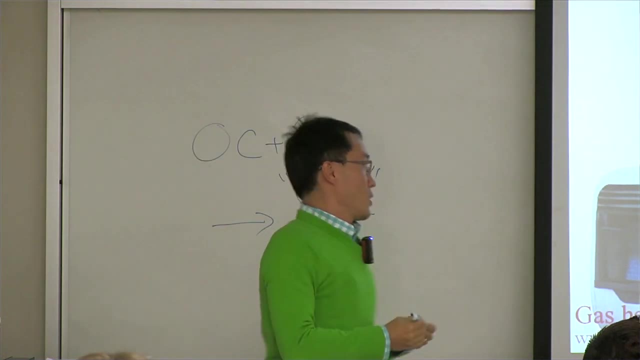 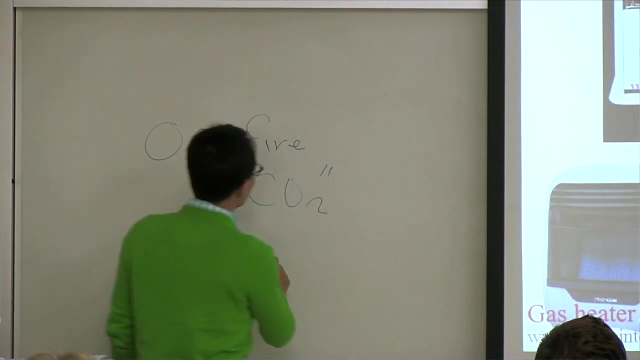 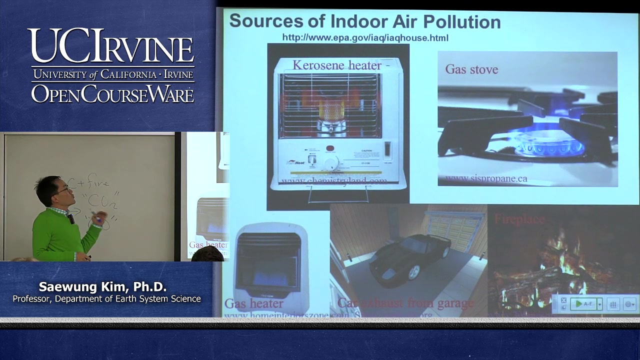 Fire. Obviously, complete combustion is going to emitting CO2.. But usually, right Yeah, Usually CO2 never gets accumulated at higher concentration. that can really bad, harmful to you. But CO which is coming from incomplete combustion can actually accumulate inside of the house. 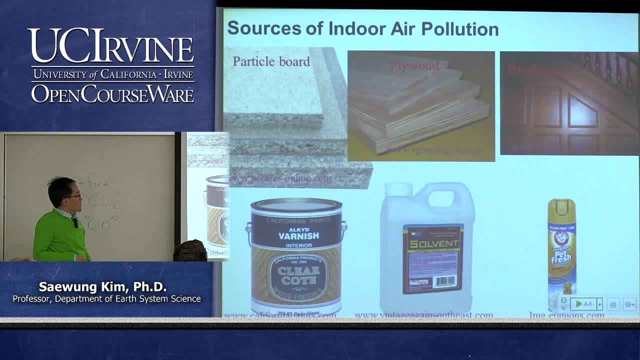 and then they can actually eventually kill you. So that's the some indoor air pollutants, CO. This is important indoor air pollutants. And then in house there's a lot of plywood and then we tend to bring a lot of solvents and then paints, things like that. 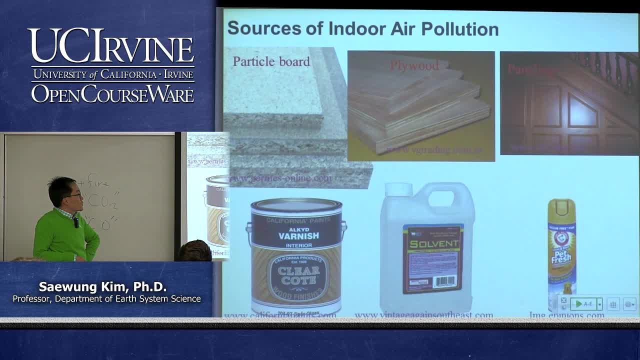 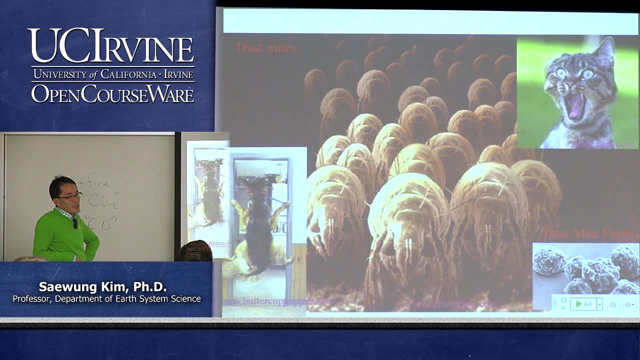 And then those kind of thing can emit VOCs to the atmosphere, indoor air. Then another thing: if you have a microscope and then you know this kind of thing can actually sitting in your pillowcase and your blanket, things like that. so once you go, 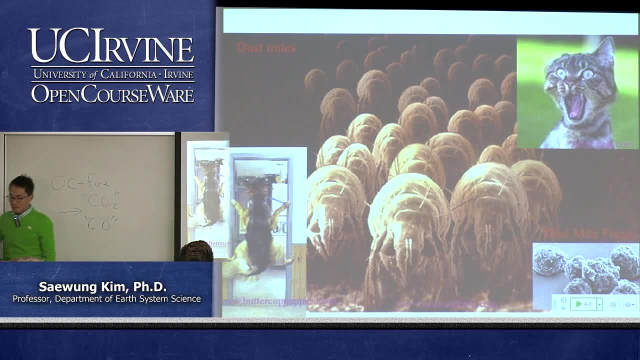 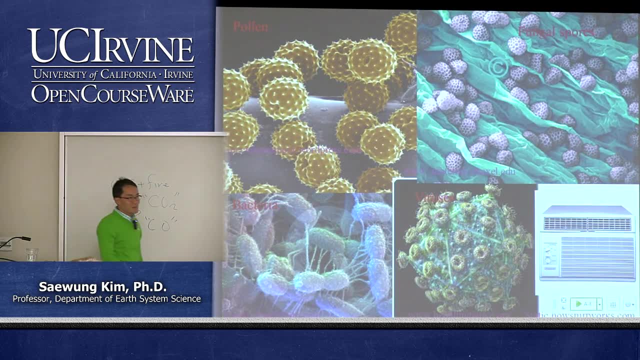 back to house today, Just all just clean it up, wash it out. So that's the message, This just try to make you scary, kind of thing. And then all those other stuff. The sweet, sweet home is actually pretty dangerous place if you take a look at this thing. 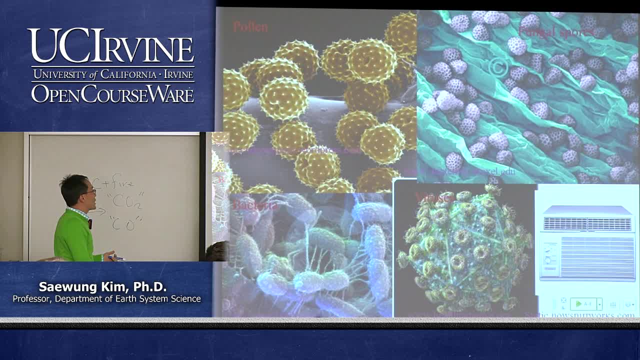 During the spring time, pollen can rolling in your house and then fungus spore, things like that, Even bacteria and virus. Why the the virus? the? it's kind of a why we have a kind of infectious disease. Infectious disease because virus can be traveling through the atmosphere. 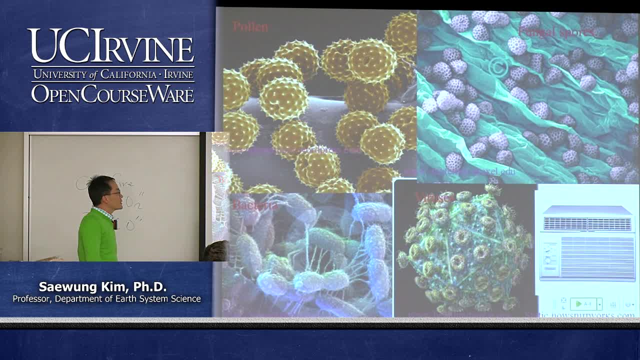 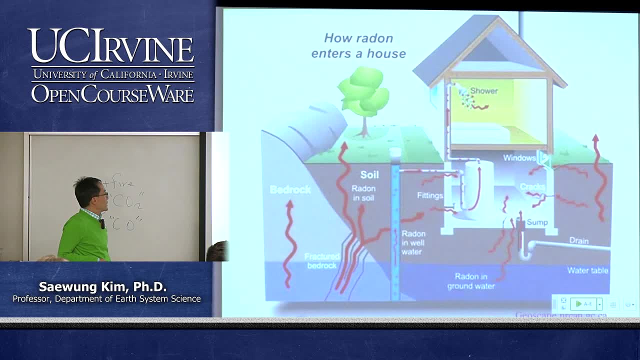 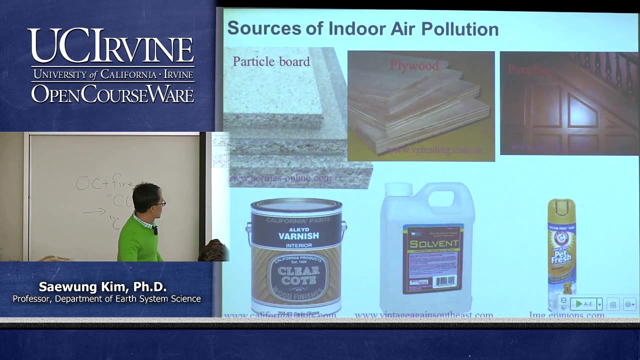 So if you count this kind of infectious disease kind of thing, that kind of infected through the atmosphere, then it can be air pollution too, right, So did I skip that thing. Oh, actually we need to take a look at one thing there. 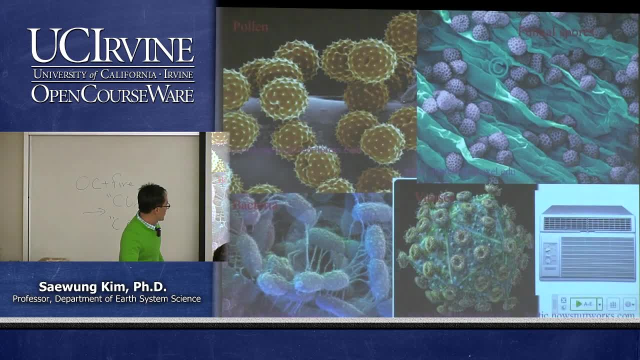 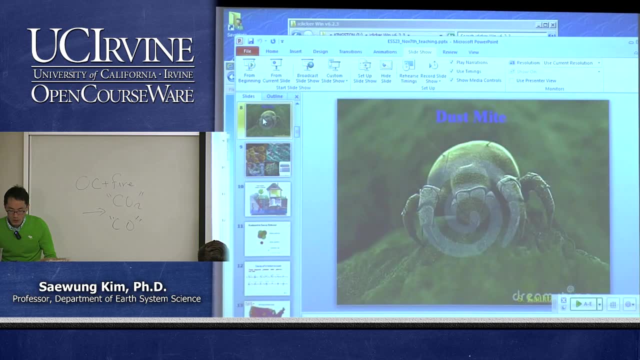 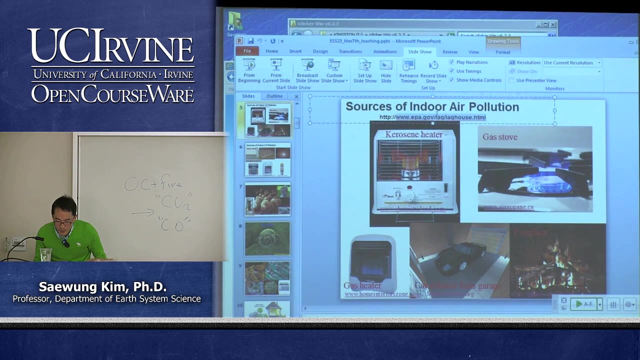 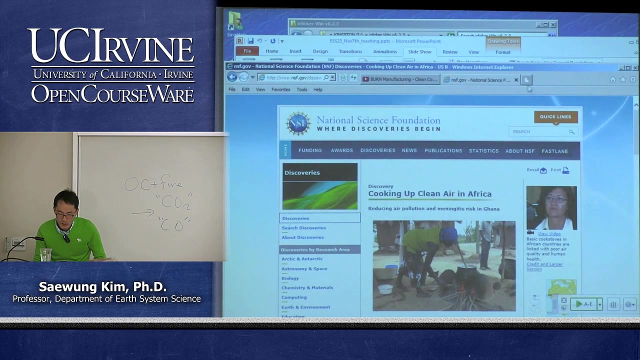 Hmm. So let me actually, Let me actually take a look at one more thing: the website We supposed to be supposed to take a look at the website. Oh here. So EPA has nice website that summarize the source of air pollutants in your sweet, sweet. 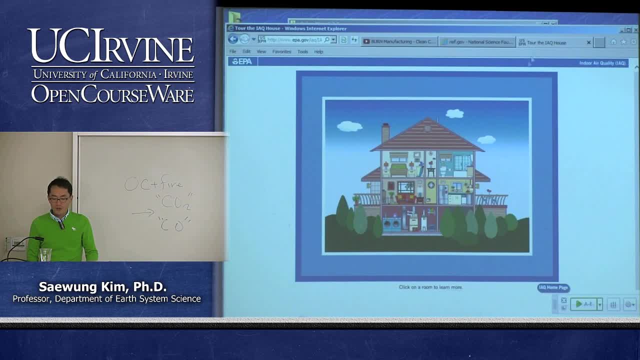 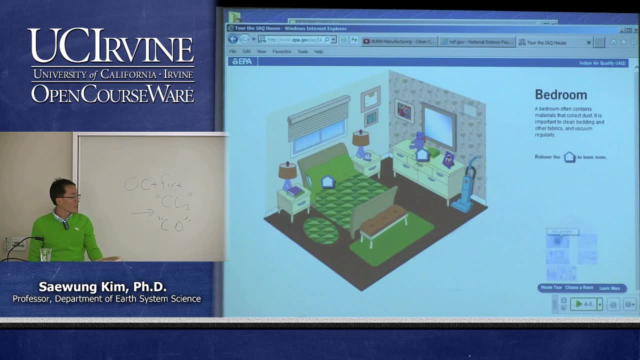 home. So that's this. It's very, very nice looking home. Weather is great. You know the cloud is rolling around very peaceful, But if you take a look at the inside of the bedroom, dust mites that. we already saw that. 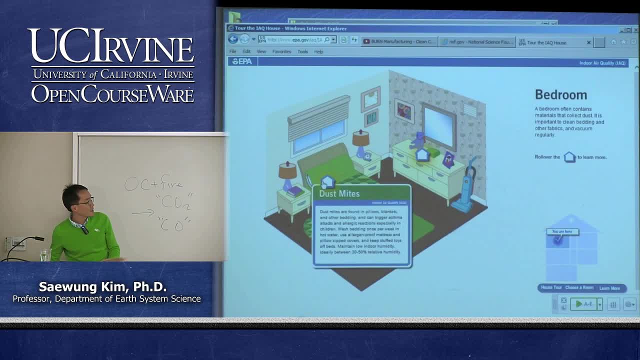 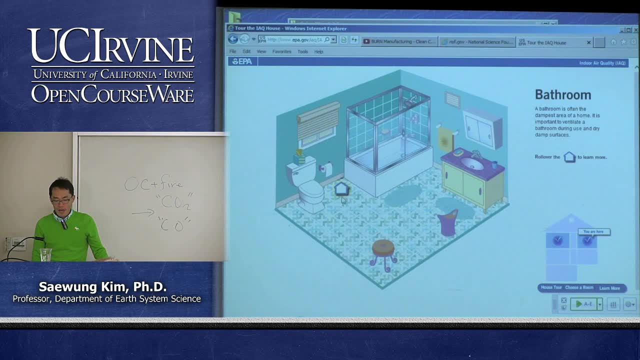 microscopic photos also. your pillow case and your blanket- things like that- has this kind of thing. So this is the bedroom, And then let's move along to the bathroom. The mold can be rolling around. Obviously, this can be bad for your lung. 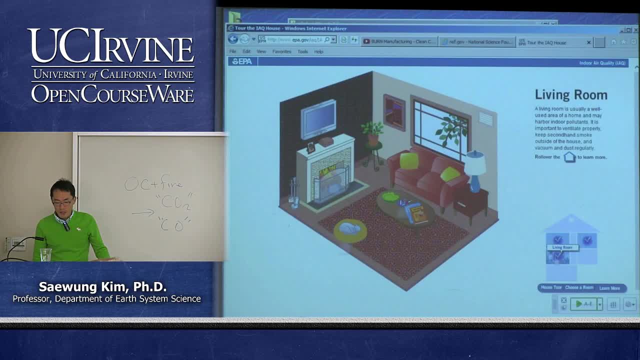 Okay, health things like that- that's one thing. Even in the living room, the carbon monoxide- this nice looking cozy fireplace- you probably miss this kind of thing this time of the season- can emit carbon monoxide, So you want to put some carbon monoxide detector. 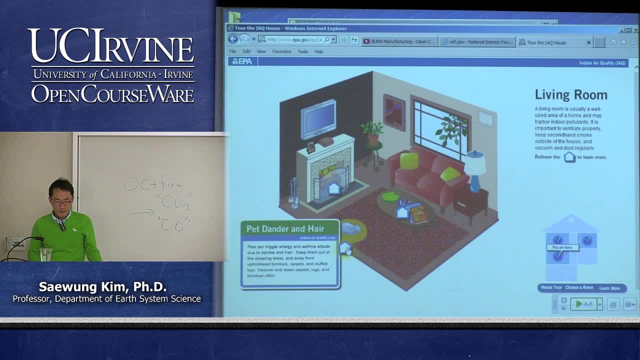 in your house, And then this pet thing has a pet vendor and hair can emit it to the atmosphere- Oh, cigarette. so secondhand smoke can be a big thing, although if you are not a smoker, if you have a smoker in your household. 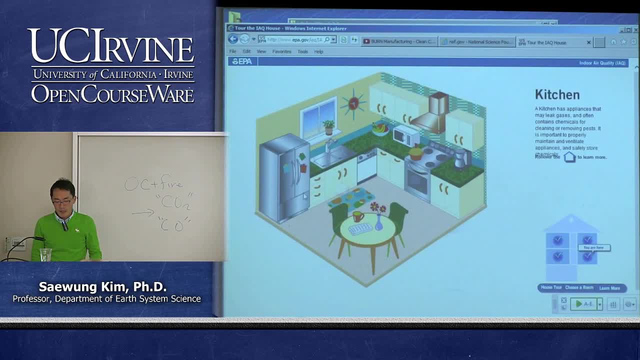 that can actually be bad for you. that can be bad for you. And then kitchen. so even fruits can. some pesticide residue can stay in the fruit. that can evaporate inside of the house because the air inside the house is kind of isolated. 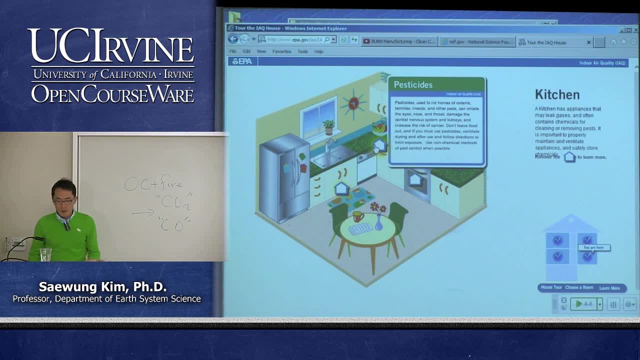 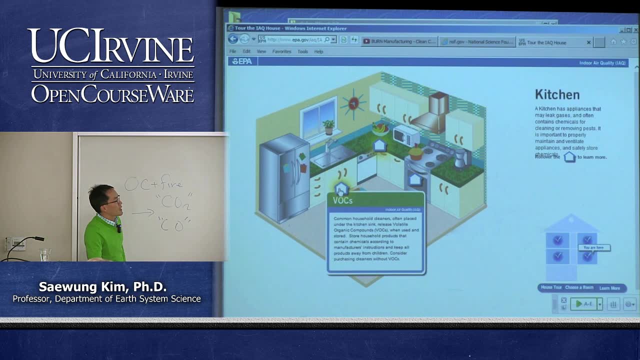 so it can be accumulated. It can be accumulated to the atmosphere, right. So the sink counter- there's some detergent, cleaner things like that. that's actually VOCs, because so once you smell something, that means that there's volatile organic compounds. 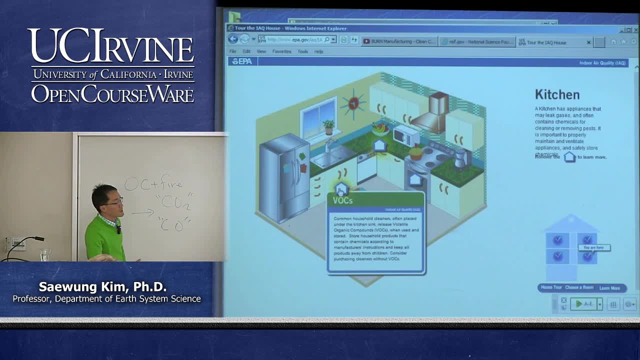 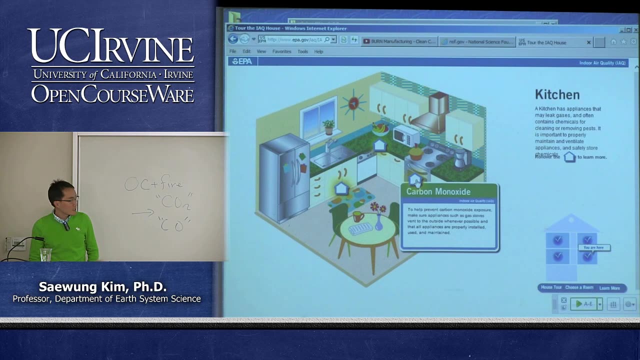 actually reach your nose and then that's how you sense the smell. So this kind of detergent- cleaner things like that- also emits VOCs to the atmosphere. If you are sensitive, then this can be an even problem. So obviously this stove thing. 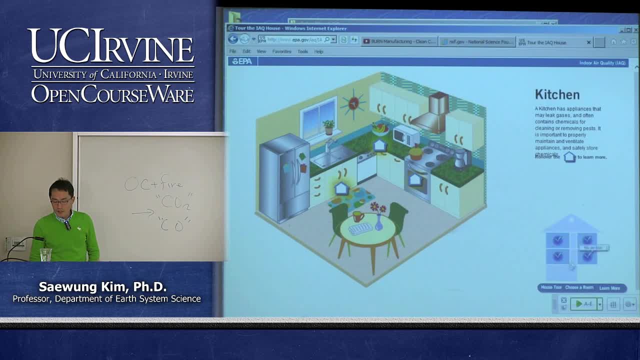 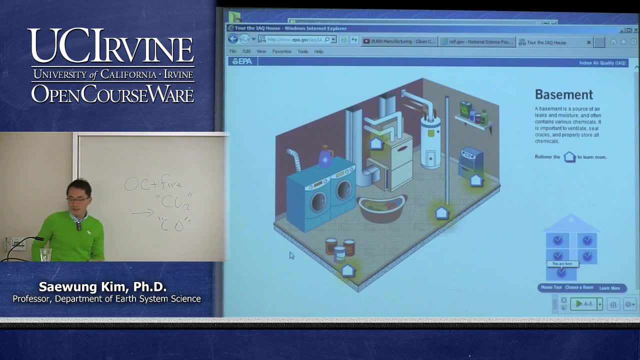 can emit the carbon monoxide too. So this is kitchen, and in California there's not many houses has basement, but most of places has basements, so let's take a look at what can be a potential danger. stop in the basement. 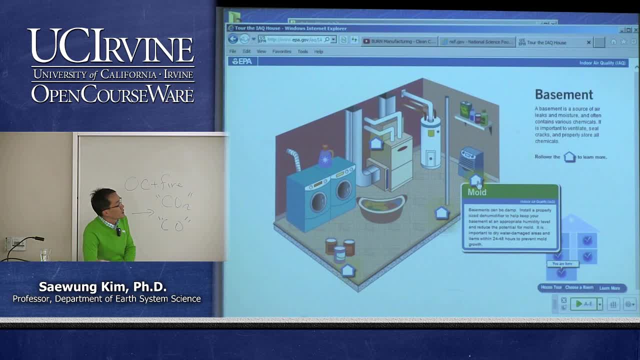 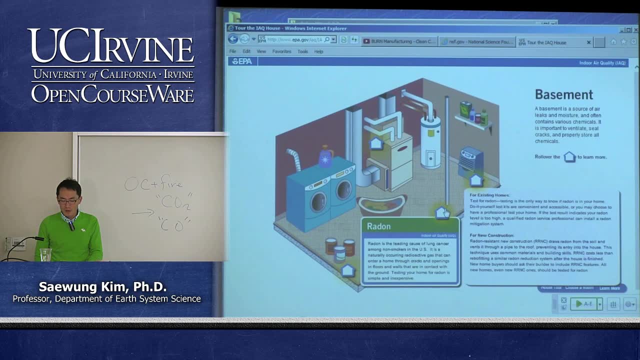 So mold can be, because usually a basement is wet, so mold can be a problem. So what is this thing? Radon. so we'll discuss about radon, especially in the basement. A lot of radon can be smearing into your house. 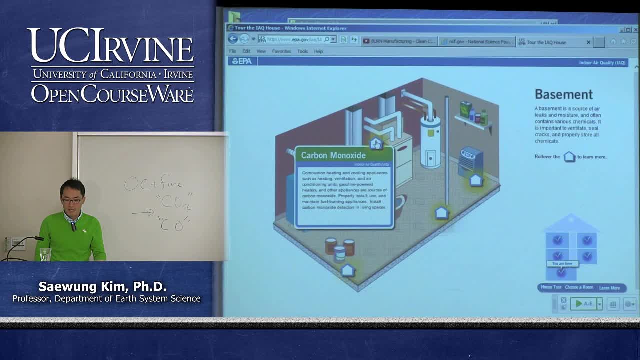 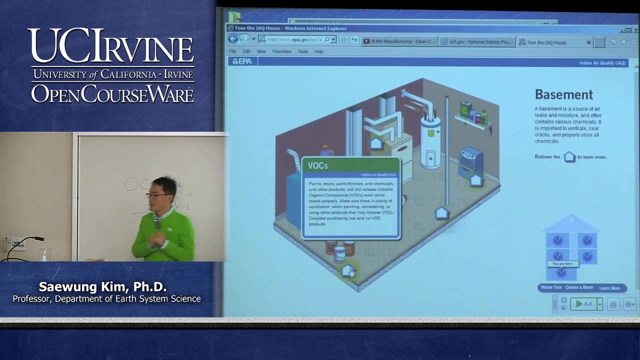 and then this is carbon monoxide. The water heater, things like that can, because that's burning process. again, the carbon monoxide can be coming out from this burning process and then a lot of people actually store their paints in the basement. then that can emit the VOC. 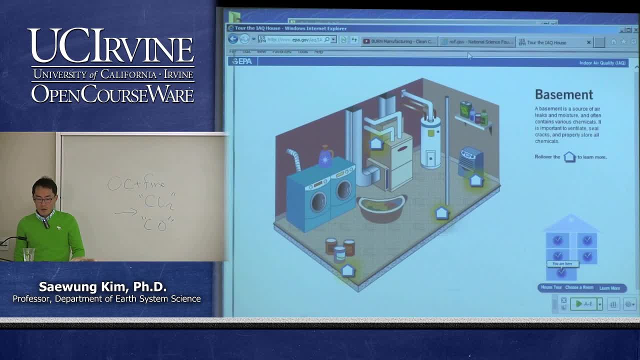 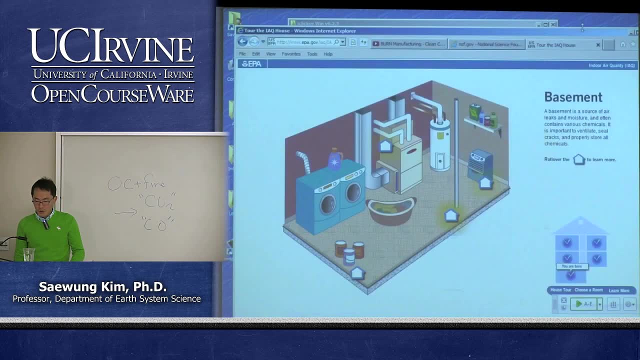 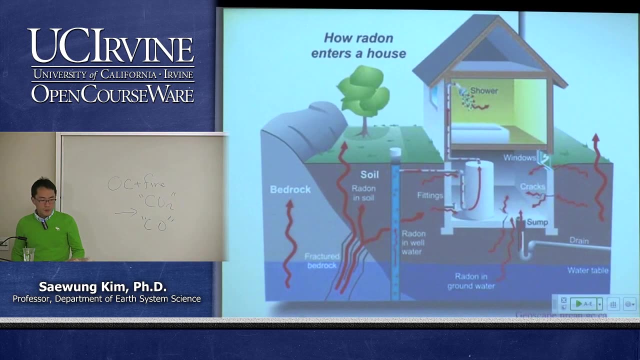 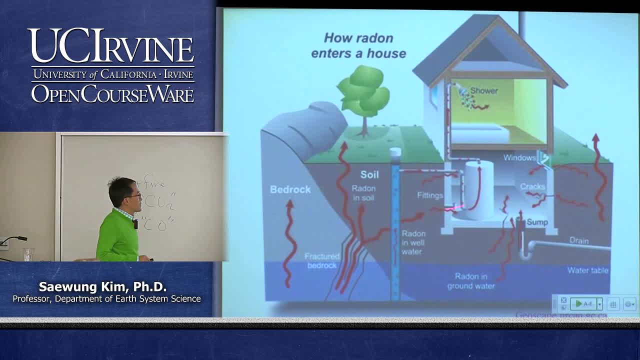 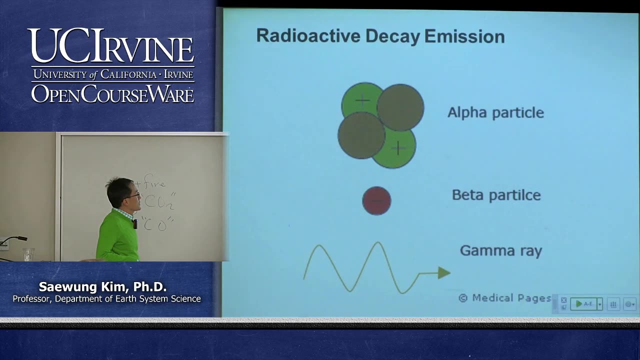 it can be smeared into the space, especially in the basement, and also it can smear into the water line and then it can just get into the house through the water. So we talked about radioactivity. So radioactivity is that basically the atom is unstable. 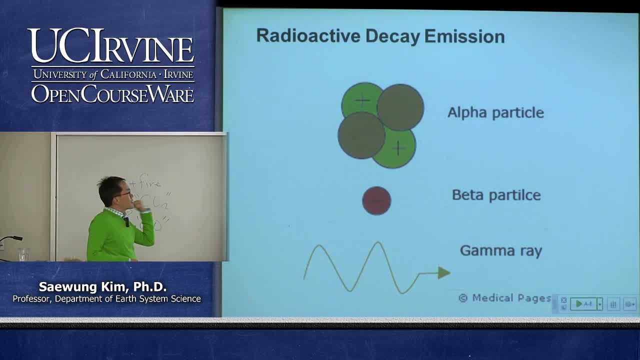 so it decompose to more stable atom and then by that decomposition it's associated with the emission of this energetic particle. there's three energy particle we are interested in. One is alpha particle, which is two proton and two neutron, and beta particle has one electron. 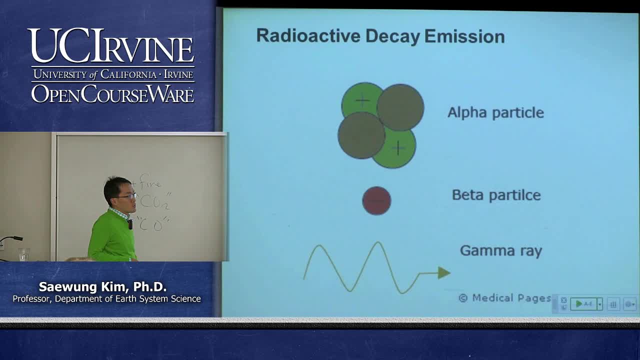 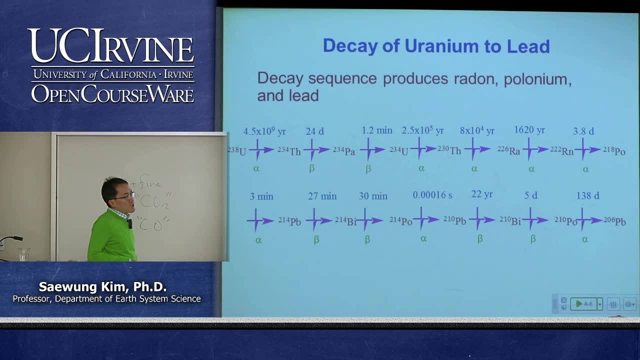 and then gamma is just ray, and the x-ray is one of these thing too. So so this radon is coming from uranium out here, and then this is what is called half-life. So if there's a hundred atom of the energy, 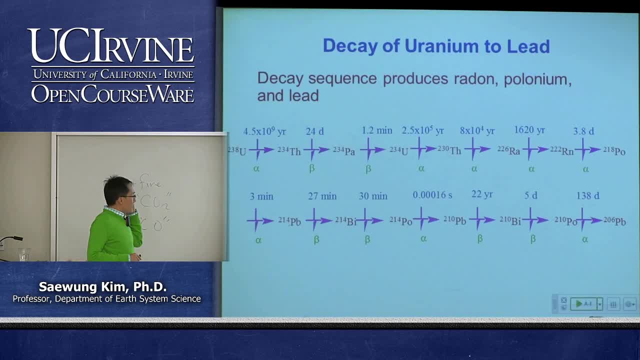 half-life of the uranium-238 is currently right here, then about 4.5 times 10 to nine years, which is 4.5 billion years, then half of this uranium will become thorium and then will emit alpha particle by that decaying process. 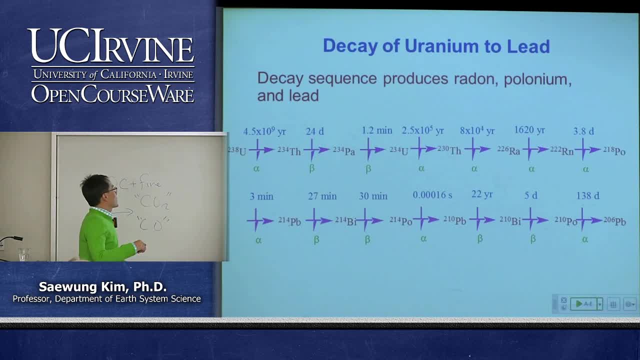 This is how you can read this thing. So uranium becomes thorium, then it just decompose into all the way down to radon. right here, actually right here. This is actually radium. and then this radon, yeah, radon, right here. 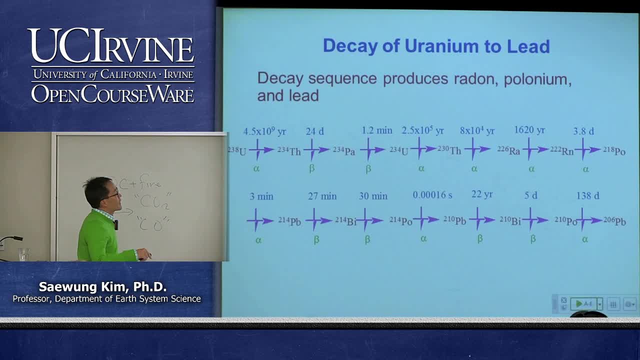 So radon is gas and then that means that you can actually inhale this thing and then it's sitting in your lung. it can be staying in your lung and then about 3.8 days it emits energetic particle, called alpha particle, and then become polonium. 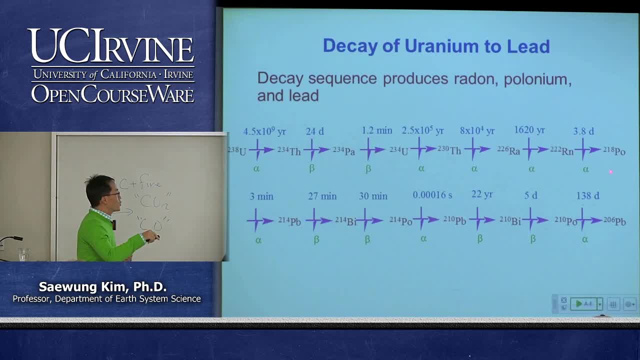 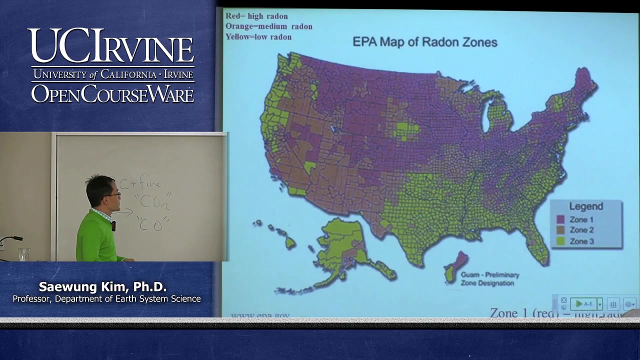 and then about three minutes after that, and then about three minutes after this polonium atom, half of them will become lead. So lead is bad thing, obviously, for your health. so that's why radon is the bad thing in terms of when the radon is smearing into your basement. 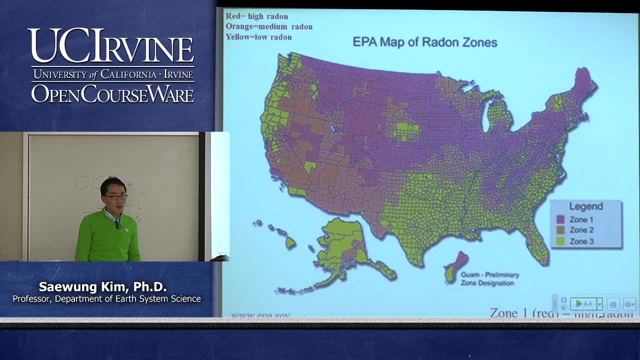 So this is radon. EPA actually did survey where the high radon exists, in terms of the basement and then in the rock, things like that. So usually high radon is observed in Rocky Mountain region, then mostly mountain region. 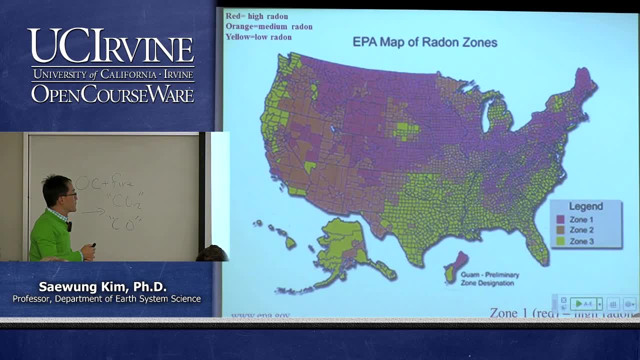 and usually California is relatively safe in terms of the radon pollution, So Colorado is right here. so when I live in Colorado, we have to buy a house, we have to buy a house, we have to buy a house, so we have to buy a house. 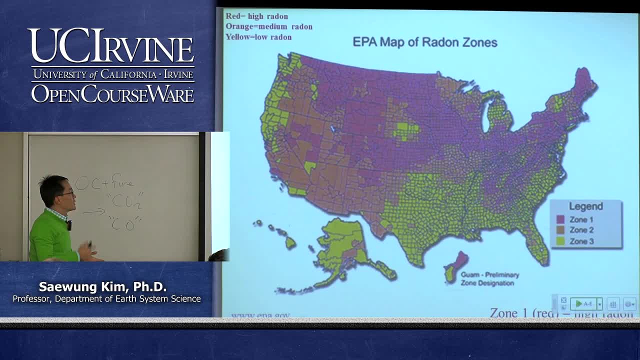 we have to buy a house. we have to buy a house, house out there, and then we actually did so. I think state law mandate that, having lead on survey on the basement and then we ended up having high lead on concentration on the. 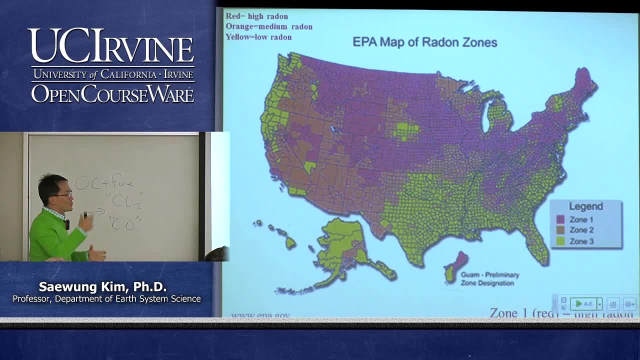 basement. so we- I think we paid like $800 to set the system that can ventilate the air in the basement to the outside and then the lead on level gets much stabilized. so don't get freaked out if you move to someplace else. try to buy a house when lead on level. 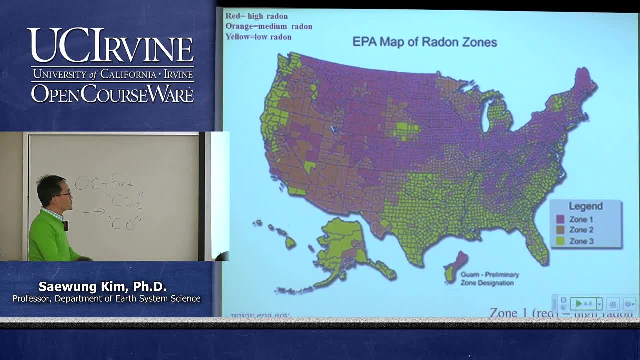 is high, then don't get freaked out. you can easily install some ventilation system that can knock down lead on concentration on the basement, but if you are thinking to move into some place- this red zone, that high lead on concentration- then you've got to. 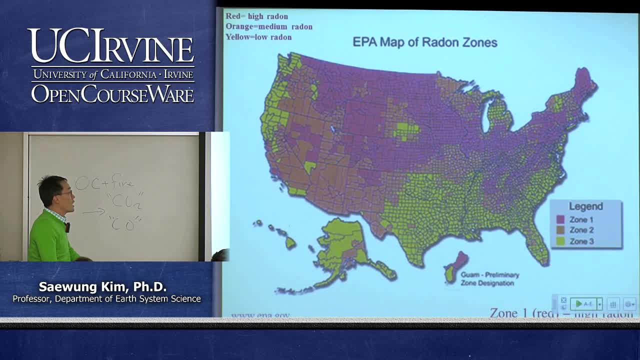 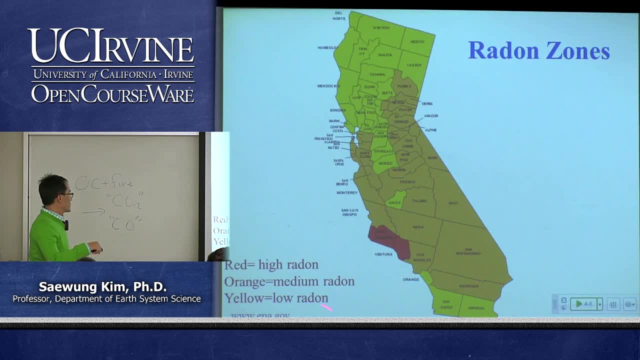 definitely check up the lead on concentration if you plan to buy a house or rent a house, things like that, okay. So this is a lead on zone. Basically it's relatively safe. so yellow is low lead on and then red is high lead. 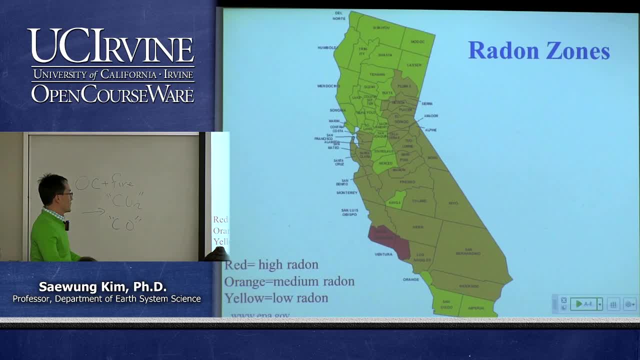 on, except Santa Barbara region, I don't know. but if you plan to move out here and buy a house- mostly I think houses in California doesn't have basement, but if you just move into basement things like that in this area- you've got to check out that lead on concentration. 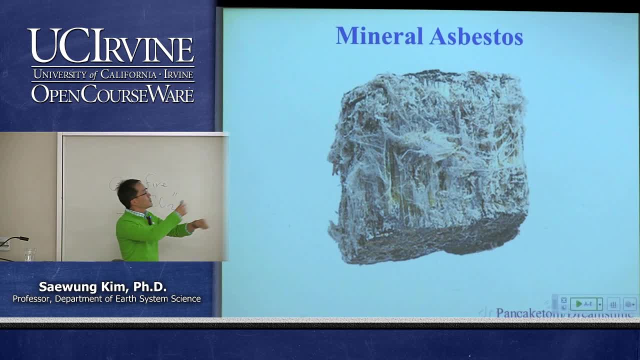 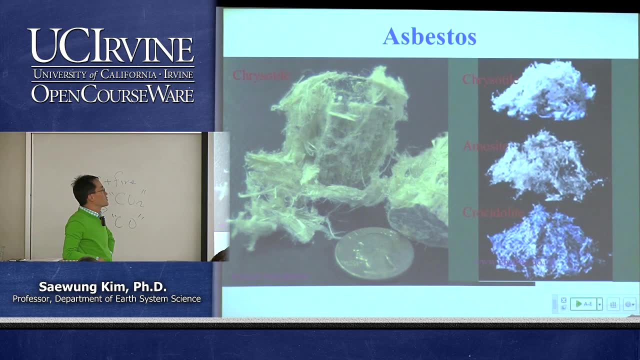 okay, And then asbestos. So this is naturally occurring mineral, So it has been used a lot in terms of insulation material. So this is how asbestos naturally occurred. So this is your quarter, so the size of this then you can. you should be able to see that. 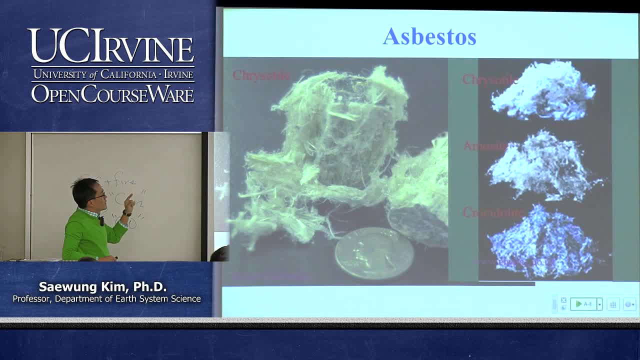 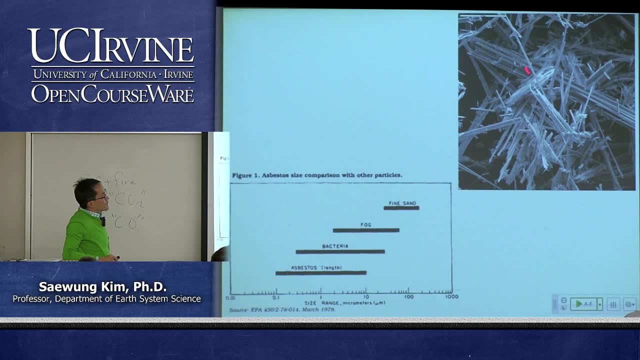 there's kind of a needle shape kind of thing. it's kind of a. that's the shape of this mineral. So you can see that Okay. So if you take a look at this thing under microscope, that is obviously it's composed. 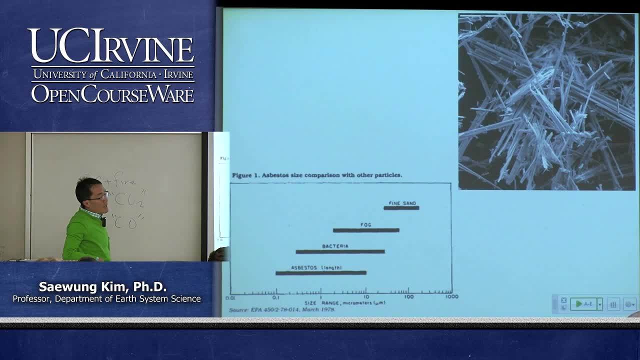 by really really small needle shape kind of thing, And once this thing gets airborne the size of this, each needle is sitting somewhere between .1 to 10 micrometer. okay, So why size is important? Because I think we 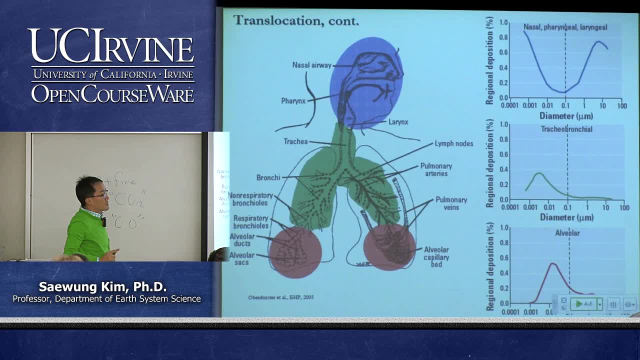 When we When over this thing several times, basically size matters in terms of how much, how long it can penetrate into our breathing system. So, basically, most of the really really small particle, really really large particle, particle size higher than 10 micrometer can easily filter out nasal airway. 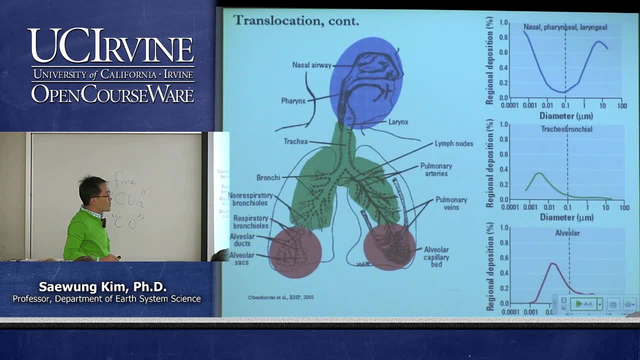 But the particle somewhere in between .1 micrometer to about 2.5 micrometer can easily filter out nasal airway. Okay, So the maison is then the last step where you can create a visible resin fortress like the one you will see. okay. 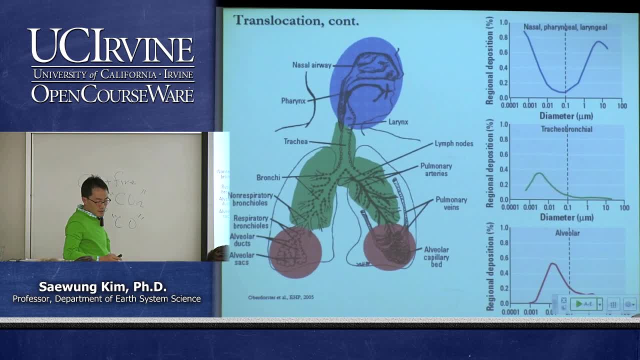 Now let's jump back into that, Okay, So take out our chinaterift When you put your chinateft in there and actually focus on this thing and you look from up here and you're looking what The shade? 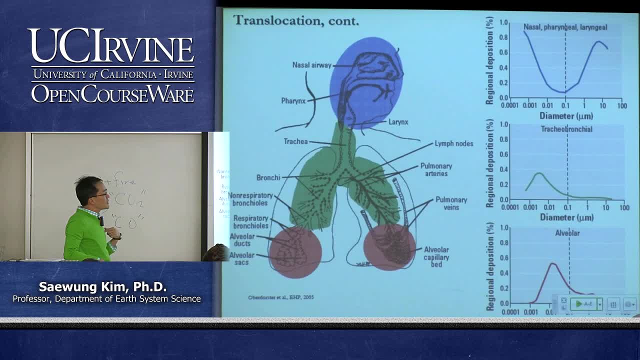 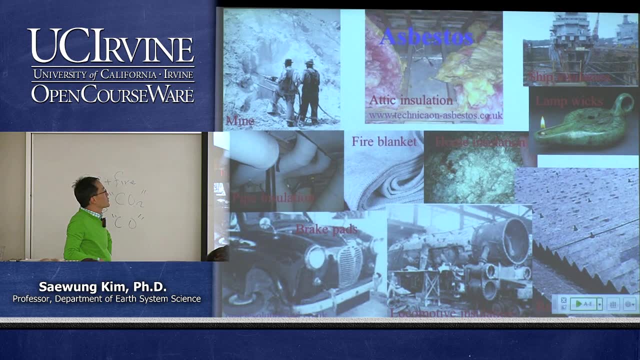 The shade. Let's go in and pull this thing. okay, Yep, Cut. Okay, I got it exactly All right. so Now you can guys see it. Okay For this, you can actually inflamm this one thing and then you do theничel. 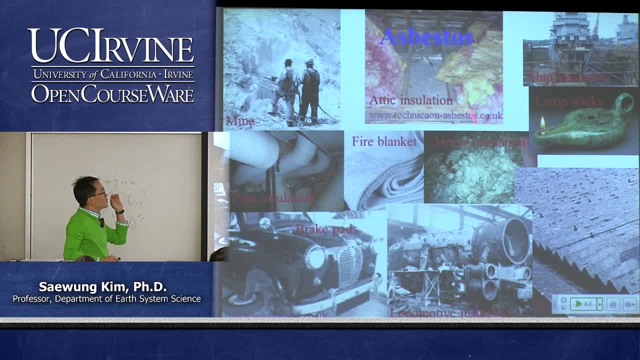 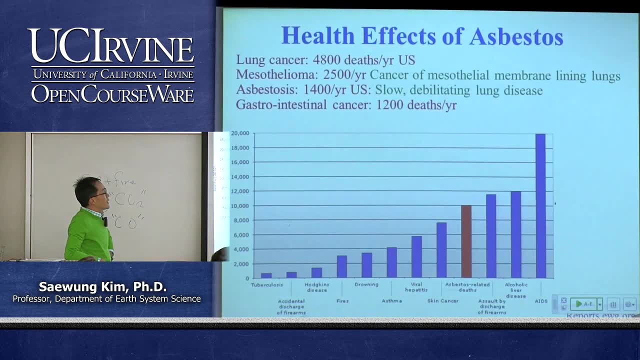 with it, All right. So they use this kind of Avastos and they process Avastos and then use it as an insulation And then this is consequences. At first time we didn't know Avastos actually can be bad for the health, but ended up that. 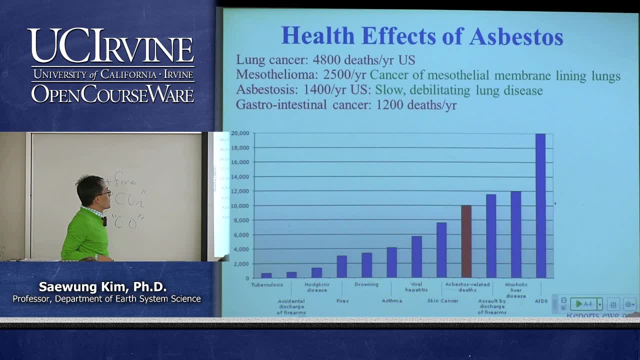 I think this is 2002 number of deaths in the US. The number one reason for the death in 2002 was AIDS, and then alcoholic liver disease- That's pretty striking- And then firearm discharge, things like that, And then after that was Avastos related disease, which is about 11,000 casualties. so right, 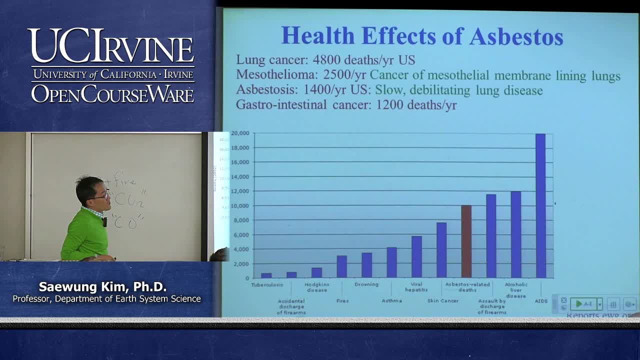 here. So the specific reason behind of it is lung cancer and then mesothelioma and then some other cancer. So So if you watch the late night TV then there's a lot of actually commercial about that. If you have mesothelioma, chorus kind of thing. 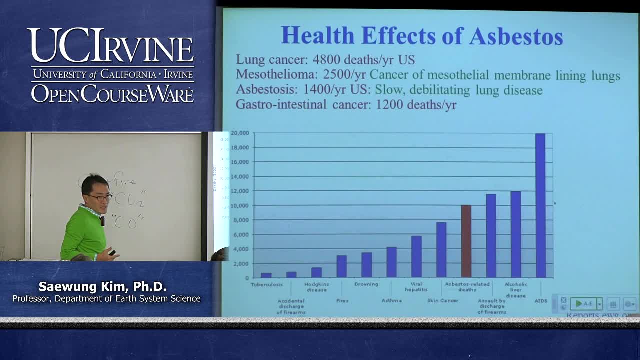 Have you guys watched that thing? Yeah, that's this thing. So that's kind of a lawyer try to hook you up and then make a big sue with the company who produced this thing. So that's mesothelioma is coming from this Avastos pollution and then, because it has 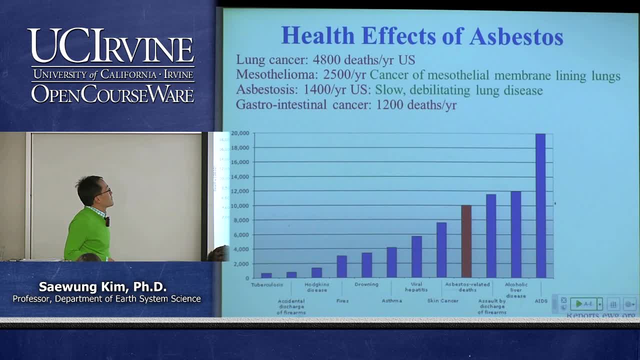 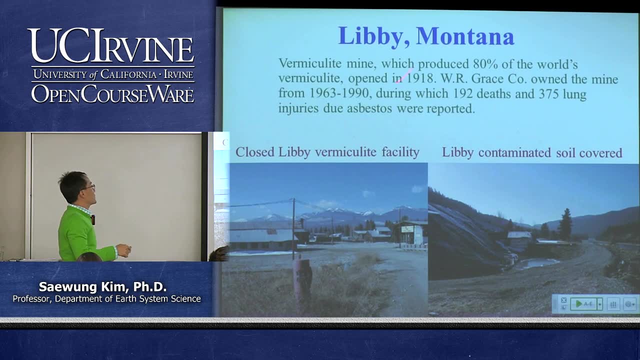 been used as insulation, So it is mostly from the indoor air pollution, right? So this is one kind of dramatic example that this is. have you anybody heard about this town, Libby Montana? It's a really, really small town. it's like 2,000 people total population. 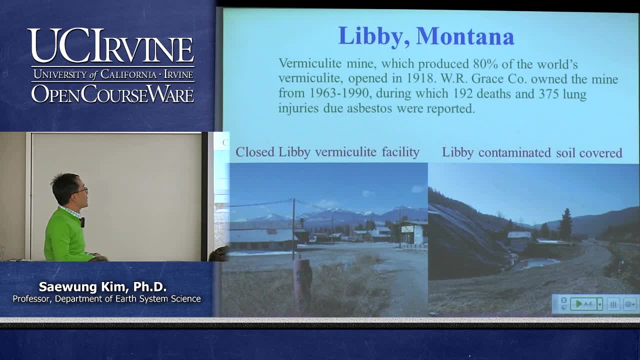 But this town obviously has a lot of this mineral, this vermiculite mine, So that's another part kind of mineral that has been used as insulation And that happened to have it's kind of mixture between this vermiculite and then Avastos. 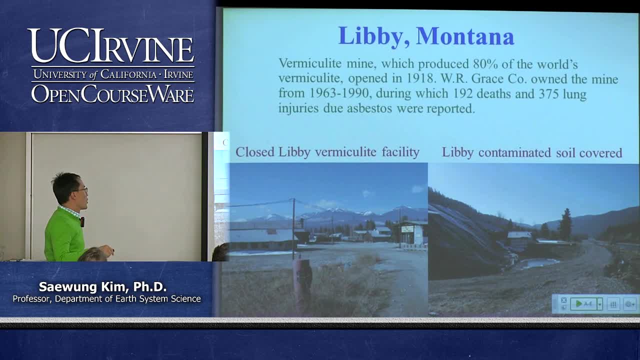 So there's a lot of production was going on, So one time it was 80% of world production was from this town, And then it happened to be this: it was a mixture between Avastos and then this vermiculite mineral. 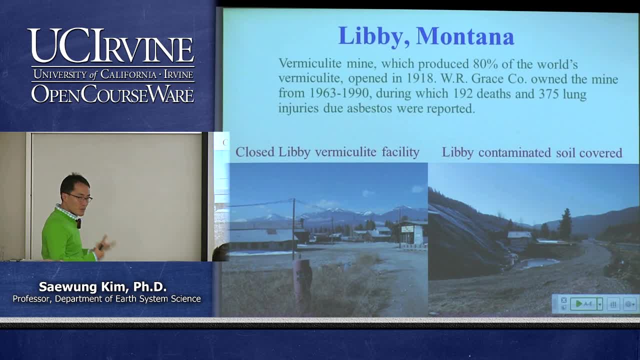 And then, as you can see, it is relatively small town, And then- this is obvious- It's big money, And then most people who are living in this town are actually all working on that- mine And then about I told you that the overall population is about 2,000. 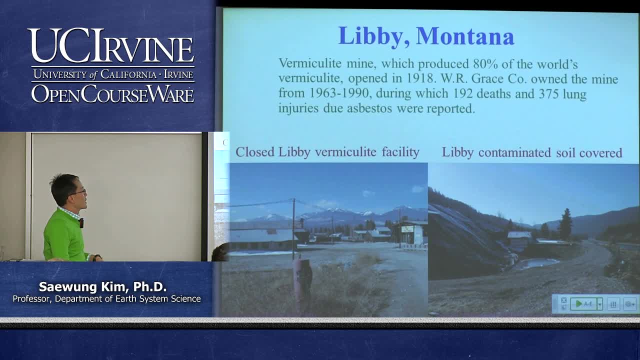 And then number of death: about 25 years time frame has been about 192 deaths. That's a very small town, so this is a lot of casualty. And then about 400 lung injury was reported in this town. So that's so. basically, these statistics indicate that how bad it is. 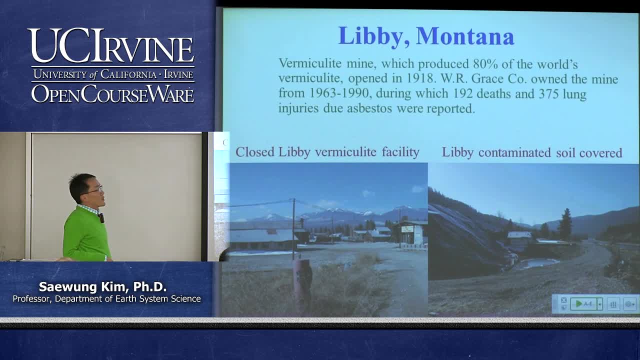 That Avastos pollution. So again it's practical kind of information. So if you plan to buy or rent a house- I think built before 1970, then you got to check that out. what's the insulation material? So if it is Avastos you got to do something. 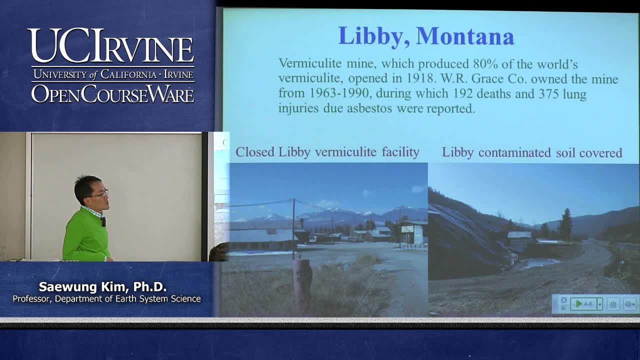 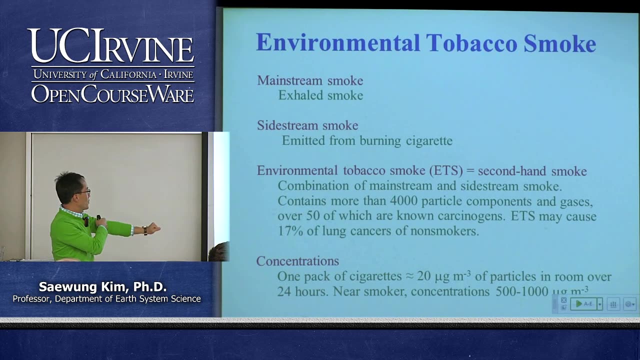 But I think most of states actually enforce to replace all those insulation material if it is Avastos to safer material. So Anyway, you got to check that out. And then the other important thing is tobacco smoke. So I hope you are not smoker in this class. 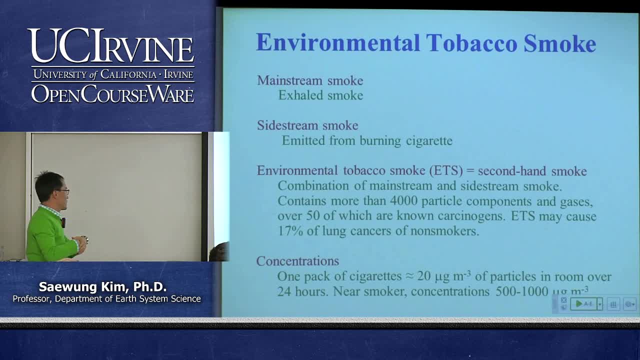 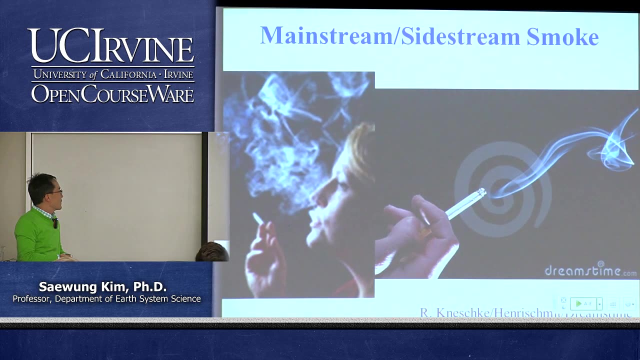 That's for your health. And then we are smoke-free campus, whatever thing is enforced, I think this year. So if you haven't quit your smoking, I hope I can change your mind from this couple of slides. So this is a figure. 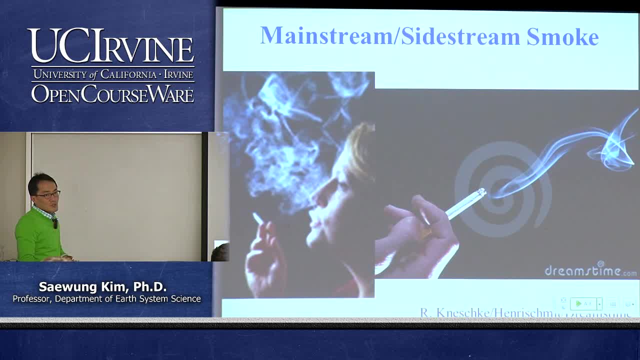 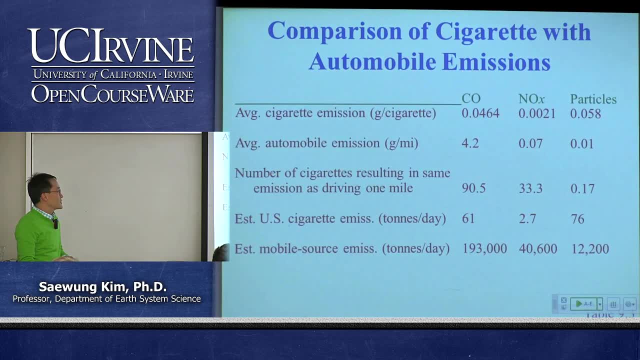 That obviously you can see this smoke, which means that that's gas and particle, right? So what kind of gas and particle? Interestingly that also this cigarette smoke contains a lot of particle, and then this carbon monoxide and NOx, and then all other stuff. 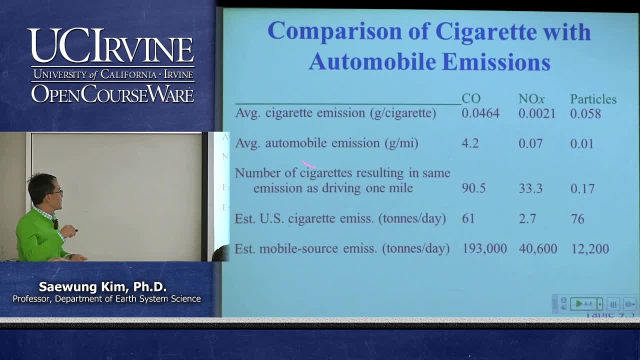 Then this is very interesting table that compare that average automobile emission gram per mile. So basically this is the emission of CO, NOA and NO2 and particles every car running one mile. So this is total number of CO, NOx and particle from the tailpipe if you run the vehicle about. 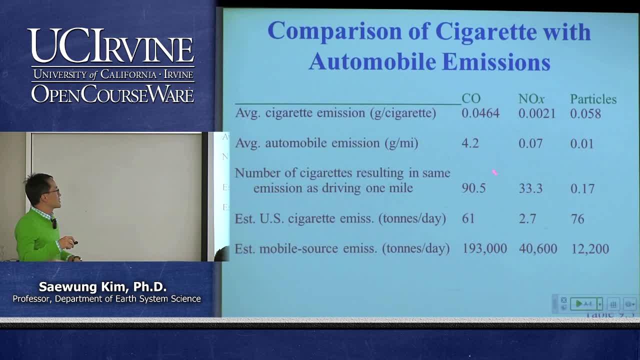 one mile of distance. So obviously CO and NOx is much high in terms of car driving. But if you compare this particle Then Actually This one cigarette actually generate more particles than the car tailpipe running one mile. So basically just good analogy is that basically you are just inhaling this automobile tailpipe. 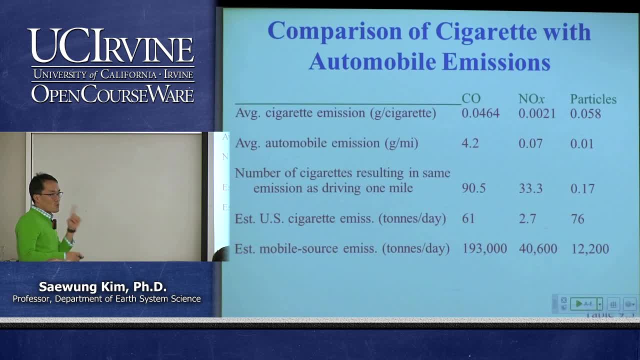 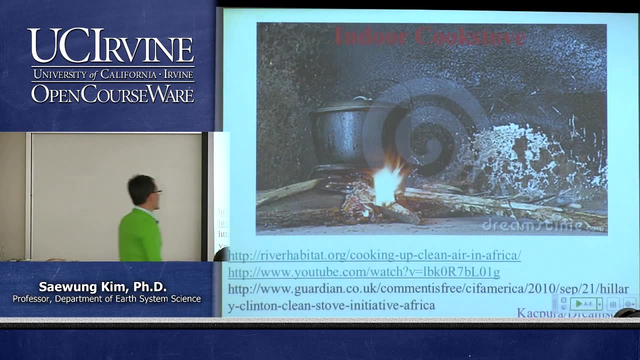 for one mile of the running when you just smoke one cigarette. Okay, That's that bad. So quit smoking. So that's the message right here. So another important source of the indoor air pollution is indoor cook stove, which looks like just like this: 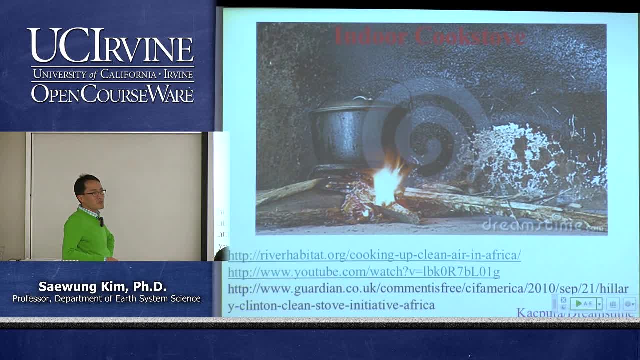 So in developed world like US this is not really problem. Not many people actually using this kind of the cooking system, You know, unless you're just going out to campground and then you know having some coffee and cook your meal, things like that. 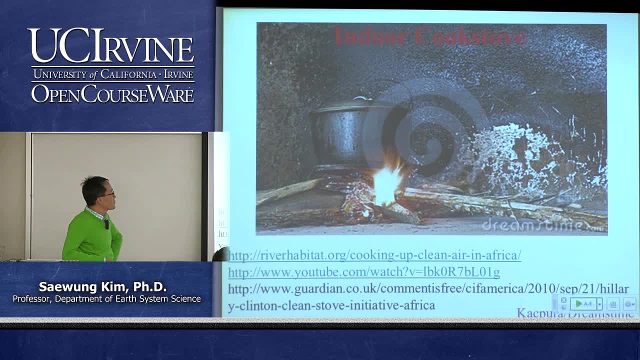 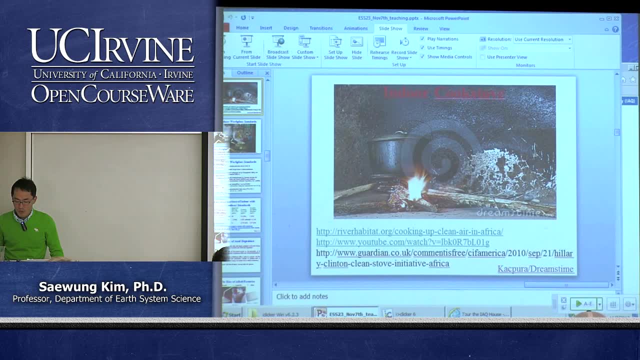 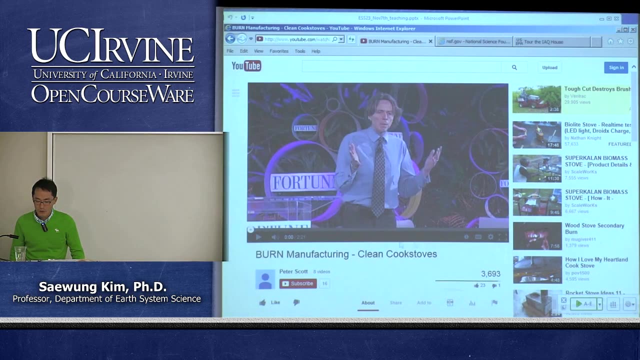 You use this thing, But not many people are actually using this kind of cooking method in developed world. But that's not the case other part of the world. So let's watch couple of the video related with this problem. So let's go into the front and watch this thing. 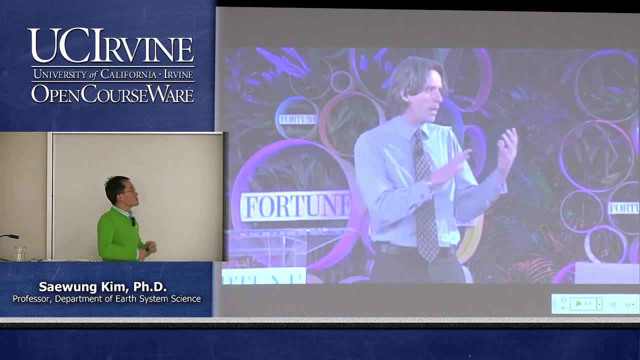 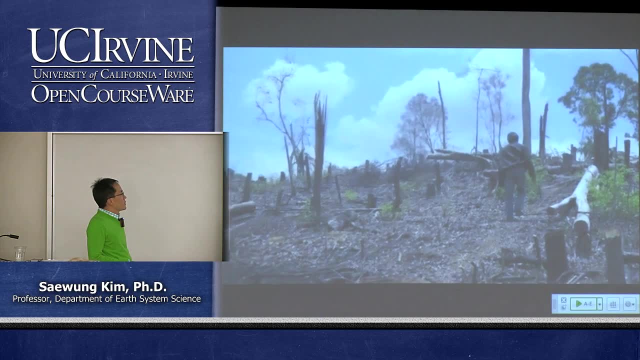 My name is Peter Scott. I'm the founder of Burn Manufacturing. 20 years ago I went to Africa and when I saw deforestation in Africa and Congo I got down on my knees and wept And I said: I'm going to devote my life to save the forests of Africa, in the developing. 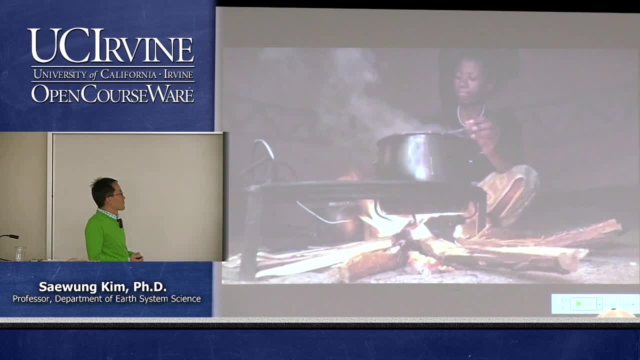 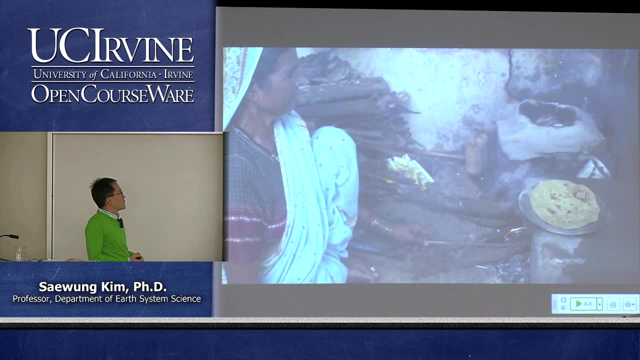 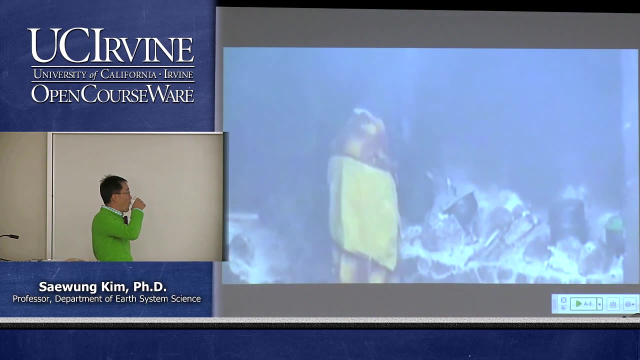 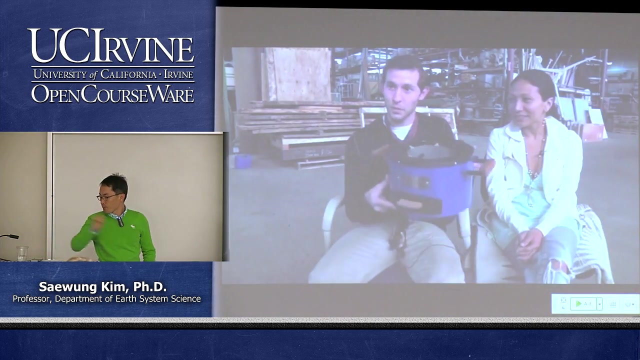 world. Many people are unaware that each year, 2 million people, mostly women and children, die from exposure to smoke from inefficient open fires. My goal was to save Africa. My goal was to create a stove army of engineers, researchers and designers. 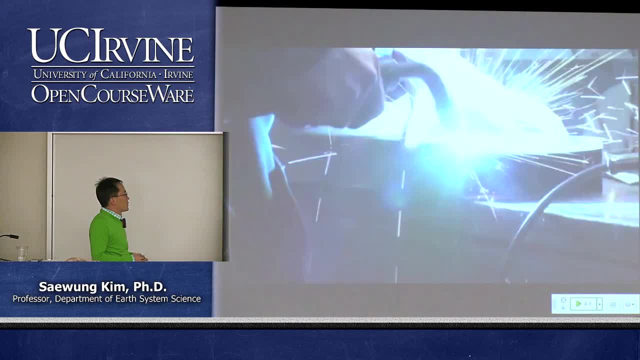 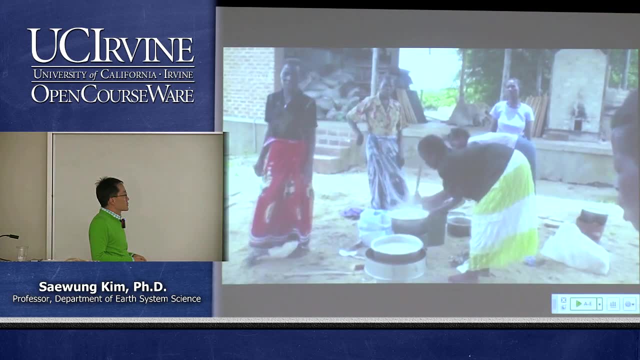 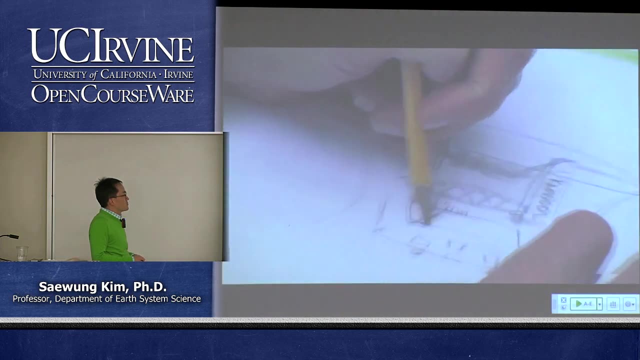 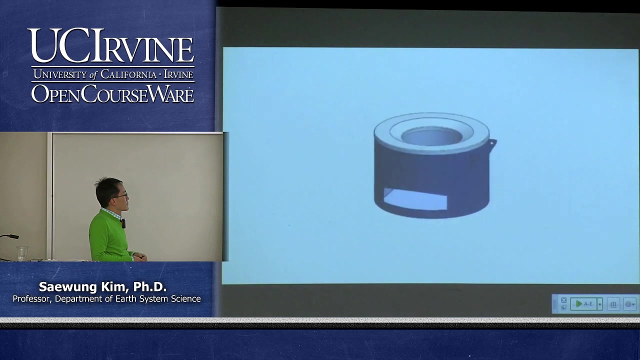 Our team works with local women to design the most fuel efficient stoves in the world. We have spent thousands of hours designing, iterating testing to create this stove: the tank. This stove uses 50% less energy than the existing improved stove in East Africa. 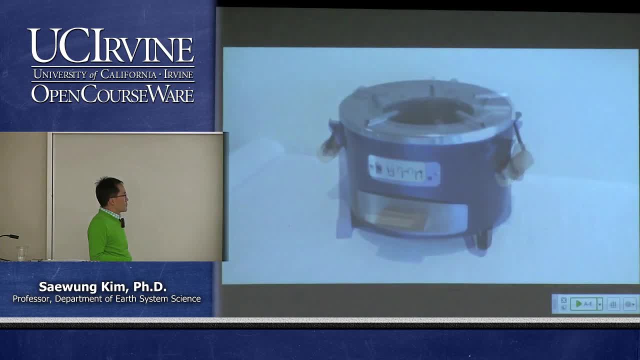 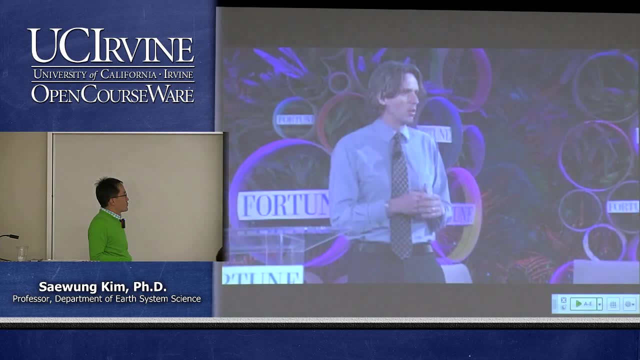 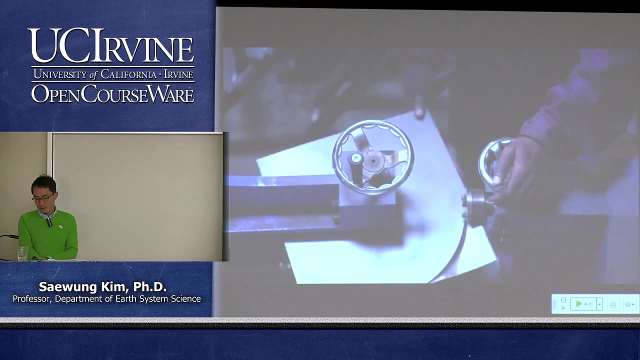 I mean really, there's an incredible opportunity. So who wants to quit their fracking job and join me? Yes, hands up Daniel's with me. By manufacturing 3 million cook stoves in Africa, we've saved the lives of thousands of people in Africa. 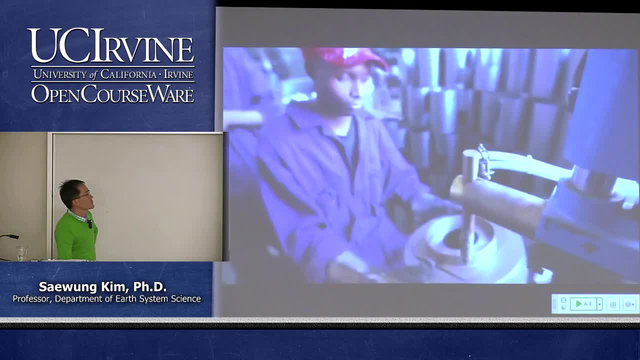 We've saved lives. We've saved the lives of thousands of women. We saved the lives of thousands of men and women. We've saved the lives of thousands of women. We've saved the lives of thousands of men and women. We've saved the lives of thousands of women. 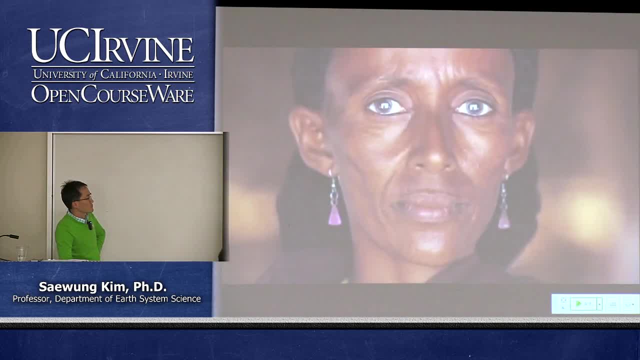 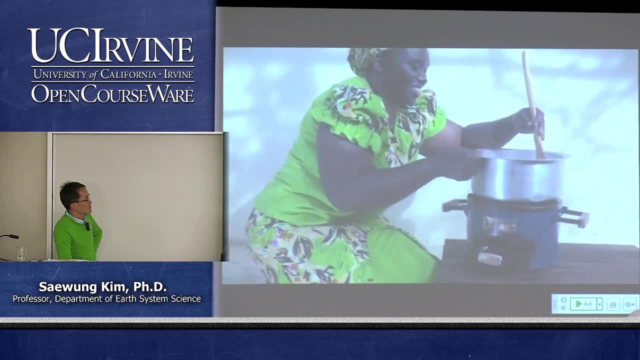 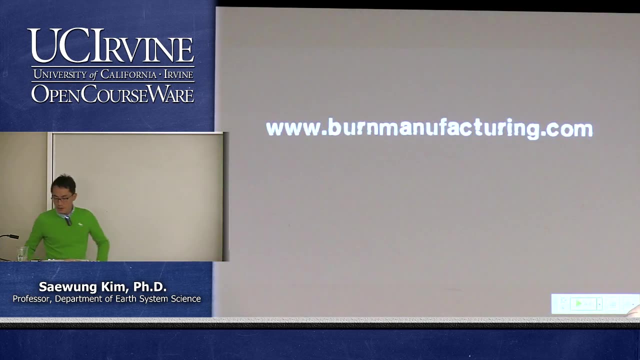 Africa. we're going to save thousands of lives, more than 100 million trees, we're going to create local viable jobs and we're going to reduce indoor air pollution for millions of women. it's an incredible opportunity. we hope you join us. so obviously you can see that's the problem in some part of the world, especially uh in. 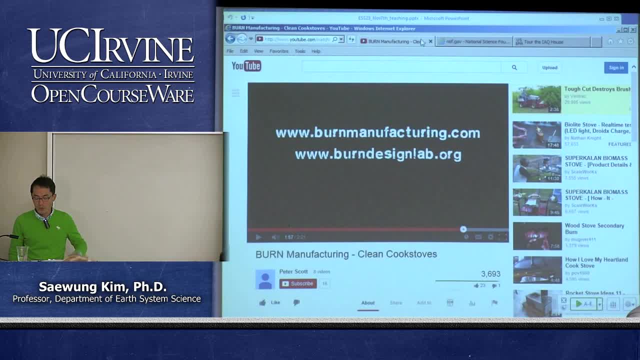 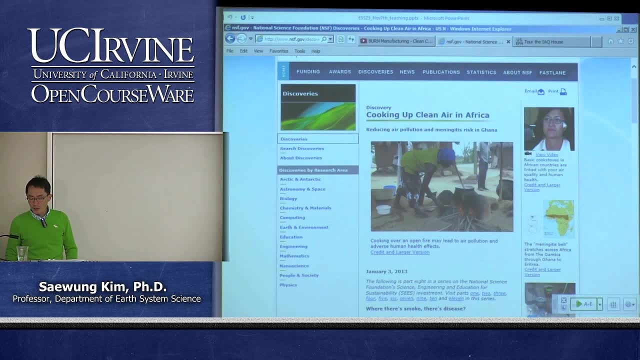 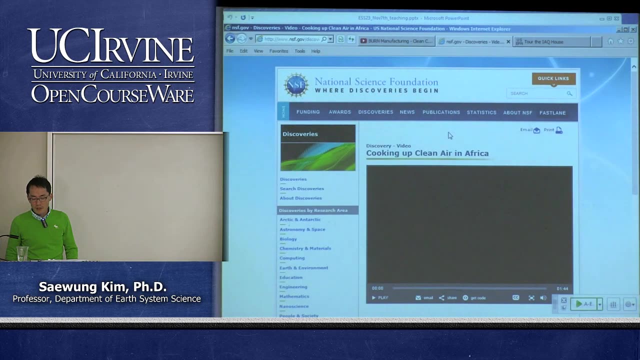 african country and then, um, actually this is kind of a grassroot movement that just initiated by a single person and then actually government is doing its research too. so national science foundation actually fund this kind of research. let's take a look at this: what the scientists should say about this thing. 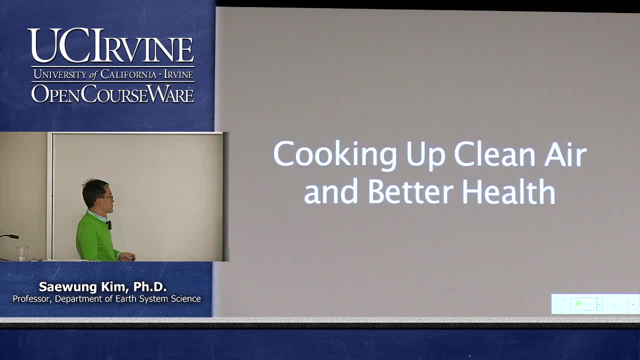 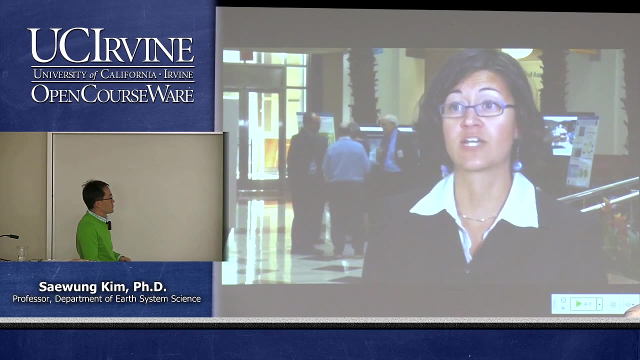 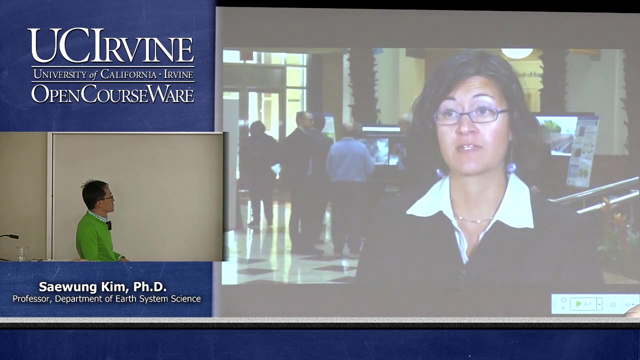 so the problem that our study is trying to address is that people in a lot of the building world actually don't use crystals. they cook over open fires, and that's about 3 billion people worldwide who do that. this practice has implications for greenhouse gas emissions. the fires don't burn very efficiently, and so they emit black carbon, which is a big 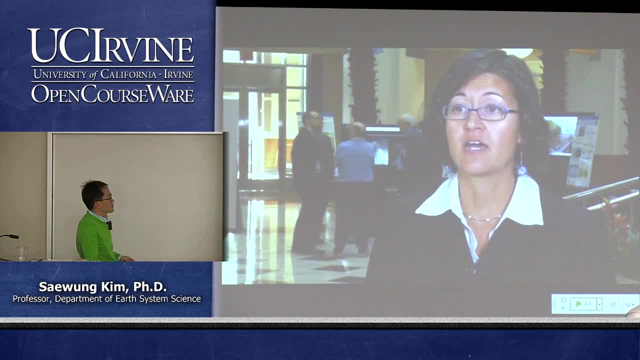 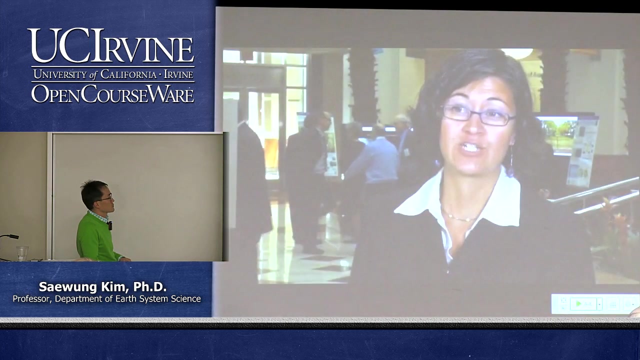 greenhouse gas contributor and they also have implications for people's health. so respiratory disease kills about two million people a year. so that's what people currently do throughout this region: they burn wood, agricultural waste, and so that's kind of the current. so what we would like to do is look at how feasible it would be to get people to. 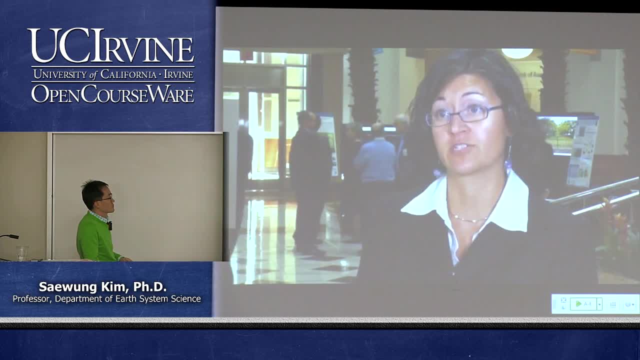 from cooking over open fires to cooking over cleaner, burning cookstones, and so we are piloting the use of some stones, and my role in the project is looking at the behavioral side of. do people actually want to use these stones? what are the cooking needs and do the cookstones 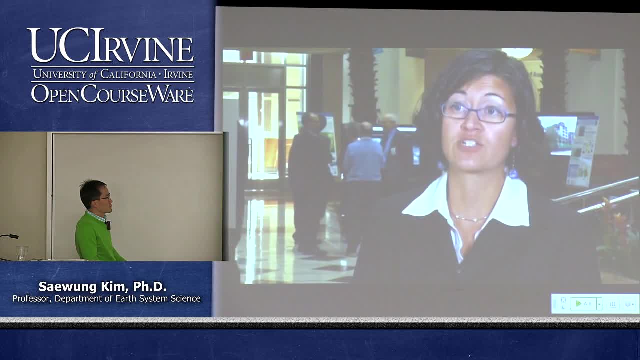 that we can introduce in this area? do they have the potential to? to meet people's cooking needs and let people cook in a cleaner way, but also in a way that continues to. so i'm going to give you a little bit more about the use of these stones. 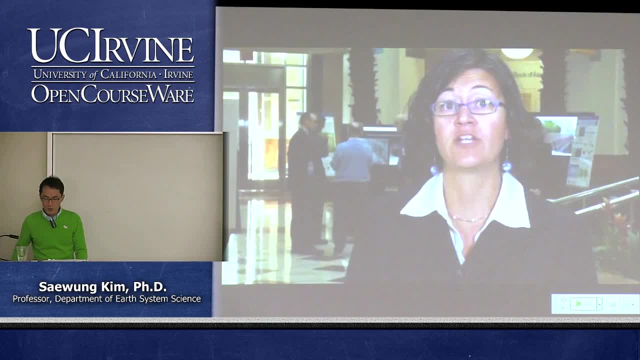 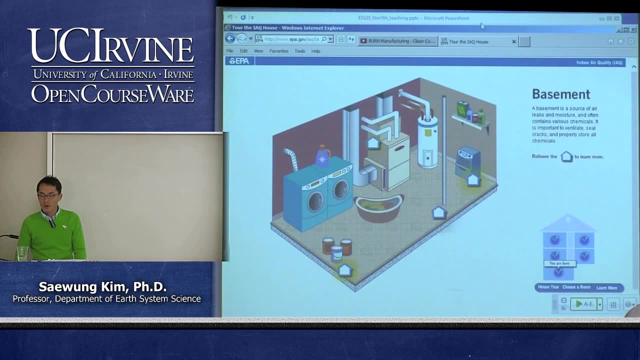 so she was talking about that wood burning in the house and then again it's kind of the same process that what caused that london type smog. then those kind of burning will produce co and so2 and then particles and then it's in the house environment. it's kind of isolated environment. 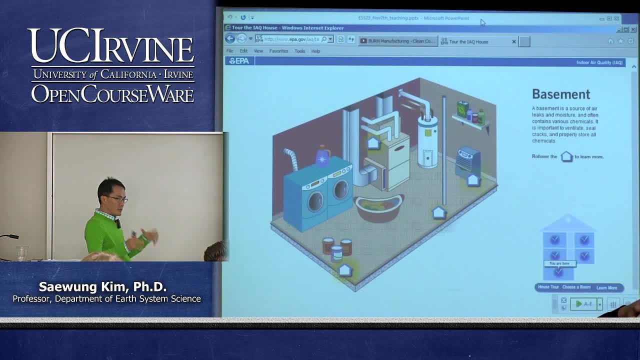 there's no ventilation going on, especially for the small kitchen, can emit a lot of that. then that kind kind of environment- actually those immediate CO, SO2, and the particle can accumulate a lot- can get the very high concentration in there right. 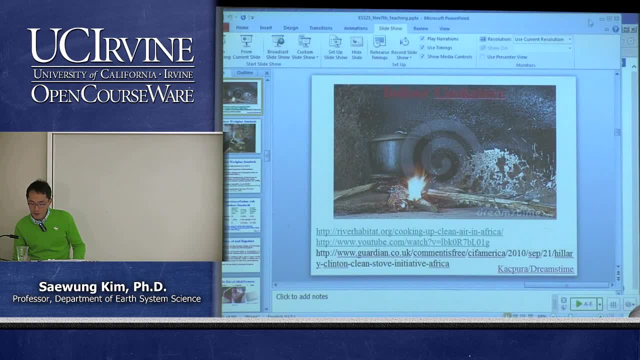 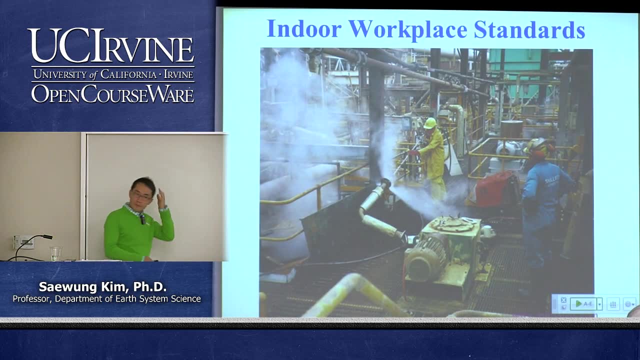 So that was this part. Okay, let's move ahead. So once you have a job and then working on the industry, things like that, and then obviously we discussed about that ozone regulation level, which is 75 ppb for eight hour average. 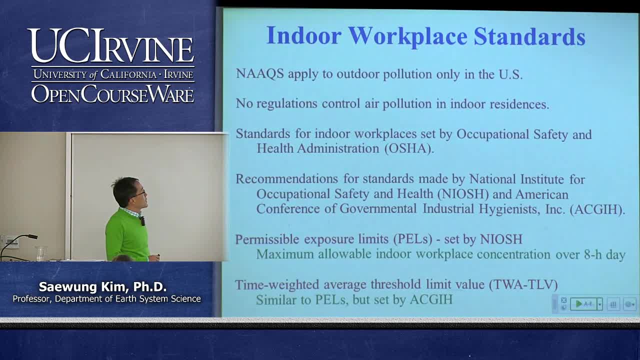 that is enforced by EPA. But indoor workplace standard is not regulated by EPA: is regulated by OSHA standards for Occupational Safety and Health Administration. So if you have any problem in the air quality in your job, things like that, then you're gonna take a look at the OSHA homepage. 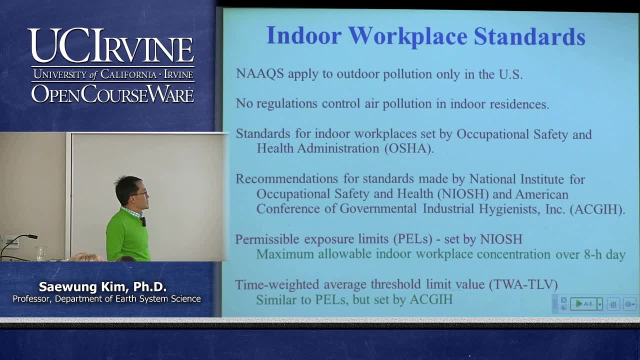 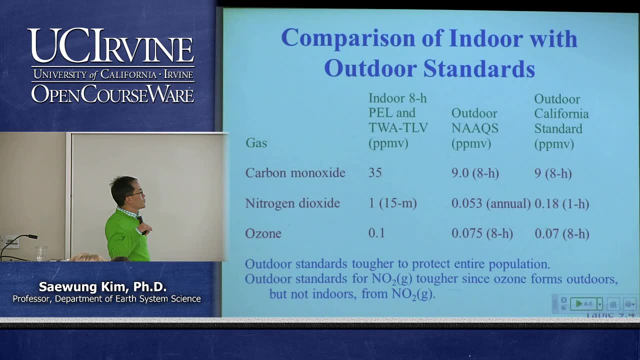 other than EPA homepage. So that's the main message in this slides. So, as you can see here. so let's just take a look at this NO2 level. So EPA, so basically that's EPA, and there's California, and then this is EPA standard. 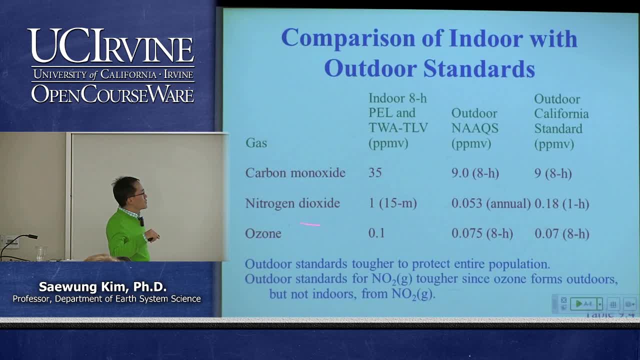 and then this is OSHA standard. So for the eight hour OSHA standard is one ppm and then EPA standard is 83 ppb, .83 ppm. This is annual and then one hour is 18 ppm. So obviously NO2 concentration outside regulation level. 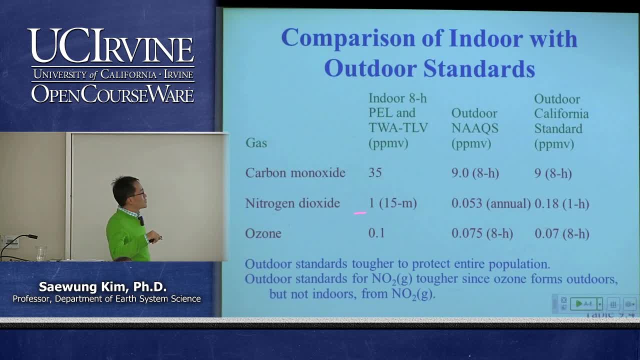 is much tougher than indoor level because there's no possibility NO2 actually produce ozone indoor environment because there's no sunlight. So that's why the regulation level is a little higher, actually much higher than outside regulation level. So that's the kind of differences. 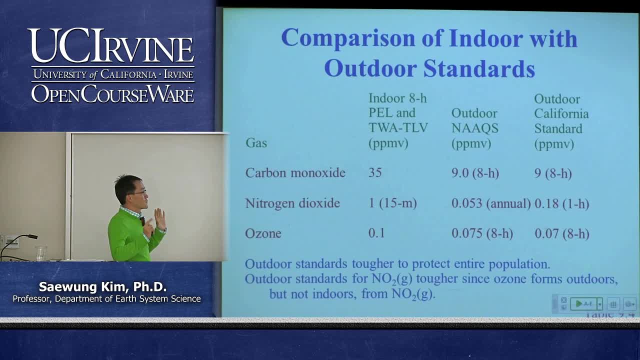 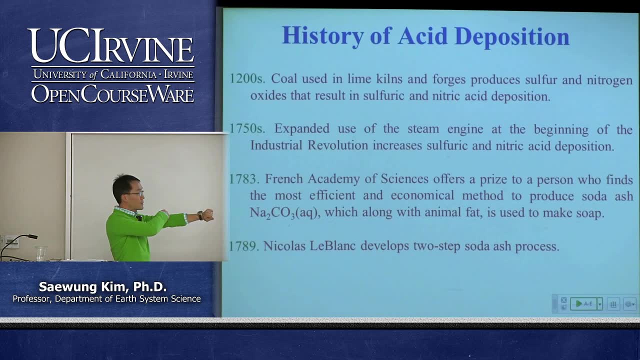 Different regulation apply to different environment, so obviously different administration regulate the different kind of thing Here. so let's move to the some science stuff: ethylene. So you guys probably heard a lot about the ethylene, so that's here what they call it: ethylene. 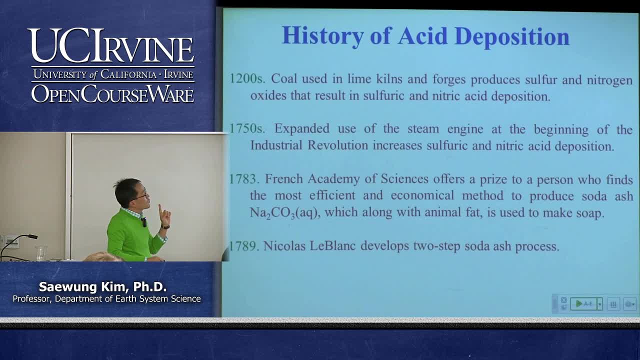 We call it acid deposition. So rain is just one event. The reason we call it deposition is that actually something like fog, things like that can be very acidic and then those kinds of fog can also affect the ground ecosystem Also, for example, snow. you know snow can be coming down. 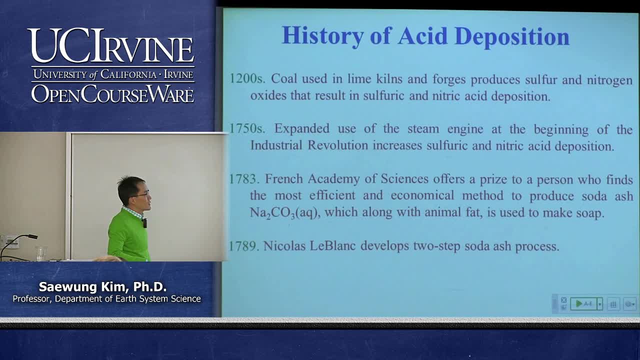 if it is acidic and then it can be melted and then can destroy the trees, things like that. So we want to include, kind of we want comprehensive term- that anything coming from the sky that get acidified by the human pollution. 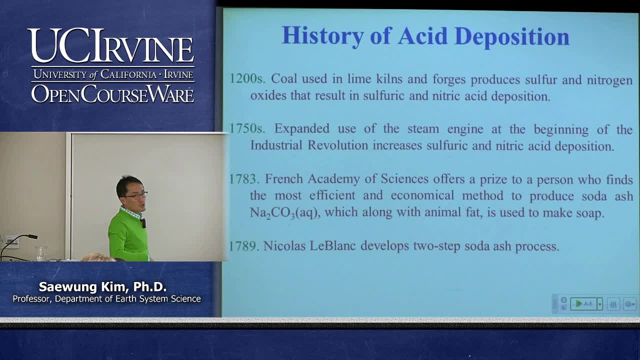 So we call this thing as acid deposition instead of acid rain, So this is more kind of comprehensive term. okay, So we talked about coal, started used about 1200 for making lime cleans, which is kind of building, which is a material for the building material, and then that emits sulfur, which 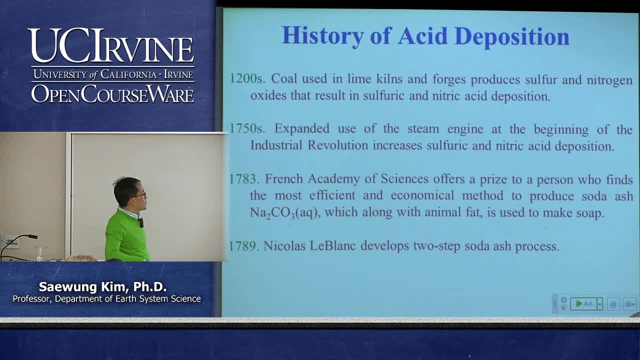 is SO2, and then nitrogen oxide, which is NO2 to the atmosphere, right, And then also this SO2 eventually becomes the sulfur dioxide. is this sulfur dioxide? and it becomes sulfuric acid and then people start to realize this acid deposition from. 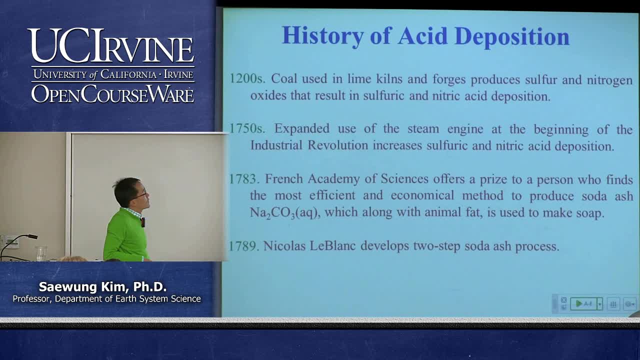 sulfuric acid and nitric acid from NO2 actually make up for it. So this is a real problem on the ground. And then the real this acid deposition problem become a real problem in about the late 1700s, when a chemist developed the method to make the soda ash. 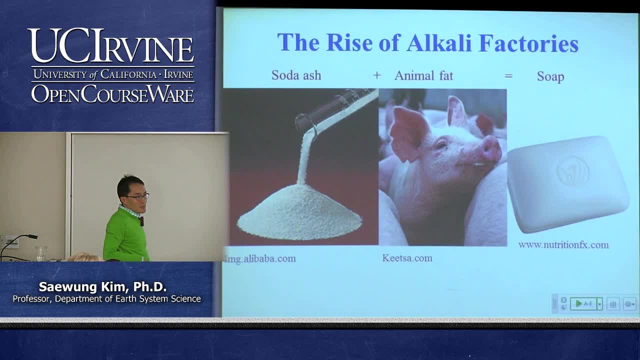 So what's the soda ash for? To make a soap? So, basically, if you just dissect the soap, that nice smelly soap that you use every day, maybe every hour, If you worry about the infectious disease, whatever thing, actually it's kind of if. 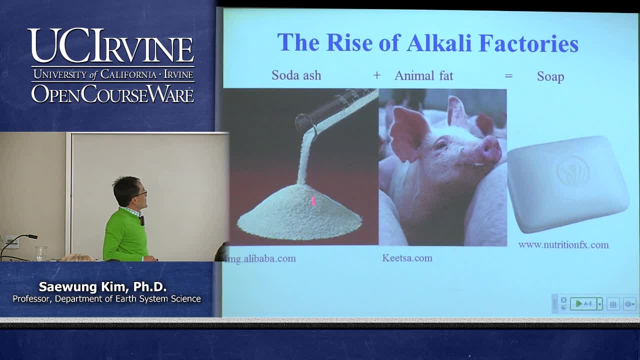 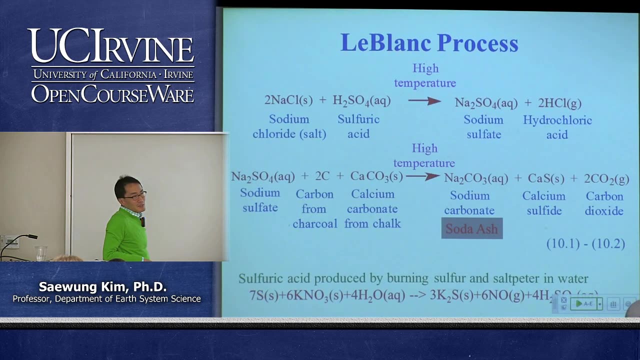 you just dissect the components, then you need soda ash, and then you need animal fat, And then this photo basically shows you where that animal fat coming from, right And then how we can make the soda ash to make the soap, this chemical processes. 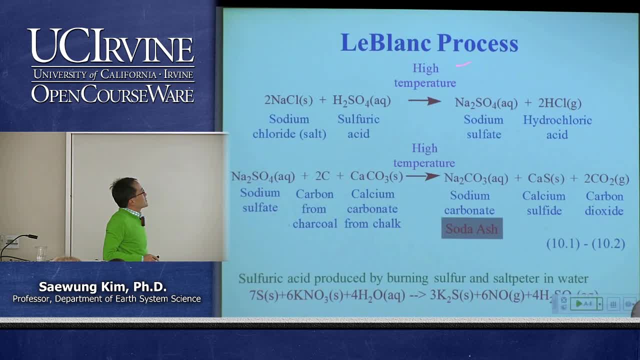 So basically, in high temperature. so this is a chemical engineer named Lou Blanc, And then he developed this process to make soda ash. So if you're afraid of this, all those chemicals, what you need to remember is use high temperature. So some bonding process is going on, right? 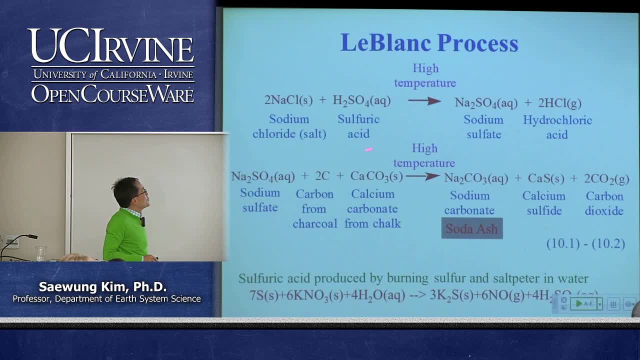 This high process temperature is what that means: That it use sulfuric acid out here to generate the soda ash and then it is making HCl, which is very strong acid. Okay, Okay, Probably you can remember that bar, I guess, I hope. 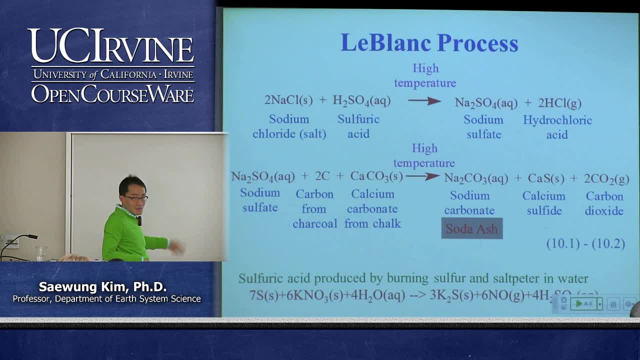 So it is bonding, probably cool out there. So it is. it's going to be generating a lot of CO, SO2, things like to the atmosphere. Then it is using sulfuric acid, which is very strong acid, And then it is also by product HCl gas phase. HCl is emitting to the atmosphere. 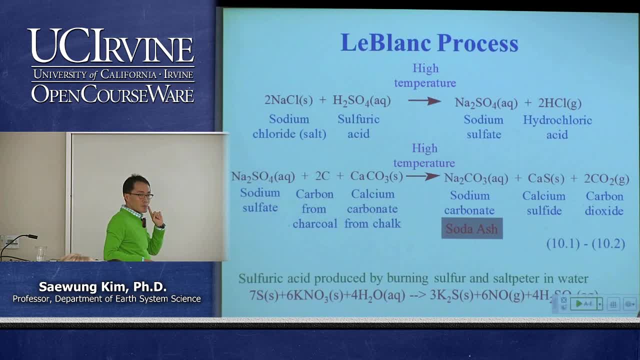 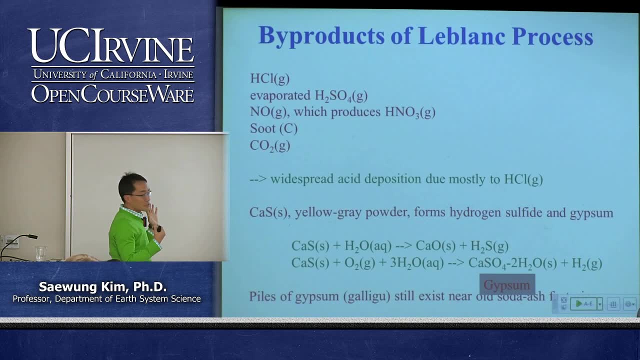 So these are source for acid Acid precipitation Because they are strong acid. Okay, So that's, this is summary. So if sulfuric acid and HCl, and then these are byproduct of the coal burning And then another coal, another byproduct, it was gypsum, which is mineral composed. 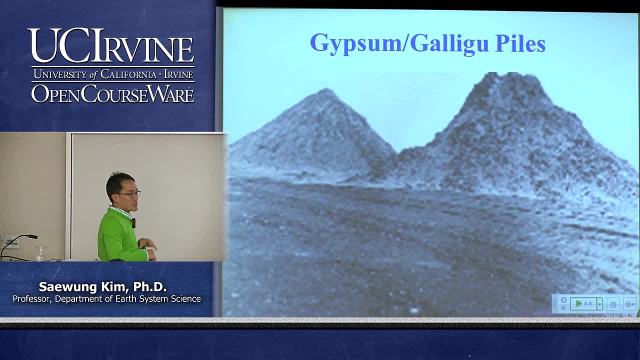 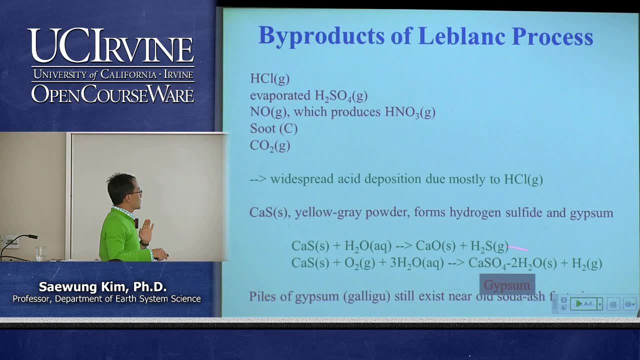 by this thing. So if you take a look at the old photos near that, this soda ash factory, you can see there this pile of gypsums everywhere from this chemical process. So this kind of this is kind of visual thing. This happened to be solid. 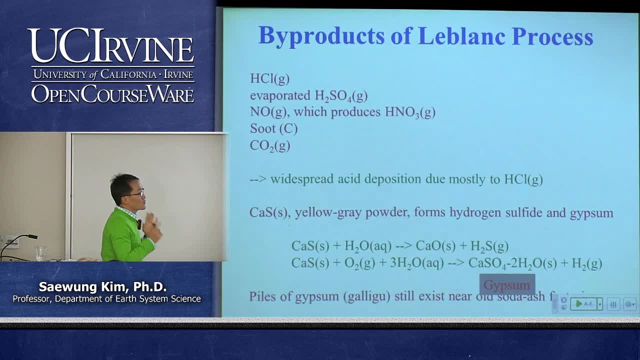 You can see the pile of gypsum, But what you should able to see from this process is that this is solid, so we can see it. But these gas phase pieces- although we cannot see these guys- HCl and sulfuric acid and 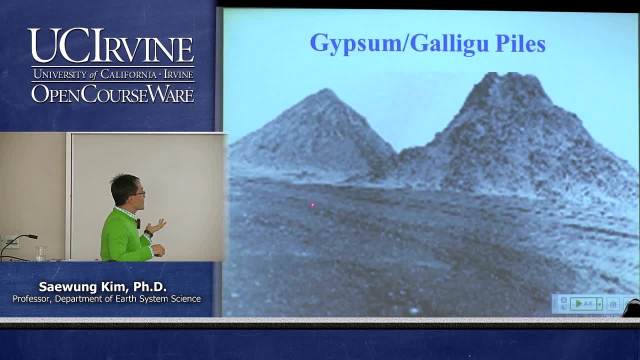 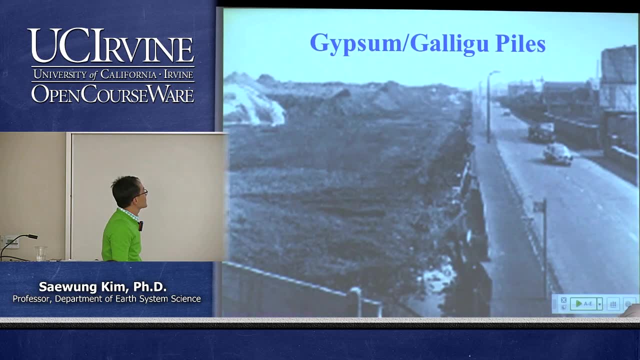 then NOx and then some particle- Actually, Although we cannot see it, those things actually sitting in the atmosphere and then making acid rain. Okay, So that's another pile of gypsum. So, again, this is good visual indication that there's a lot of HCl and sulfuric acid is. 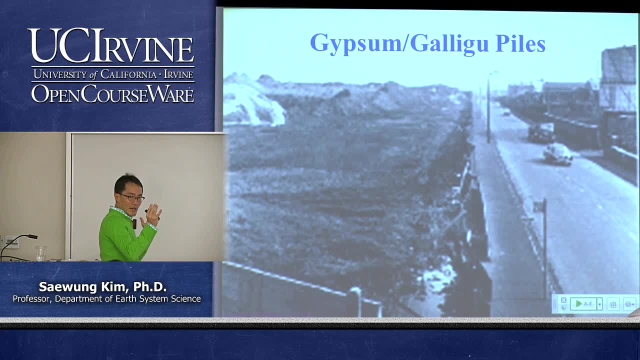 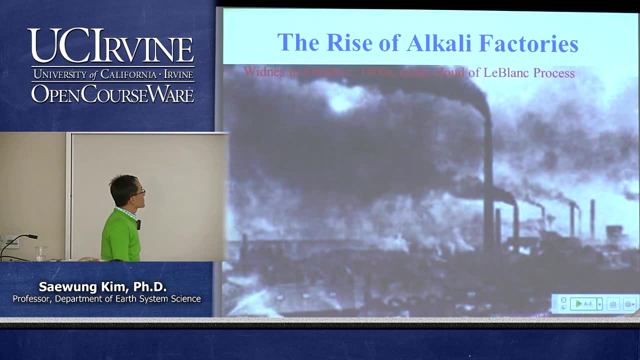 sitting in the atmosphere, Then if there's rain event, then those kind of acid is going to be dissolved into the rain. Then it's going to be will get affected by that acid rain. Okay, So that's the when a soda ash factory 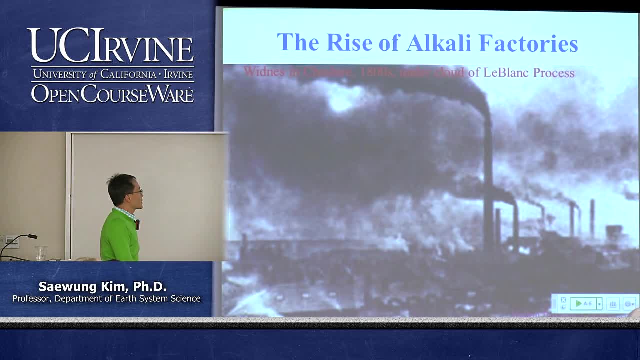 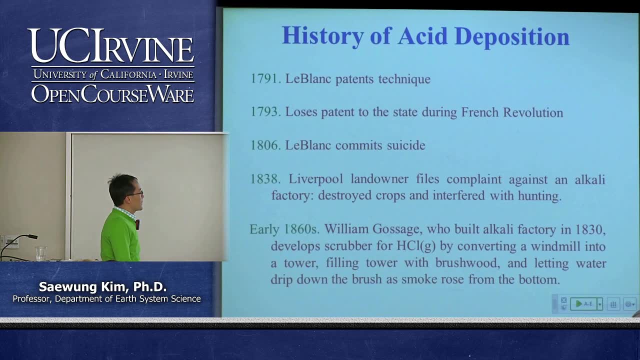 It's going on. there's a lot of processes going on right. So immediately after this Louvre Blanc process, kind of developed and patented, people start using a lot this process to make soap right. So once you start using soap, you cannot stop using soap right. 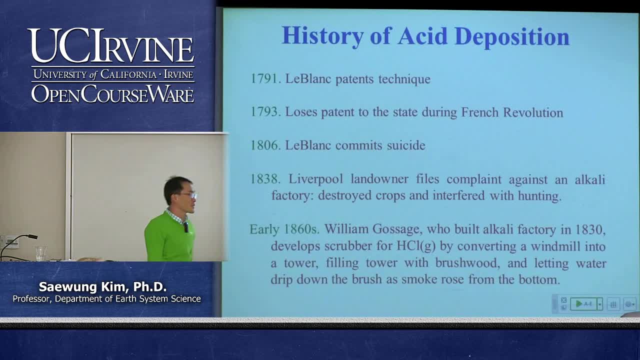 You gotta using soap because that kind of clean feeling you cannot never forget about it, right? So people just kept producing that soap all the time. So that's Okay. And immediately after all, 40 years after that process first patented- people realized 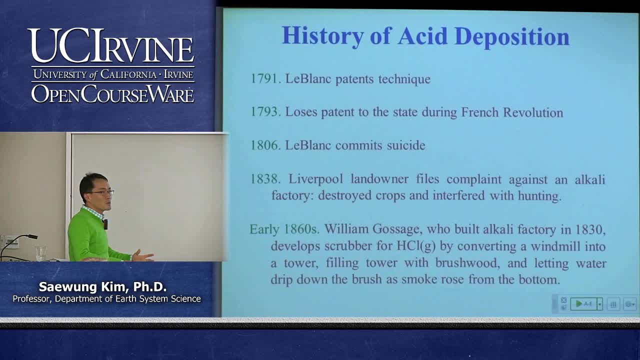 it actually destroyed crops and then interfered hunting. Probably hunting was really big deal back then. We are not really worried about hunting that much, but basically this indicate that it affect on our daily living. And then if you remember that definition of air pollution, basically if that human made 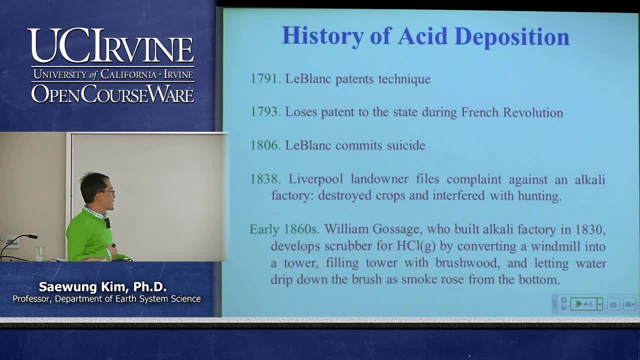 gas or aerosol. if that affects on our daily life- daily life- then that's, by definition, air pollution, right? So that was mainly HCL. So again, we cannot really go back to the life without soap once we start to use soap. 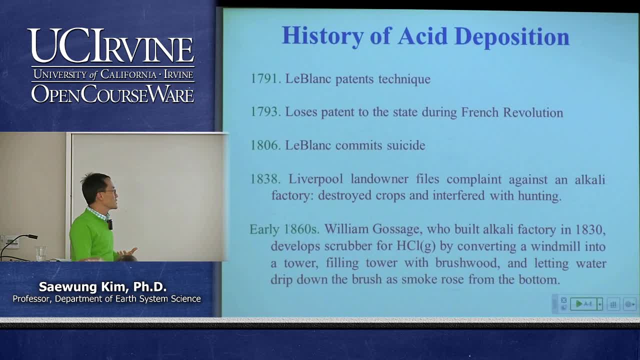 So what people are usually doing is that kind of developing technology can lead of the HCL. So about 1860, engineer William Gorsuch developed the HCL. Okay, Okay. And then the next thing is the scrubber that can remove HCL from the stack of the soda. 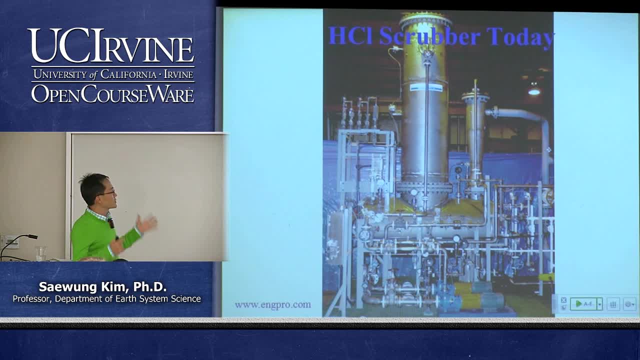 ash company. So this is modern day HCL scrubber, So this kind of gigantic thing. Then, when air is passing through this scrubber, so HCL can be removed from the exhaust, so that the air without HCL can be emitted to the outside, 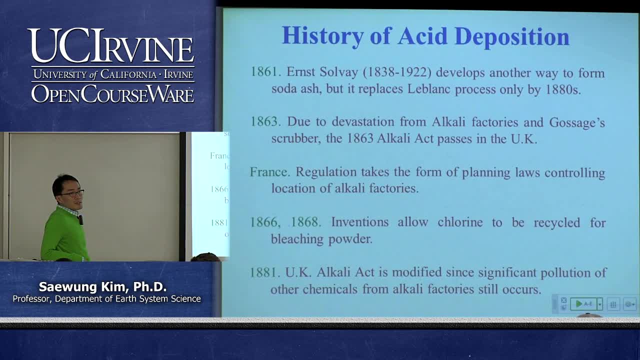 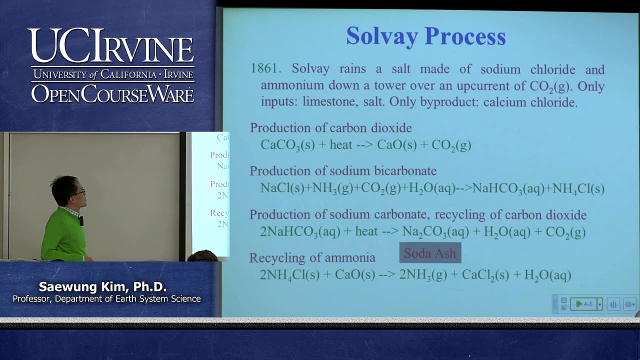 Okay, So even better solution is that kind of developing new chemical mechanism that doesn't produce any HCl, right? So that's, that was done by unsurvey. So survey process. so this is survey process using a total different material, CaCO3. 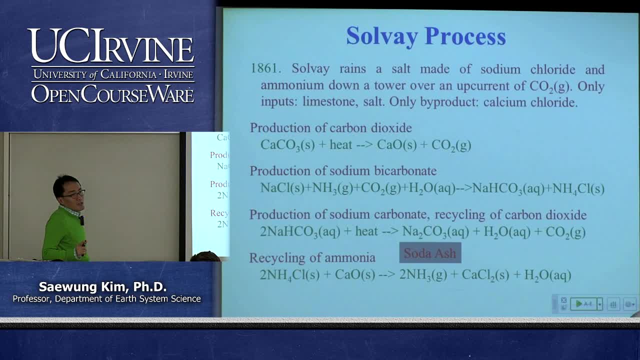 So if you take a look at these processes, you cannot find any acid in this process, right? You cannot find HCl, you cannot find H2SO4. So this process basically doesn't emit any strong acid to the atmosphere. So at least the problem of the acid precipitation from HCl solved by adopting this new chemical. 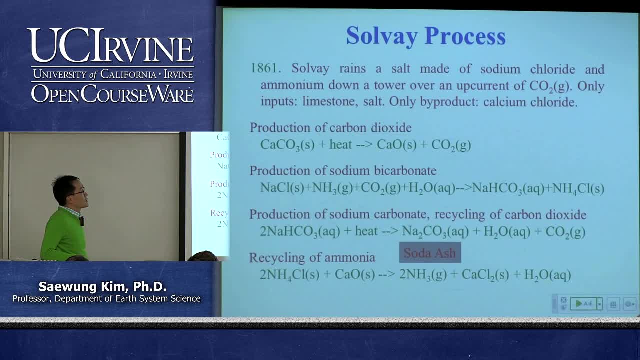 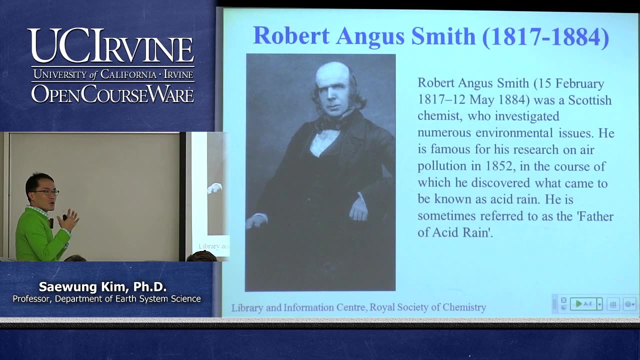 processes. But obviously we know that after this we solved this problem: HCl problem. still the acid rain, acid precipitation It's a problem. So we will discuss about that thing, about what the other chemical compound actually affects on the acid precipitation. 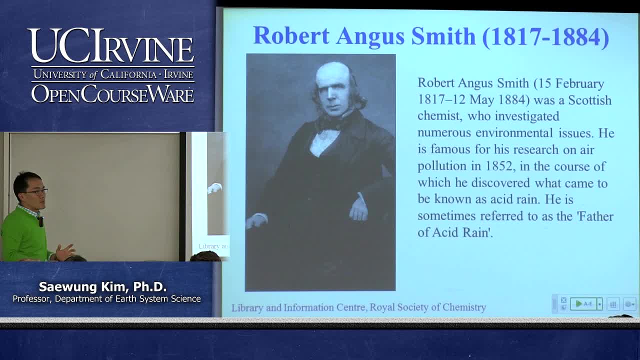 So this is a guy who looks like criminal. he's not really a nice looking guy, but he's father of acid rain, very environmental friendly kind of guy. he studied a lot about the acid rain, So it's for your knowledge. So I'll stop here. 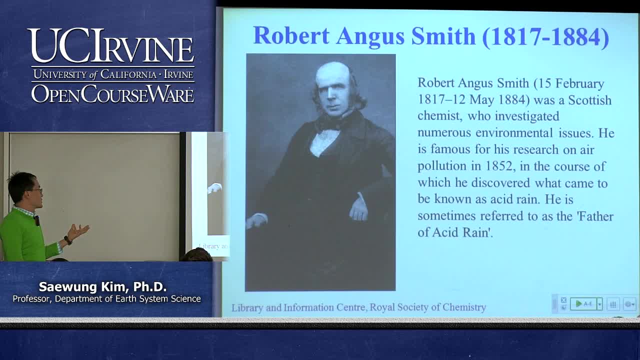 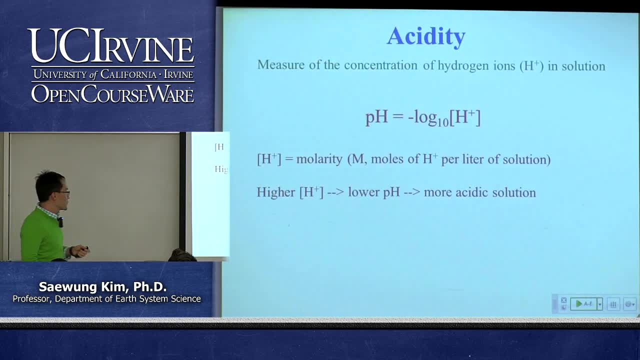 So I'll try to introduce this guy who addressed a lot of questions related with acid rain back in 1800, right, So to understand acid rain, we need to understand acidity, and then we really want. we scientists love to quantify everything. 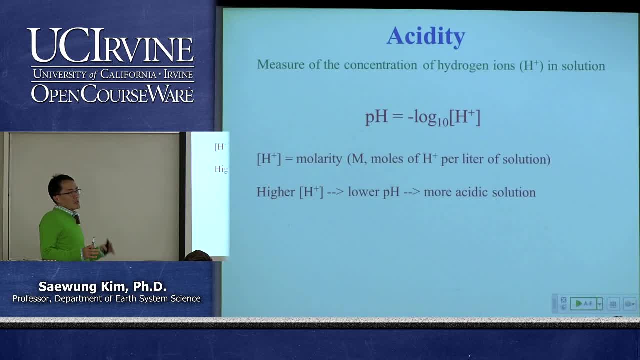 So we really need to know. we really hate the idea about the acidity is high or low. So high, if it is high, how high? And then if it is low, how low. That's why we love numbers, So I will introduce some numbers today. 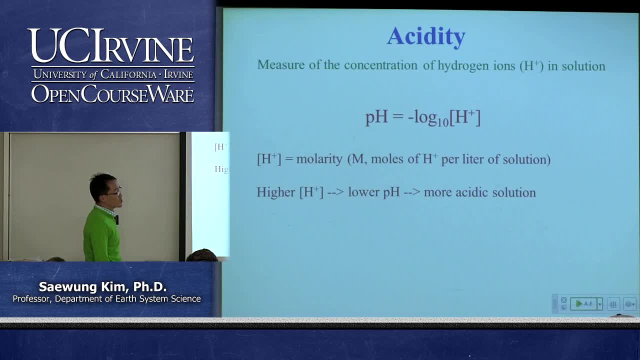 So basically we call it pH, So that's kind of a concentration of the H plus in the solution. So basically you can think that this parenthesis indicate that concentration. so this parenthesis H plus, H plus means that concentration of H plus in the water. all right. 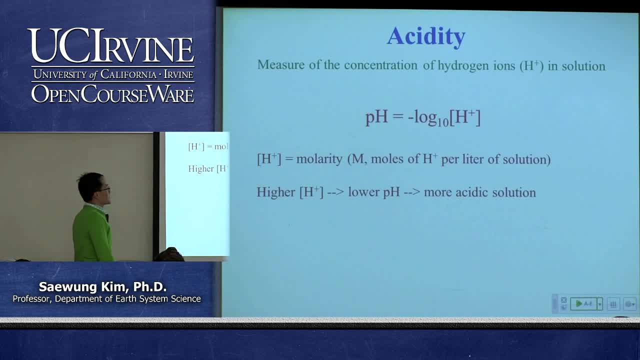 So why we are putting this real thing in front of H plus? Because to make our life, you know, easier, at least to me, but to make life, your life, more miserable, maybe in terms of to understand this log scale, But it is not really too difficult term, it's more like this: 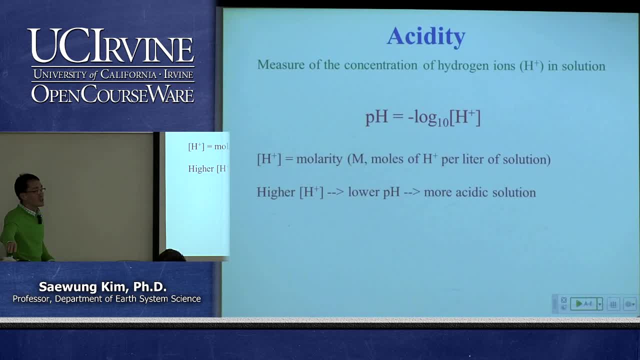 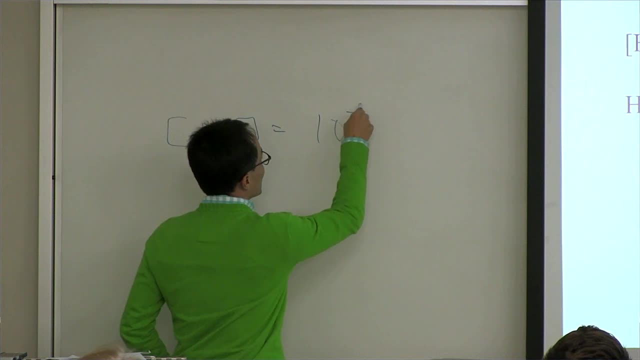 So usually, Okay, Okay, Okay. So the concentration of this H plus is very, very low. How low. In the neutral water, concentration of H plus is 10 to minus seven, right? So what you want to do is that we just want to take this seven away instead of right. 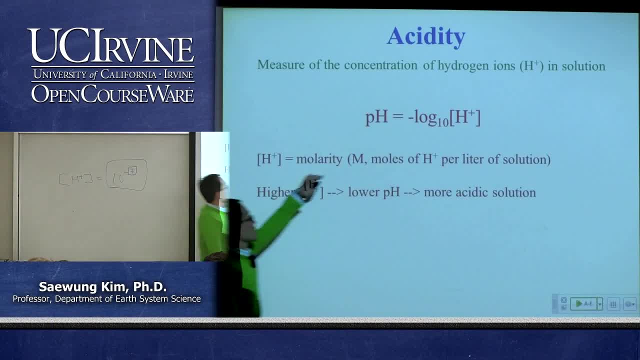 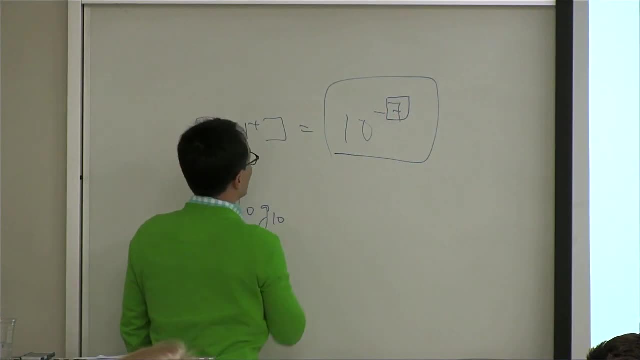 this whole thing. So what This log scale, So what the log base 10 is doing out there is that take this thing, just take this thing to the this pH scale. So if you put the log 10 in front of this very, very small number, then it will become: 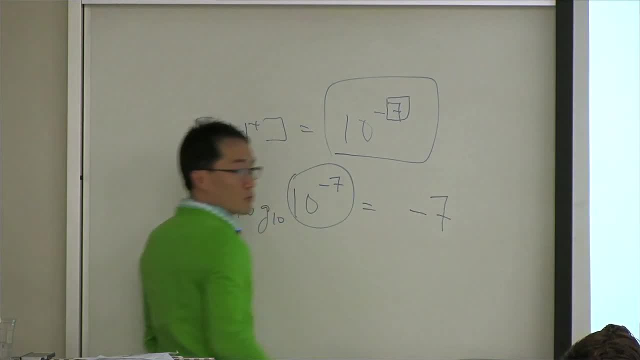 minus seven. So we just bring this thing into right here. But we don't want to use minus, So put the minus in front of it. Okay, So make this thing plus. So that's how log is working in terms of the number notation, right? 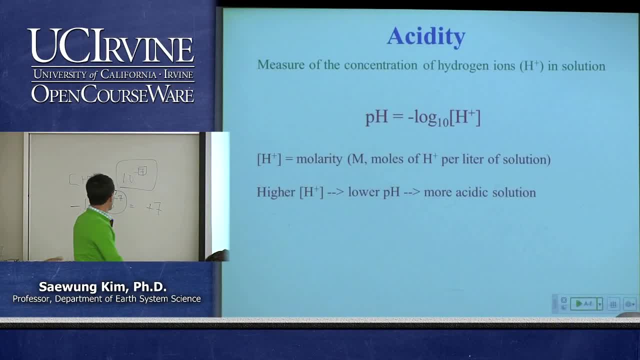 So that's that. So because we're putting minus in front of log, so that's the important part. So lower pH means higher concentration of the H, plus right. So because of this minus thing, So lower pH means more acidic And then higher pH means less acidic. 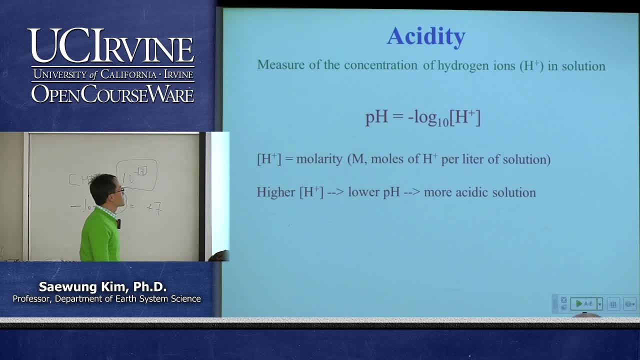 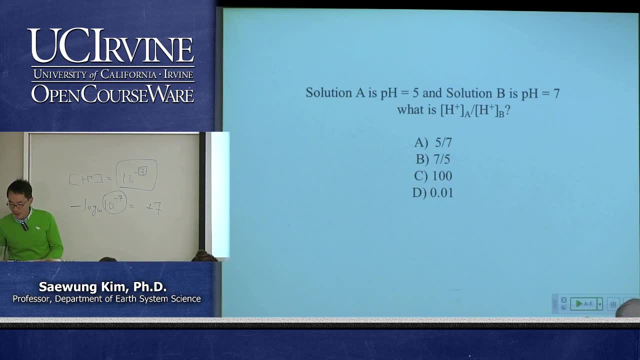 We call it basic, okay, So let's do this thing. Let's play with this little quiz here So we learn about log. Let's apply that thing. So solution A has pH five, Solution B has pH seven. What's the concentration ratio of the H plus in solution A? 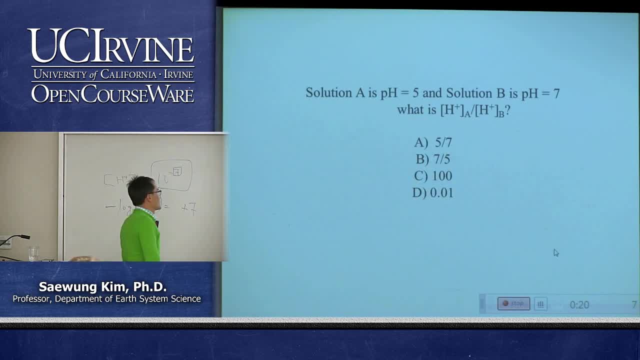 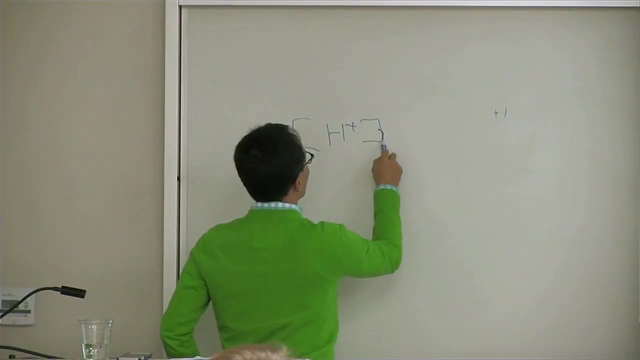 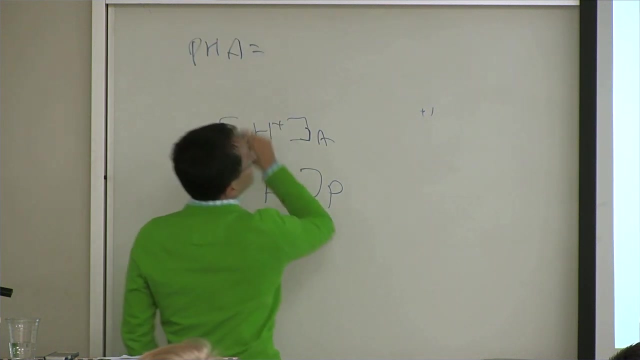 And solution B. So what's the concentration ratio of the H plus in solution A? Solution B: Okay, A H plus B, P, H, A, 5,, B 7,, 10 to minus 5,, 10 to minus 7,. so 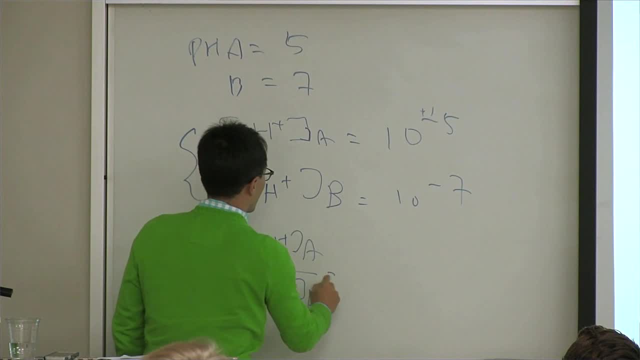 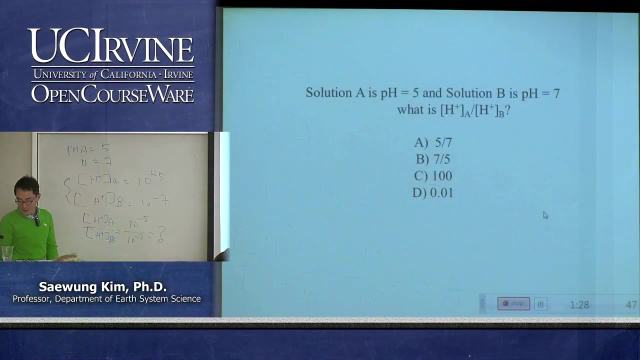 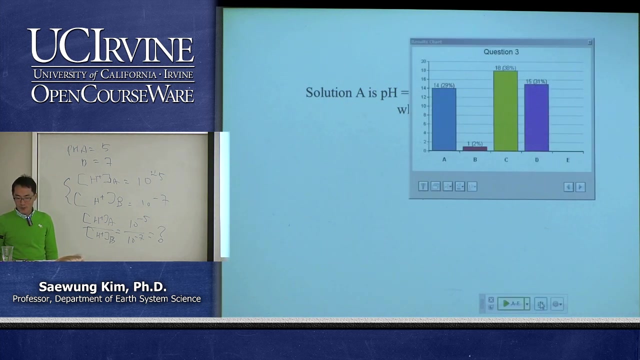 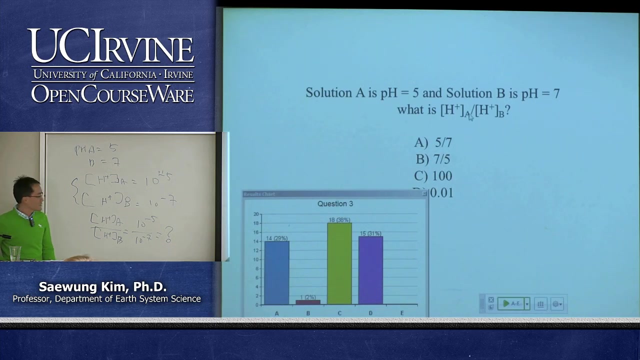 A, B. right, It's all here. We got everything All right. 47, 48.. Ooh, that's a competing answer. Even A, Please. So that's so. it should be 100, right. 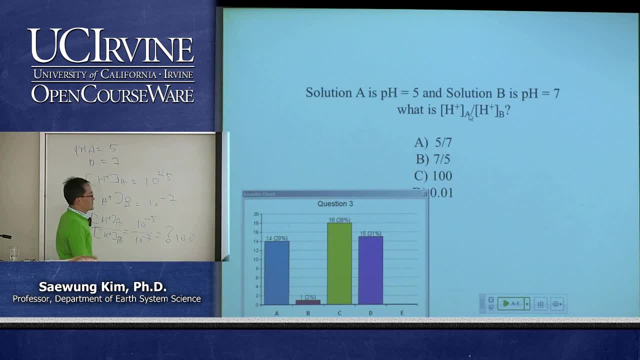 So what's the right number? C, Yeah, at least that's the most dominant number. anyway, Only 38 percent By end of this quarter. before you take your final, I hope you can understand this thing. okay, You know what I mean, right. 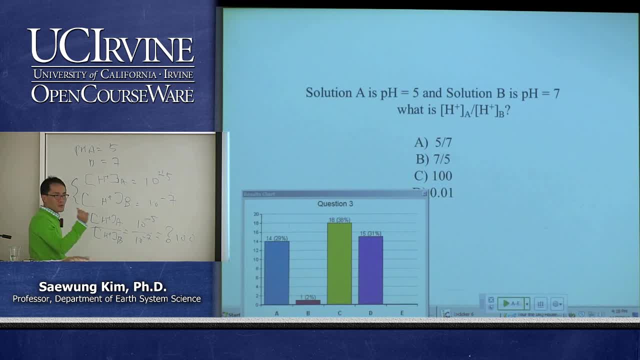 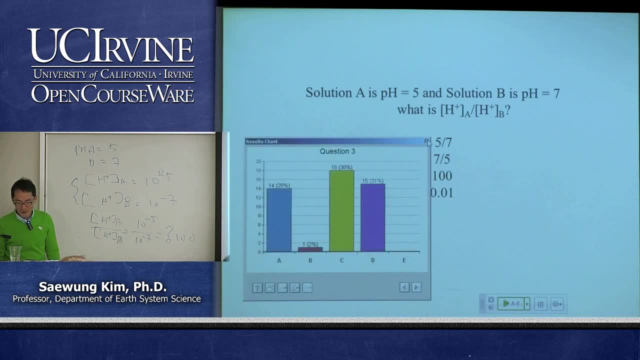 So anybody still confusing? It's pretty straightforward, right? You just want to play with me a little bit to choose the wrong answer, But did I tell you that I? I can actually see the name of the? what kind of answer you choose. 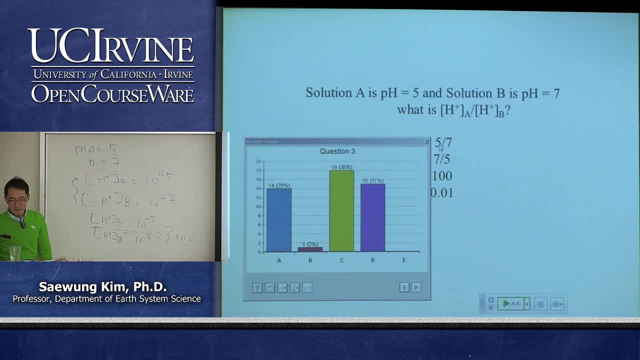 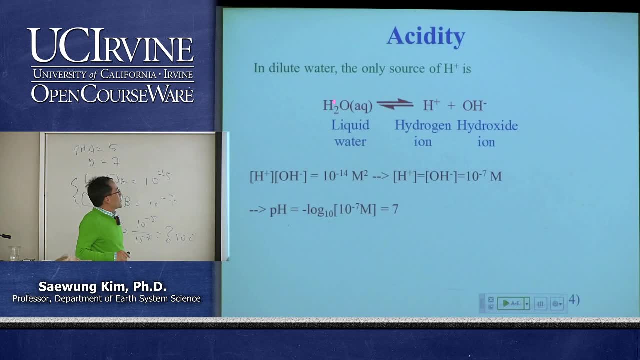 So you gotta, you gotta, keep in mind about that fact. All right, So let's move ahead. So acidity, I talked about that. the water which is, if it is only water, basically neutral water, has equal number of H plus and then OH minus. 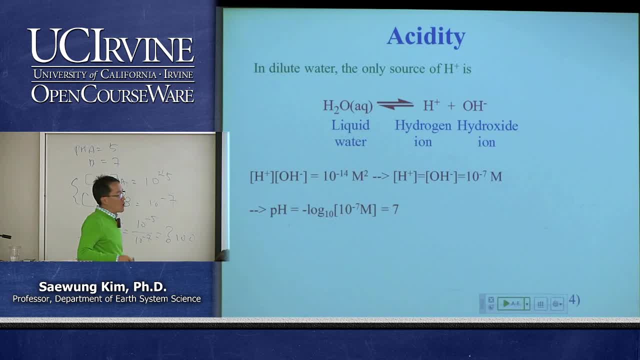 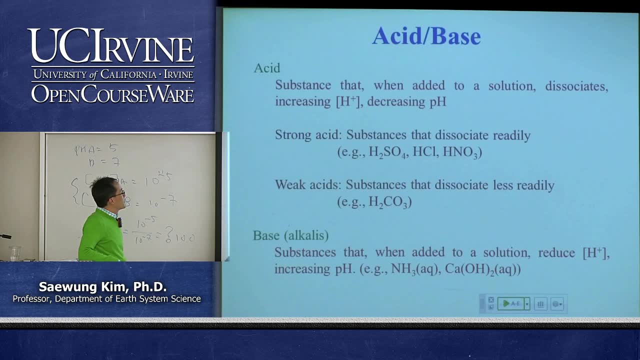 And then that's 10 to minus seven. That's why neutral water has pH seven. okay, Seven is seven, Seven is the magic number. This is a neutral. So in the world of acid, this is same as the human world. 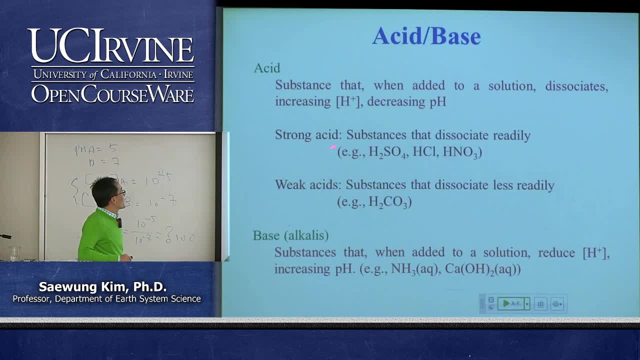 There's a in the human world there's strong guy and weak guy out there, But in the acid world there's also strong acid and weak acid, right? So strong acid basically, if we basically define that concentration of H plus. 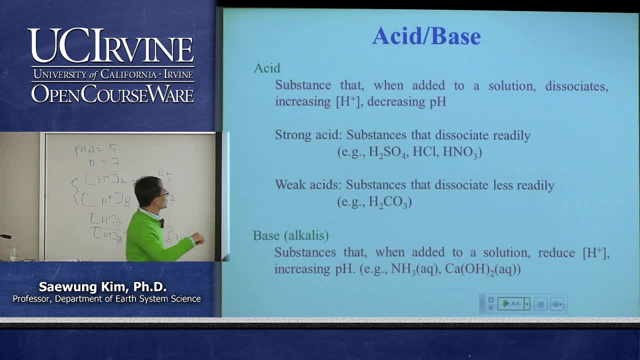 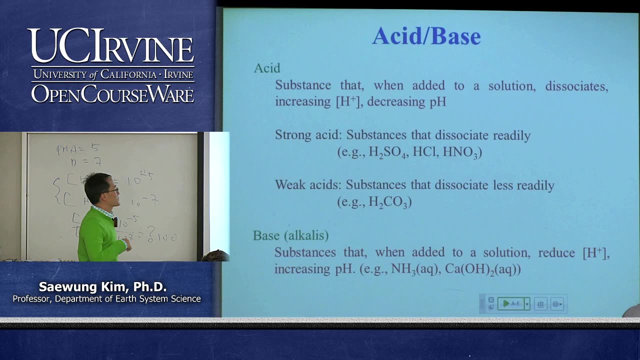 determines the acidity. so a strong acid by definition is that these guys actually can easily produce H plus when it dissolve into the water. So that's by definition, strong acid. So weak acid. so this H2CO3 is not as strong. 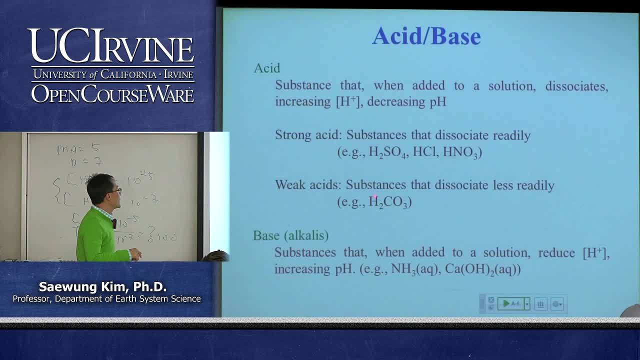 as the suffragic acid NHCl. That means that this acid actually make less H plus when it dissolve into the water. So that's the definition of the strong acid and weak acid. And then any substance that takes H plus away, for example this ammonia can take the H. 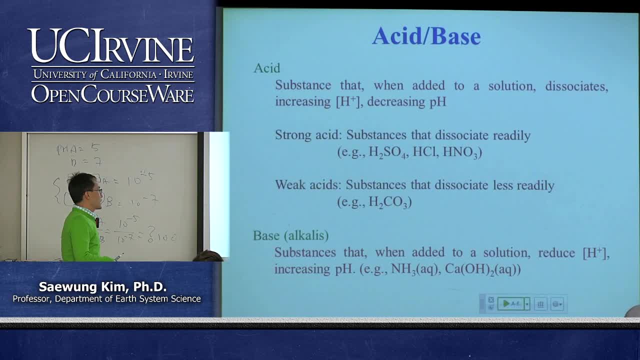 plus away from the solution and then it becomes NH4 plus. so that's why this is basic. and then or it can produce. when it produces the OH minus, it is also a base, So we call it alkali, but we will more focus on the acid during this class. okay, 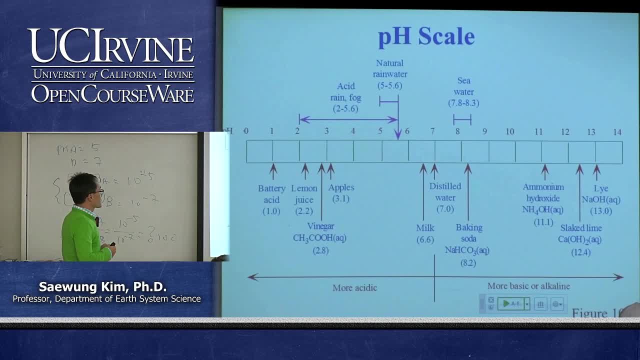 So this is the range of the pH that some different waters around the nature, so this is kind of a seawater, slightly basic, so the pH level is about 7.8 to 8.3.. Even the natural rainwater is slightly acidic, so pH range is about 5 to 5.6.. 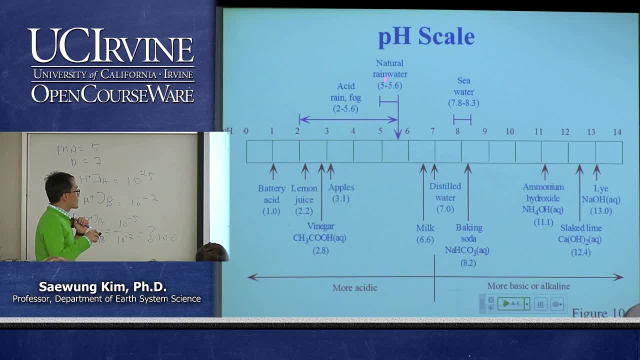 So we call it acid rain when S the concentration of H plus goes up, So pH level below 5, so that's the definition of acid rain. so usually it is observed about 2 to 5.6 of the pH level. for the acid level. 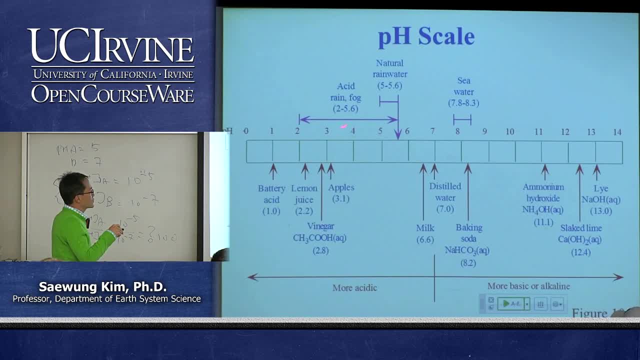 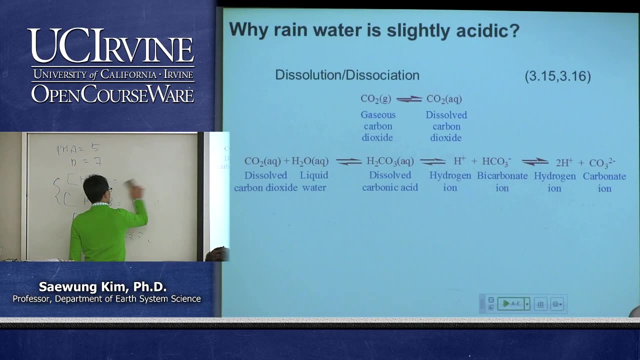 I should change this number right here. so somewhere between 2 to 5 is acid rain range by definition. okay, So why? rainwater is slightly acidic. So anybody remember What's the CO2 concentration in the atmosphere? Good number. anybody can say, too, about their CO2 concentration. 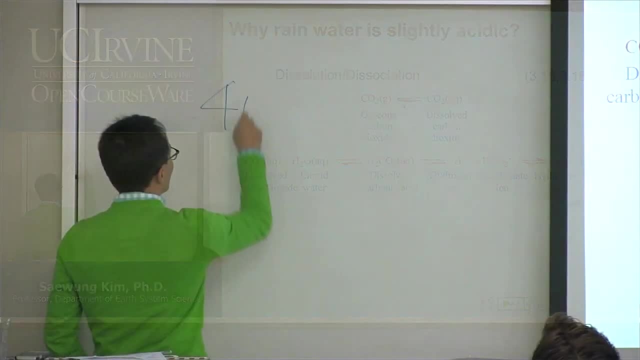 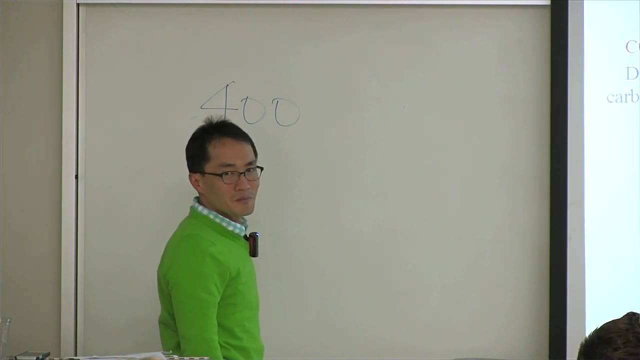 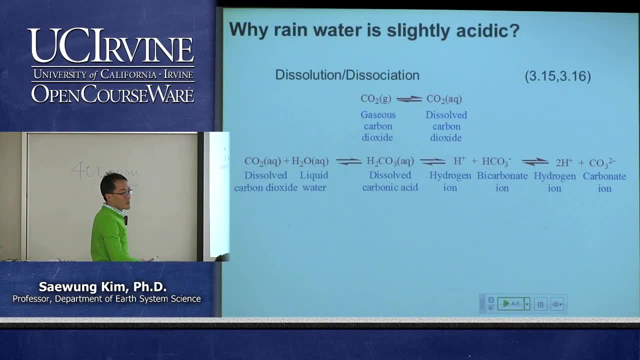 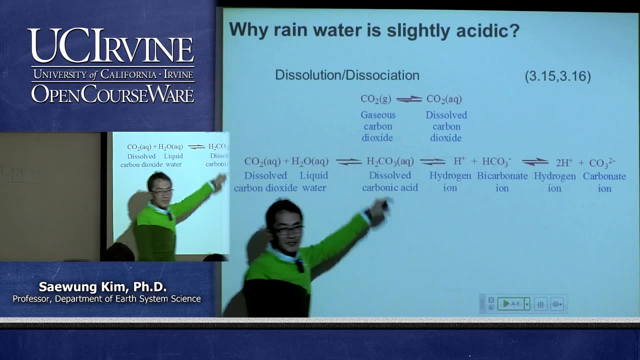 Looks good, right? Yes, very good, Right. That is a little bit copper-like, right There one is there too. Look at that. So this is the was the ocean washed asideります. Right, That is. you see, a lot of space. 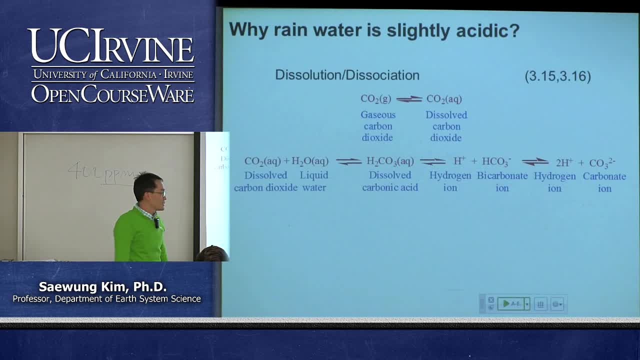 isn't it? And it is possible that didn't we come too close? because the water flow over here, the right, So that's part per million right, So that's a lot of CO2 in the atmosphere and then they can desorb into the water and 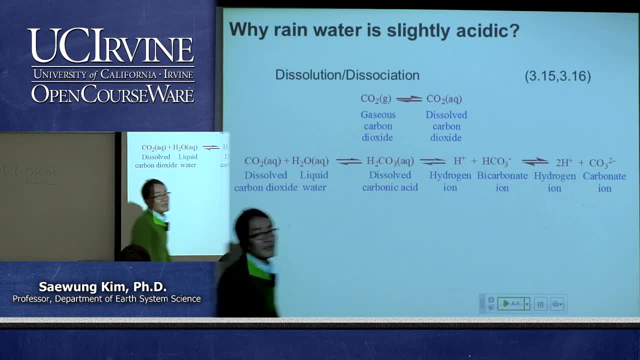 then it can produce. what is this thing? that's acid, and then that's relatively weak acid, right? So that's why it slightly acidic. and then we talked about the strong acid and the weak acid, Right, acidic. and then we talked about there's strong acid and then weak acid, and then this: 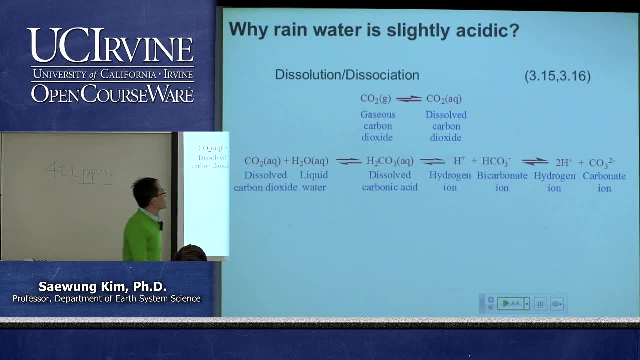 acid. carbonic acid is weak acid, so that's why rainwater is slightly acidic. and then- this is a little side story- that we worried about CO2 concentration, because it will increase the temperature of the earth because that's greenhouse gas. Also, if we have too much of CO2 in the atmosphere, actually it will dissolve into the seawater. 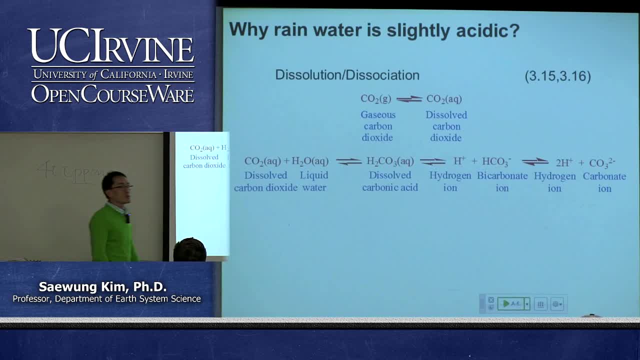 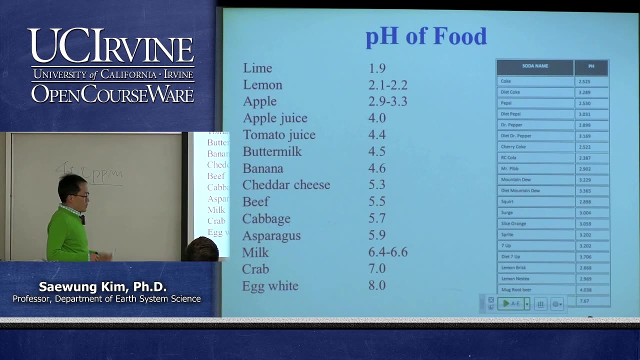 and then it will acidify the seawater. so that's another environmental problem that we will discuss when we discuss about the global climate change, which is, I think, two weeks away, something like that. So some of the foods pH. so, if you take a look at this thing, the pH from a soda: soda. 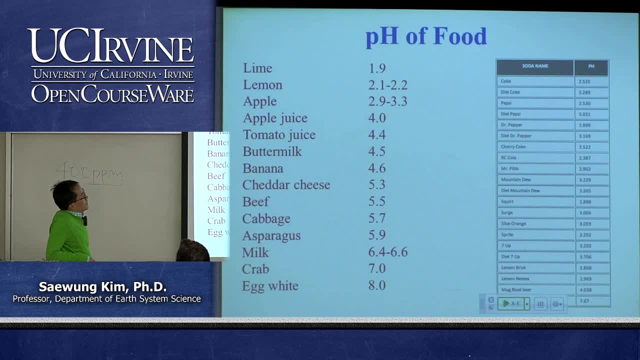 is a very acidic thing. for example, Coke and then Pepsi. its pH is about 2.5, it's kind of the strongest acid rain you can think about. It's this kind of pH range. so today the two lessons. if you're just sleepy, don't smoke. 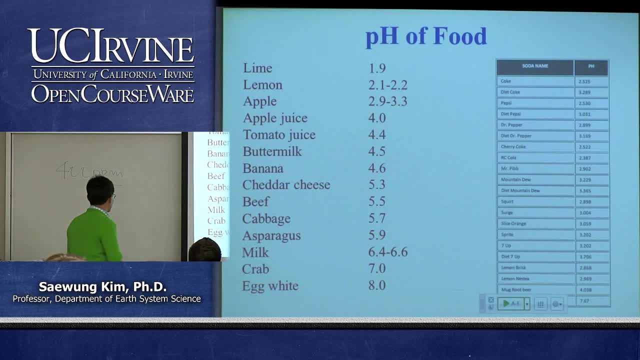 and then don't drink too much of soda. so that's the two lessons, but that's not going to be showing up in your final, so that will be good for your whole life. so that's a good thing, I guess. So some other stuff, that pH of the food, but something you can, it's good to know about. 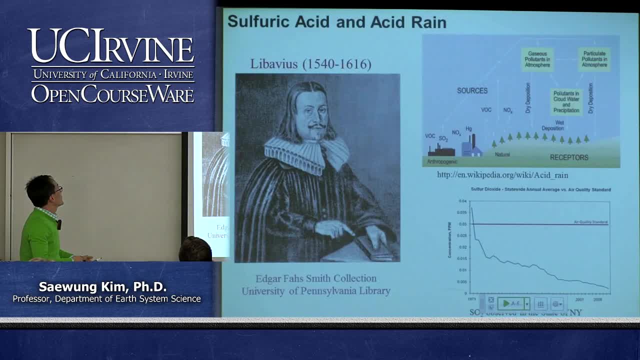 these kind of numbers because you now understand, Understand what pH means. So let's talk about modern day acid rain problem. So modern day acid rain problem is actually from sulfuric acid. So we know where sulfuric acid is coming from, right? 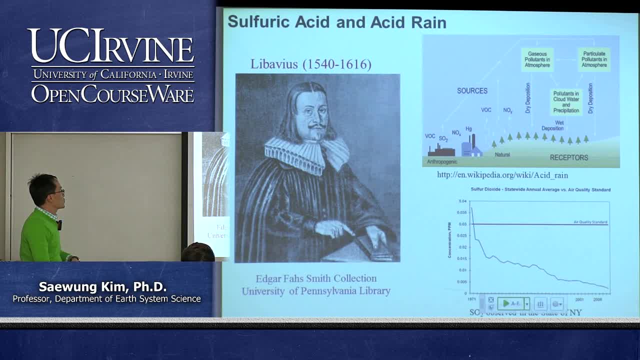 The coal burning right. So coal burning emit SO2 in the atmosphere and then the chemical process in the atmosphere make sulfuric acid. But this is kind of observation result from 1971 to 2007.. Okay, So in 2010, an SO2 concentration. it was really really problem back then in early 1970 that. 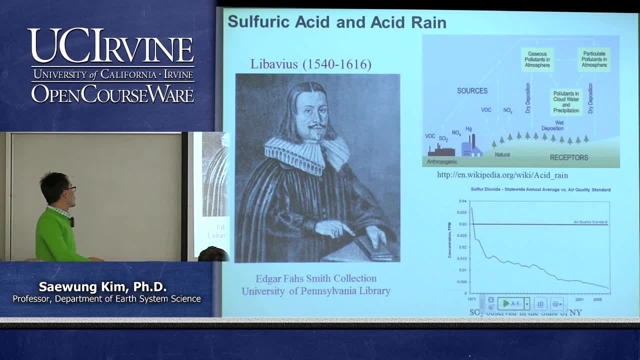 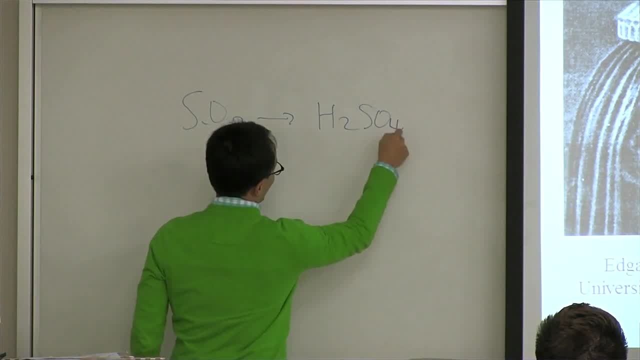 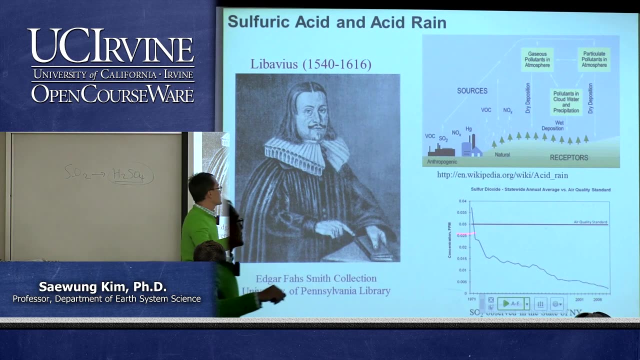 SO2 concentration is too high. So again, this SO2 eventually become H2SO4, which is sulfuric acid. So this is precursor for acid rain. So high SO2 means more sulfuric acid means more acid rain. So we address really good in developed world, especially in the US and in Europe. 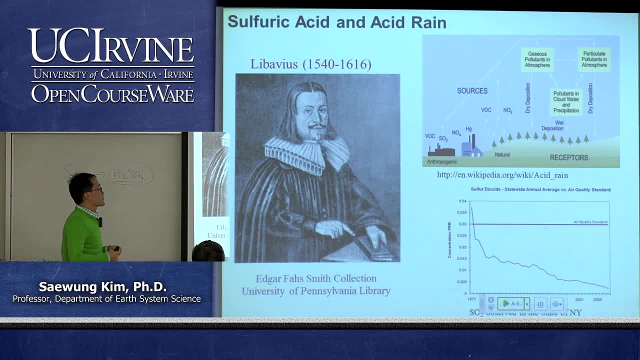 We decrease the SO2 level, not by less burning coal, more like they have a better technology. We discuss about the clean coal technology So we emit less SO2 to the atmosphere, so that this acid rain problem actually gets better past about 30 years. 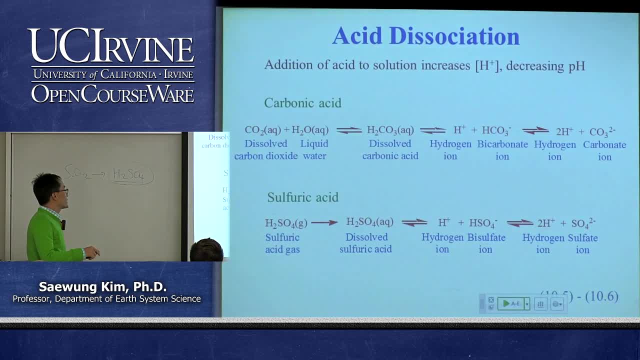 So this is comparison between carbonic acids. So this is weak acid, So it just produce less H plus than sulfuric acid. So that's why sulfuric acid is strong acid and then cause the acid rain problem. okay, That's all you need to know. 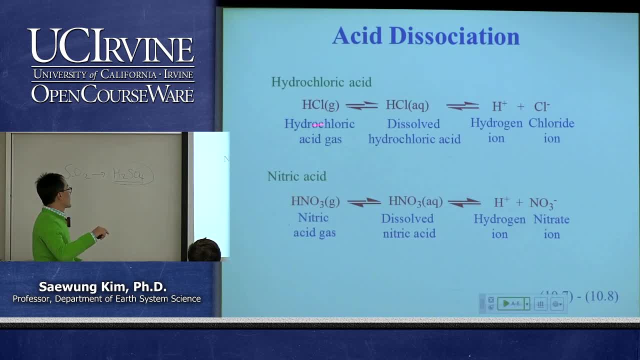 So, and then the other acid, the strong acid. we talked about HCl, So that this was a really big problem when that LeBlanc process was operating. but it's not really using anymore, So HCl is not really problem. Nitric acid. 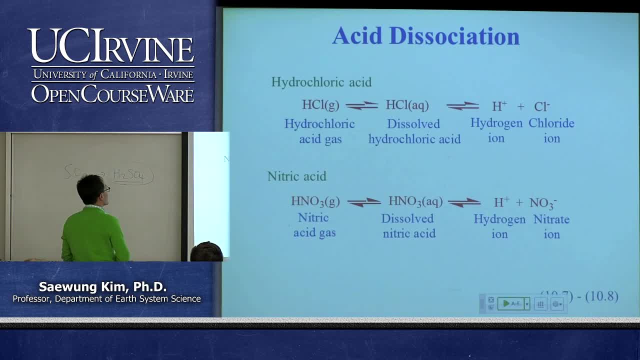 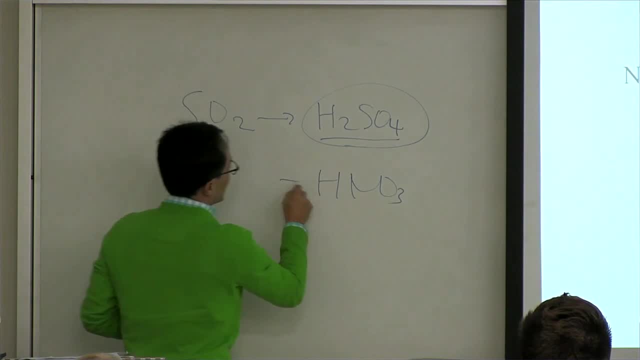 Nitric acid can be a problem, but not currently. it's not really big problem yet. So this: where is this nitric acid coming from? HNO3? So that's from NO2, from the coal, OH, and then HNO3 is coming from. 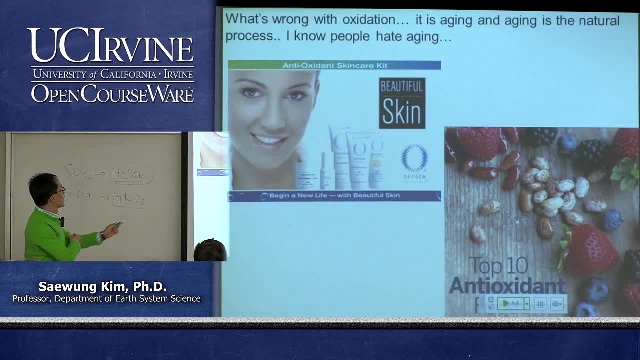 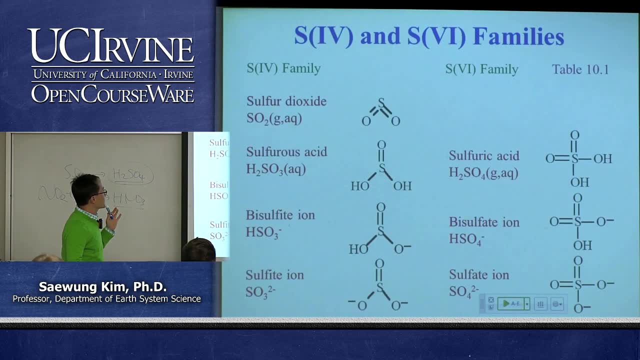 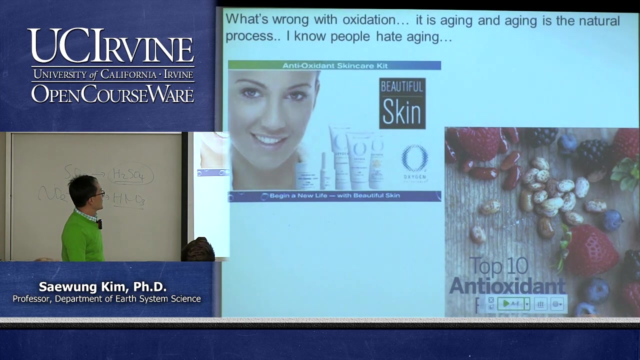 So this can be also precursor for acid rain. So I try to explain all this chemical kind of mechanism That how SO2 is becoming sulfuric acid, but I realize that's not really good idea. who really scare about the chemistry things like that? like you guys, rather. 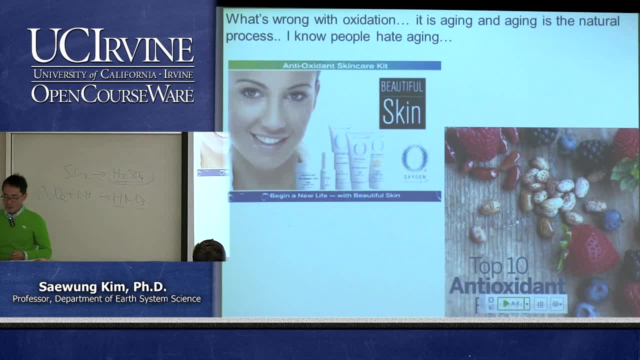 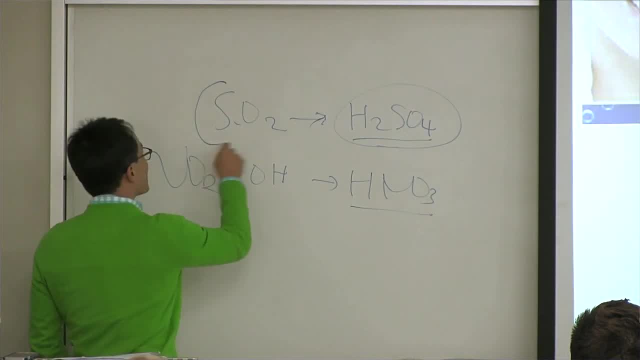 So I just try to really go back to basic thing. So, basically, this is oxidation, all right, So how do we know this is oxidation? So if you take a look at this, sulfur and nitrogen- Okay, It used to have two oxygen each, right. 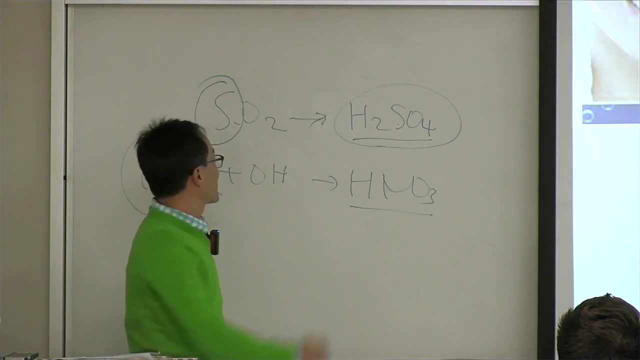 So how many oxygen this guy have. sulfur now Four. Four: There's more oxygen, right? This is not really scientifically right way to describe it, but easier to understand this thing. So how many oxygen this nitrogen has? Three, So this guy now has more oxygen, right? 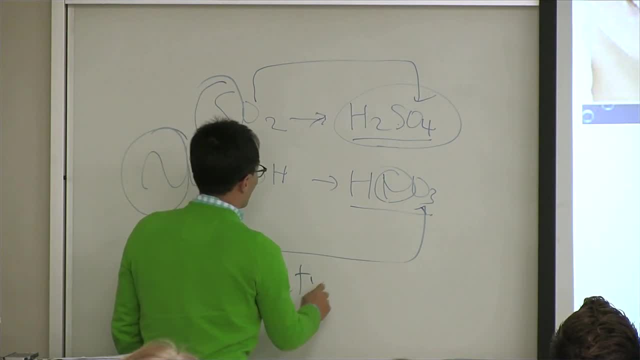 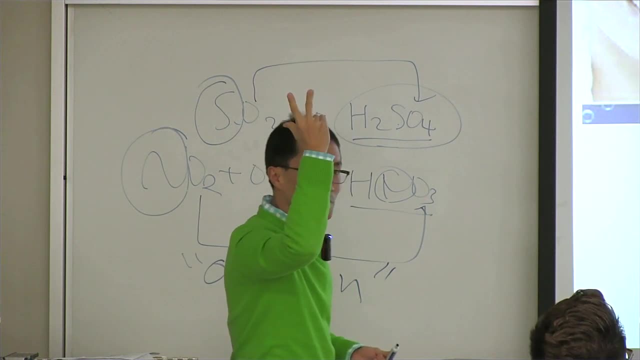 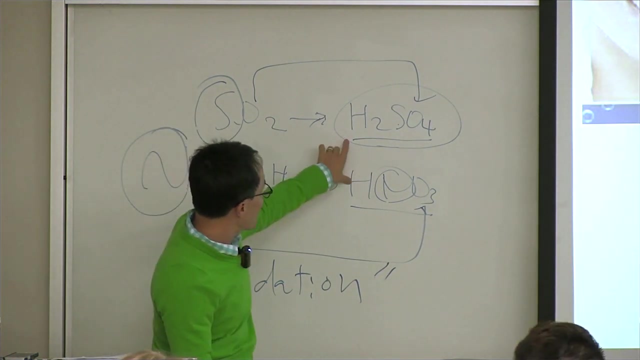 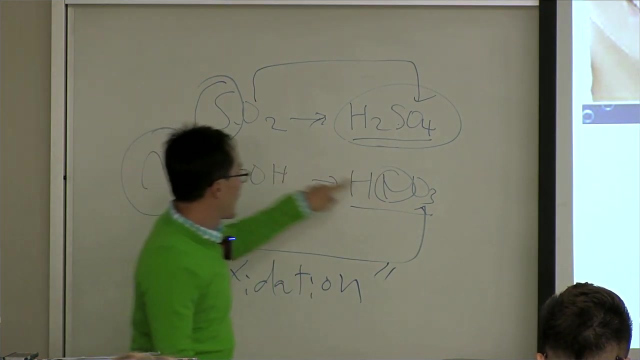 So this is called oxidation. Okay, Okay, Okay, Okay, Okay. So when air pollutants gets into the atmosphere, what is happening? It's oxidation. and then, if you just take a look at this compound and this compound, sulfur happens to have more oxygen here and nitrogen now has more oxygen in this form. right, 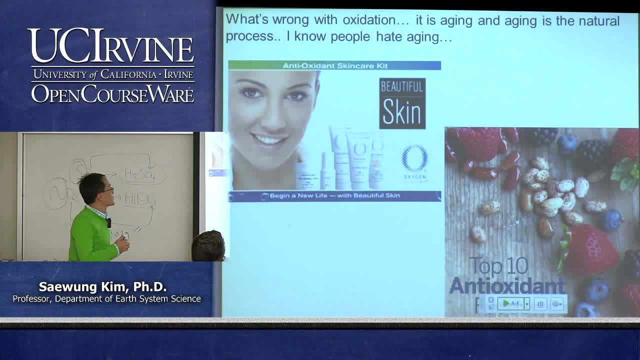 So oxidation is kind of natural processes, right? So if you take a look at all those kind of thing- antioxidants kind of thing, that's all related- People are just putting all those cosmetics on the skin too, and then they claim that. 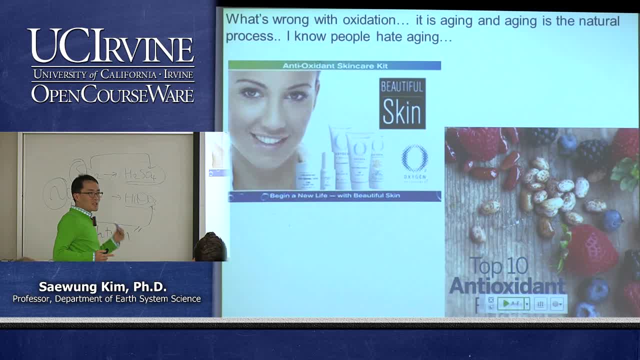 that's antioxidant, which means that that kind of slows down your aging process. So aging process is also oxidation processes, and then people try to eat all those berries and things like that and then people claim that that's antioxidant. so by definition it means that slows down your aging right. 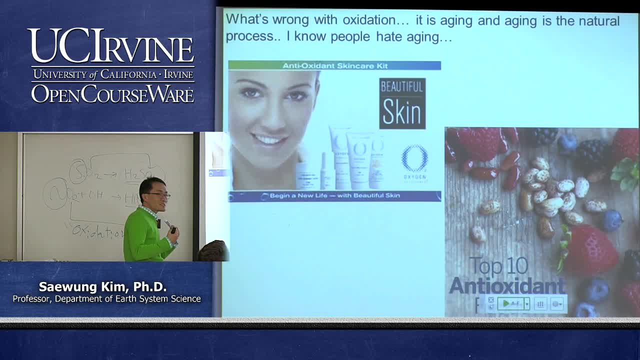 So basically, we people are also getting oxidized in the world, which by definition is aging, and then these air pollutants are also getting old and then getting oxidized, and then these guys are water soluble and then they are removed from the atmosphere by the rain things. 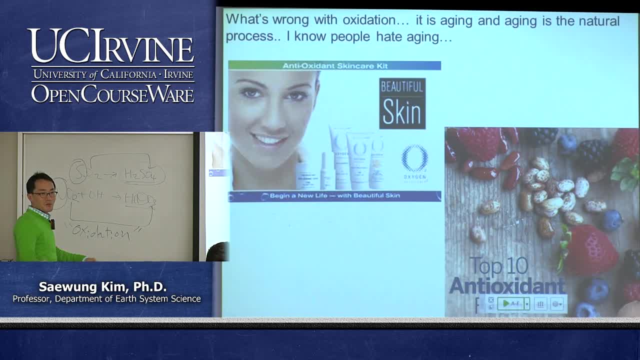 like that. Basically, these pollutants die from the atmosphere. Okay, As it gets aged, it gets oxidized, right So understand. Yeah, So people hate aging, probably your age aging is not really a big problem, not in scope. 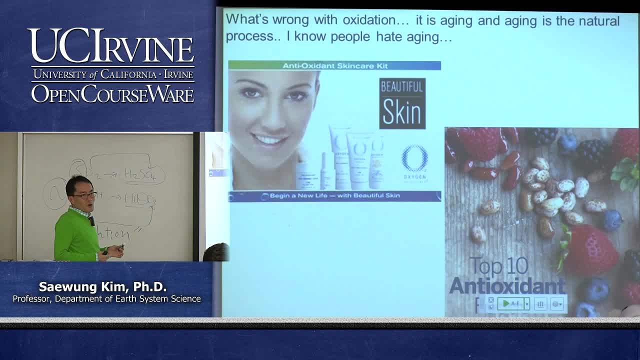 and then once you get to 21,, 22-something, once you get to the ball and then ask the alcoholic beverage, you get called. and then you're kind of annoyed by that why this guy is asking. the call things like that. 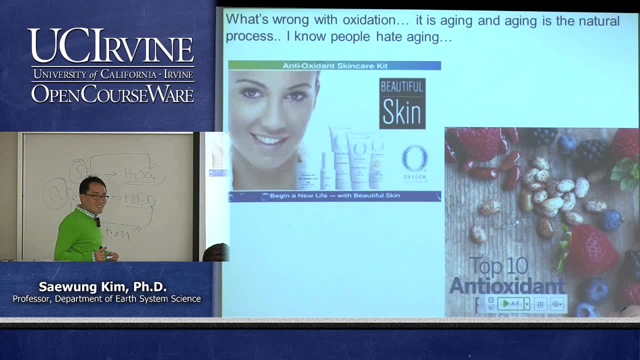 But once you get to my age, people start to not asking the photo ID. you start eating this antioxidant and then putting this stuff on the face to getting younger. So that's life. So everything is related. So that's what I'm trying to say here. 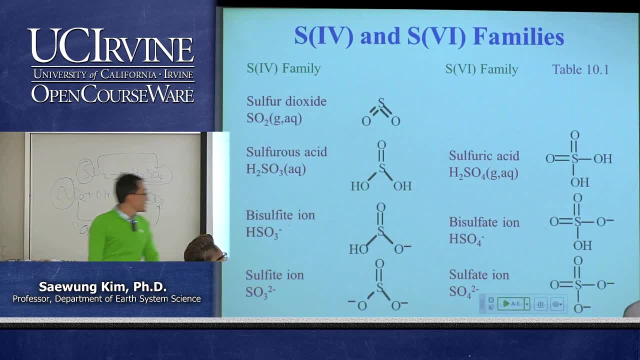 So if you are a science geek then you can take a look at this thing and then this is SO2 right here and then SO4 right here. Actually, the really right way to describe this oxidation is calculating oxidation number, So SO2.. 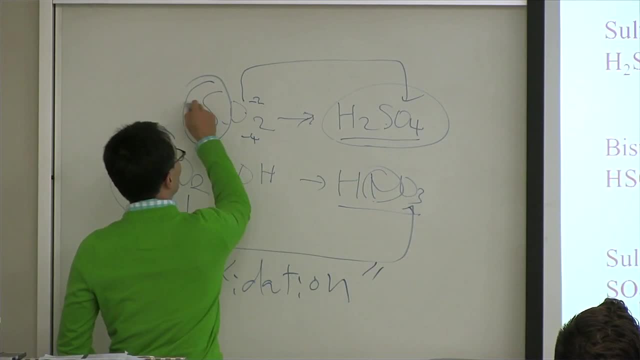 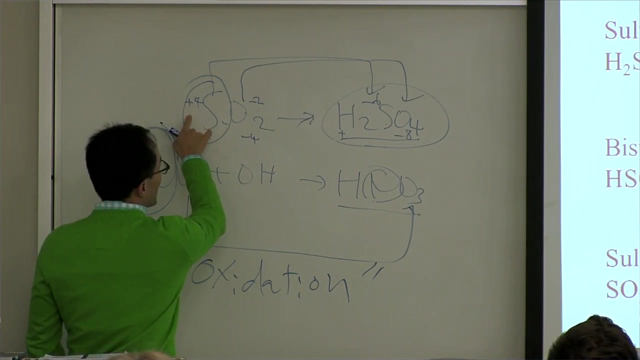 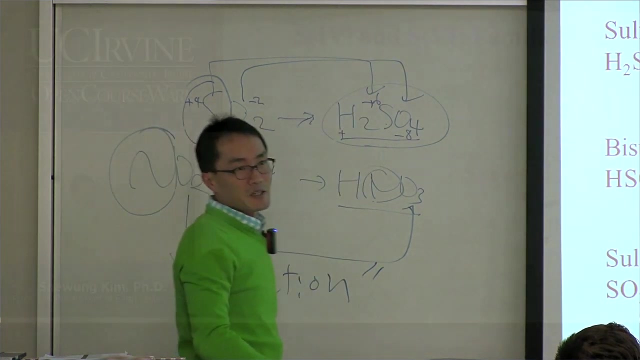 This oxygen has minus two, so that's minus four. that's plus four here, and then that's minus eight. H is plus one, so minus six. So basically, sulfur oxidation states change from that's plus six, right, So plus four, to plus six. that's the right description in terms of science world. but 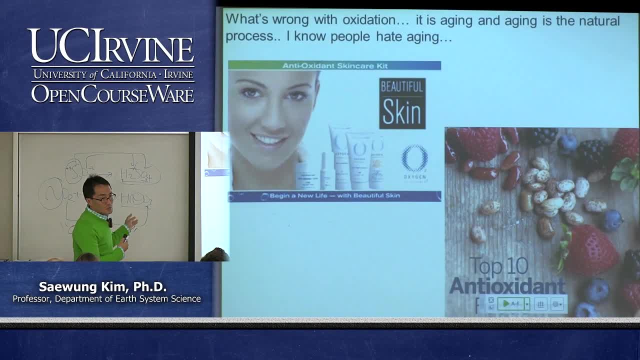 in your world. I think it'll be just fine. It's air pollutants getting old and then die from the atmosphere and then removed by the rain. Okay, And then that cause the acid rain, that problem in terms of air pollution problem, Right. 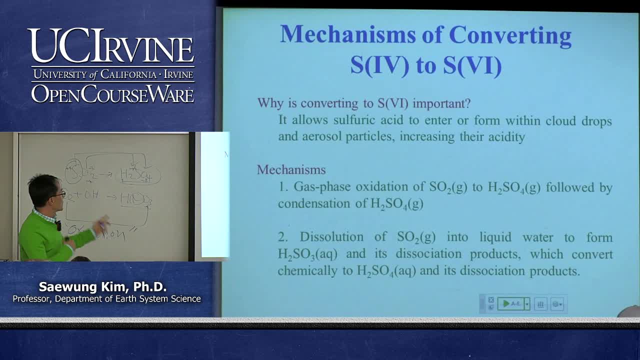 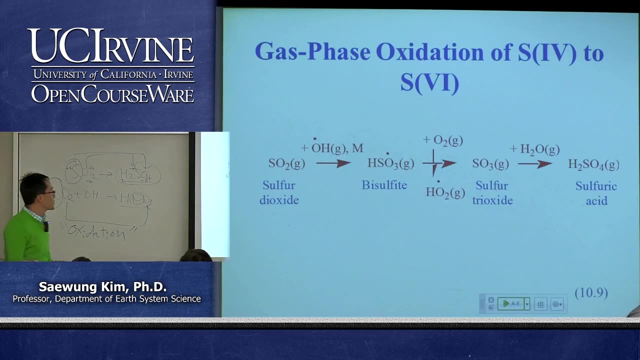 So I have 20 more minutes So you can just read from this thing. So that's really scientific exact description about oxidation of a sulfur compound in the atmosphere. So there are two way to actually we can oxidize this sulfur- Okay, This sulfur in the atmosphere. 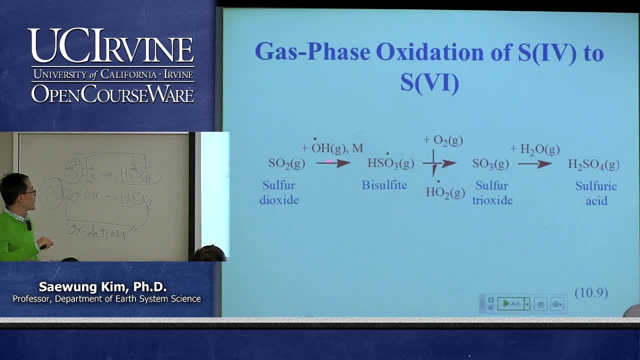 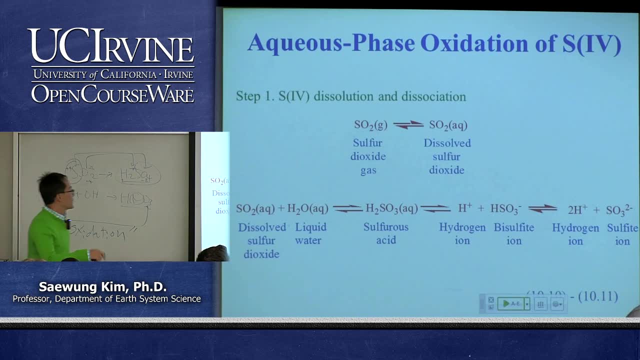 One is gas phase process that is done by the OH radical, producing sulfuric acid. The other one is actually this SO2 dissolving into the water and then producing sulfuric acid. So what you need to remember is that there's two different way to produce sulfuric acid. 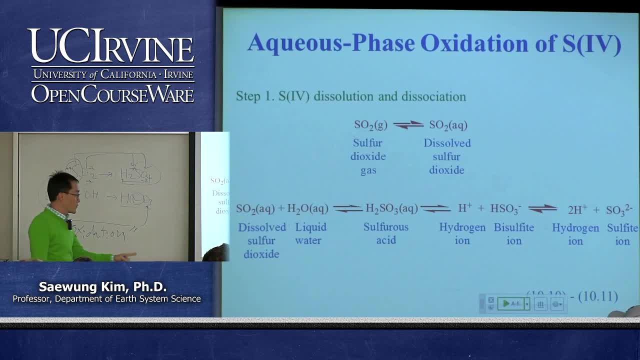 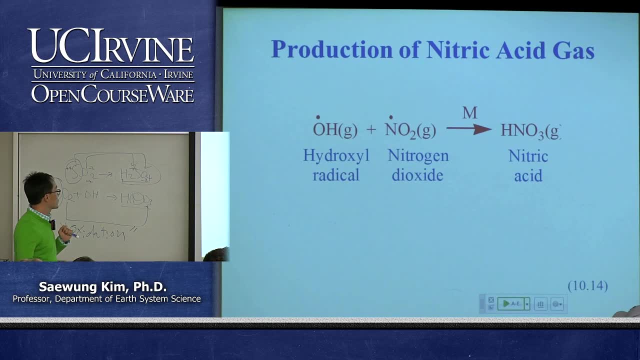 in the atmosphere, and the sulfuric acid is important precursor for acid rain, right? So that's all you need to remember. This is how you can make nitric acid. So let's take a look at the consequences of this acid rain problem. 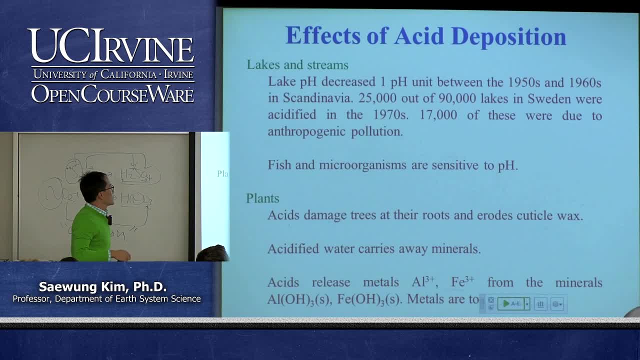 So in early 1970, so pH gets all the way down to a lot of times we observe pH one in 1950 and 1960, all the way up to 1970.. So for the perspective, to give you some perspective, So what's the pH? Okay, So the natural condition of pH of the rainwater pH is five, right? So H plus is about 10 to minus five. concentration pH one means H plus is 10 to minus one. So this is 10,000 times higher in terms of H plus concentration in pH one. 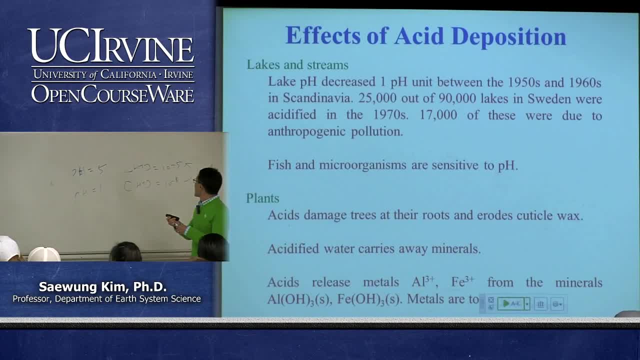 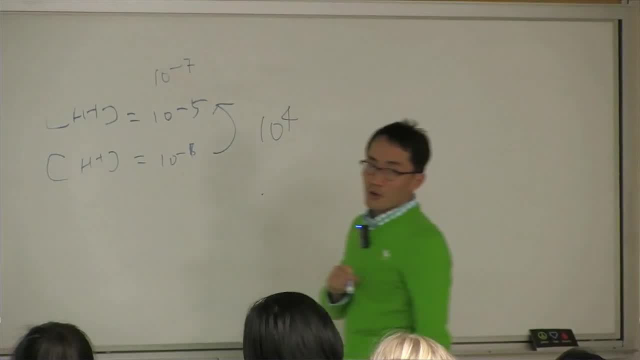 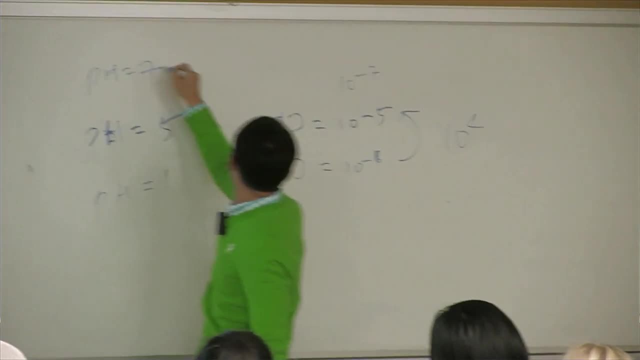 In terms of rainwater in natural condition, If you compare with the neutral water, which is pH seven, which is 10 to minus seven, So this is pH seven, right? So that's about 100 times so 10 to six. 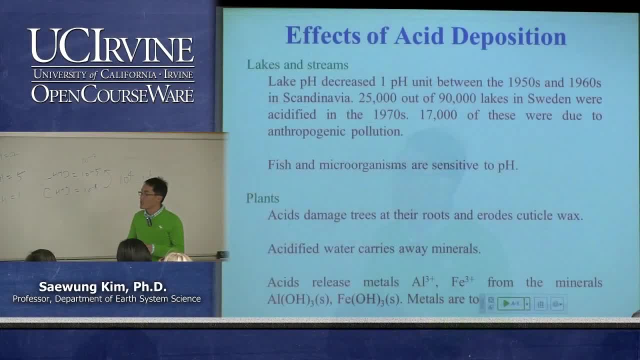 So million times higher in terms of the H plus concentration. So that was that bad, Although if you compare with the water, you know you have a lot of water. so H plus 10 to minus seven, you compare with the one and seven. 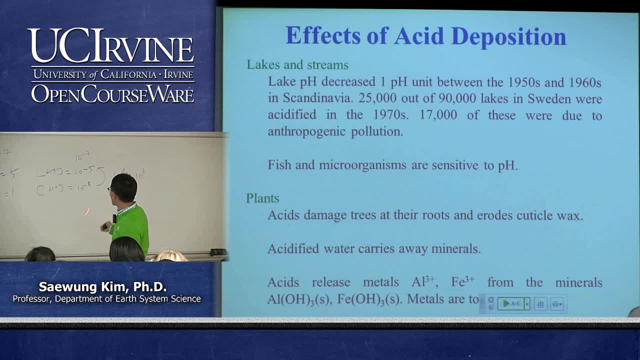 it looks like a very close number, But if you take a look at the real definition of the pH, that's million times higher H plus concentration in the lake water or the river water. So that obviously affects on plants. So you can read this thing: 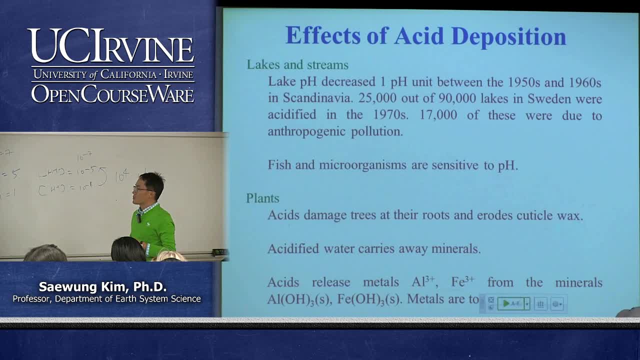 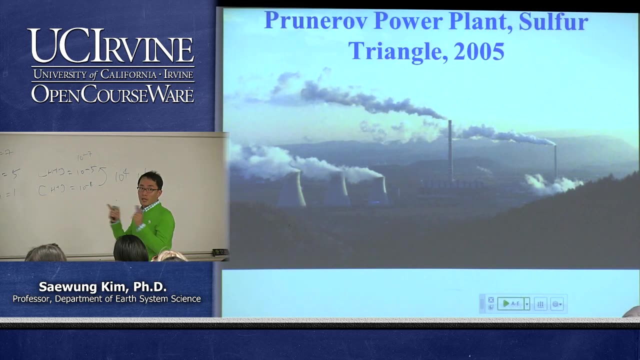 So it can just basically affect on the root system And then if just trees loose, get damaged, then basically trees is dying from this thing. So this is the emission of the coal-burning power plants. So this contains a lot of SO2 that will produce sulfuric acid in the atmosphere. 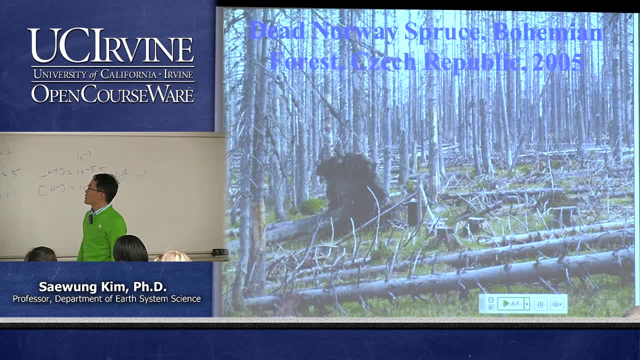 So these are consequences. This is Czech Republic of 2005.. Even in the 2005, acid rain was the problem in European country. So a lot of trees died. So a lot of trees died because of this acid rain that basically affected on root system for these trees. okay. 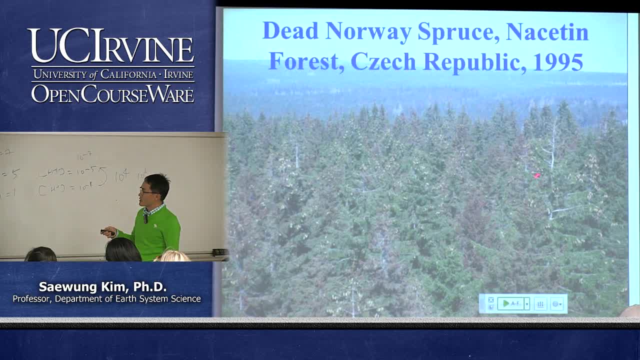 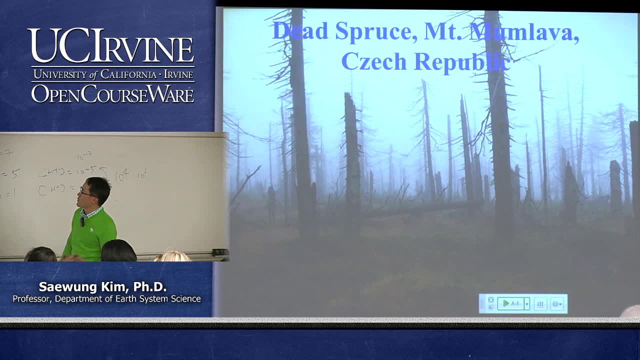 So again Czech Republic. You can see some dying trees here and there. This is 1995.. And then again the Czech Republic. And then there's dead spruce here and there, all because of the acid rain. So again all those sad photos. 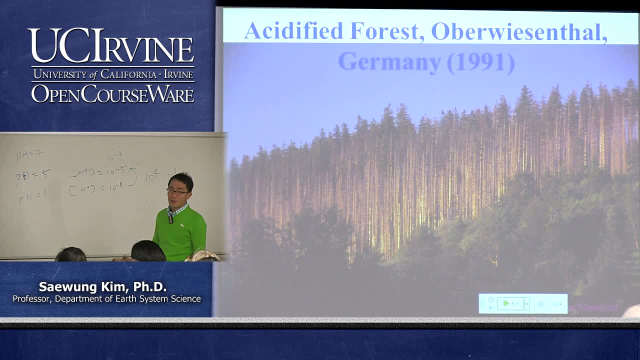 even in Germany in early 1900. So even in Germany there was a big problem in acid rain, even in the early 1900s, Even in the early 1900s 1990.. But now they address this problem. 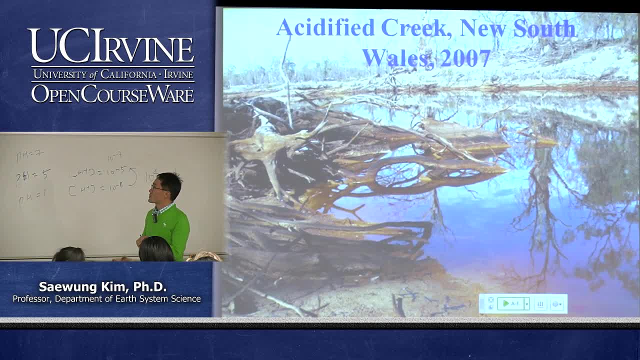 by reducing SO2 concentration in the atmosphere. So in UK. so a lot of tree got died and then all those kind of acid, those acid kind of dissolve all those material, tree material, And you can see the color of this water has actually changed quite a bit. 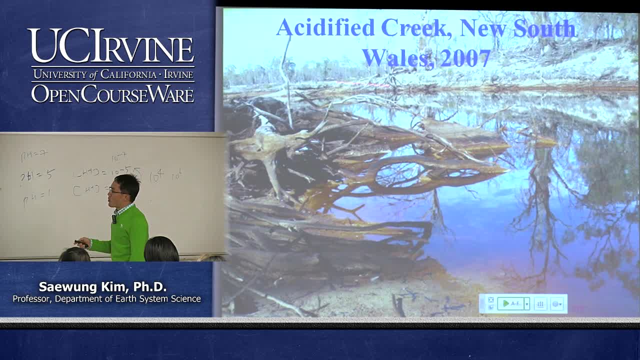 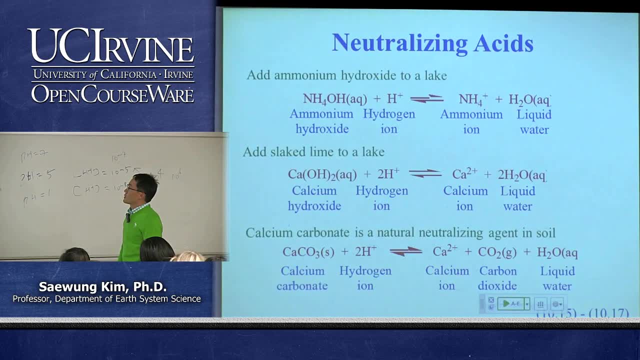 because the acid actually dissolved some of the tree parts. because the acid actually dissolved some of the tree parts And then a lot of organic material actually dissolved in this water. That's why it just has different color. So there's a couple of way. 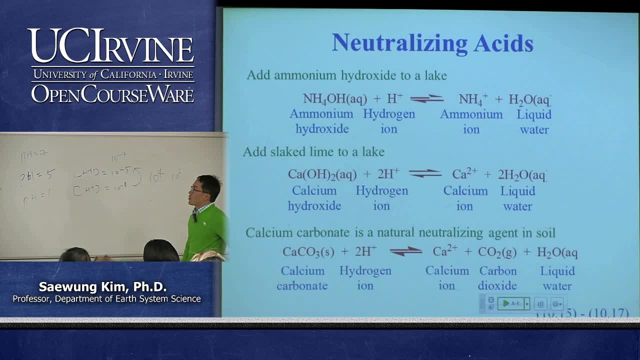 that you can address this problem by engineering. By applying some base alkaline material to the water, you can actually neutralize lake water. So people use the ammonium hydroxide and then calcium carbonate and then to remove the acid, And then calcium carbonate and then to remove the acid. 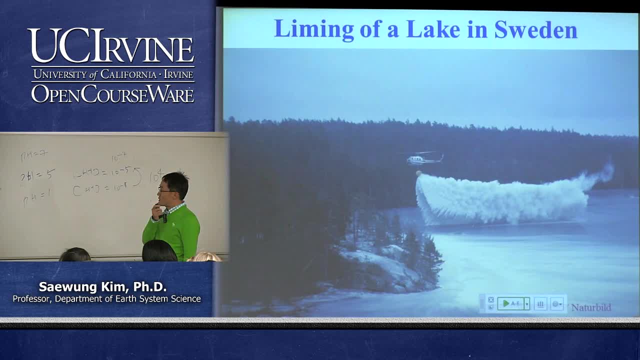 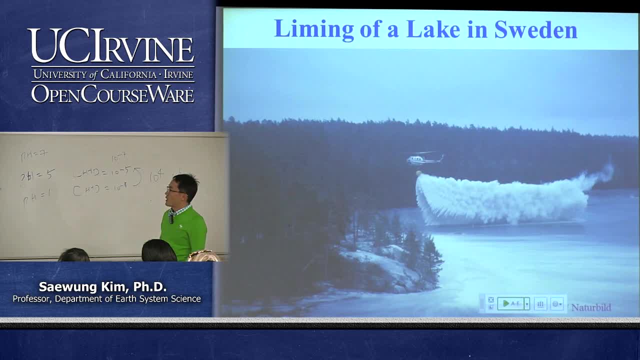 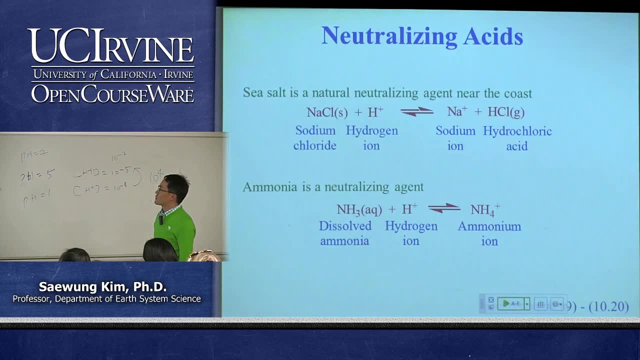 in Scandinavian Peninsula. in Scandinavian Peninsula, Actually, there's a helicopter actually spraying those alkaline materials to the water so that remove H plus from the water. So this is one way you can do. So you can put the NaCl by taking H plus away from the water. 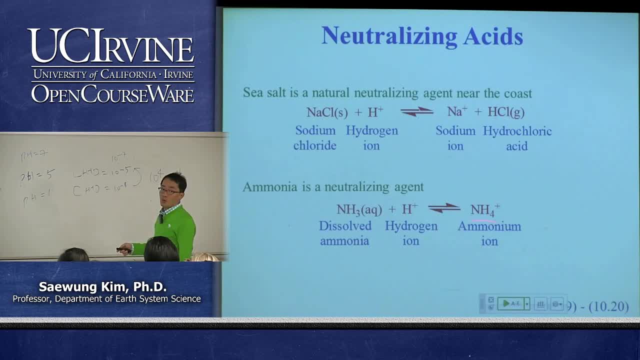 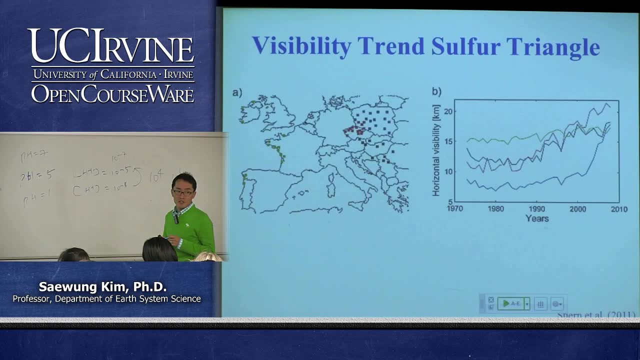 a way to address it. but you can obviously can take the H plus away from the water, So this is one that you can do, But real, fundamental solution to address this problem is obviously decreasing SO2 concentration in the atmosphere, which is precursor for sulfuric acid right. 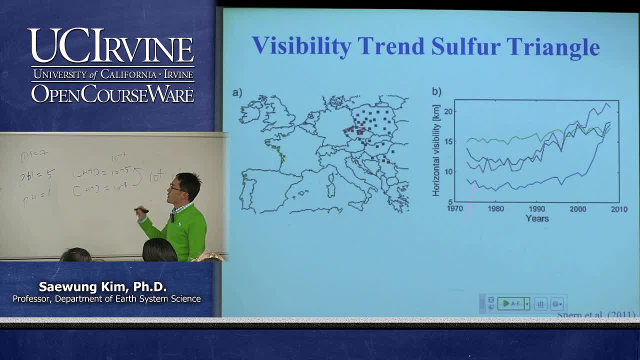 So, if you take a look at the visibility trend in Europe, so this is a green region right here. So this is Spain, right, What country is this? is Anybody? France, right, Germany, So this is Poland, I think. 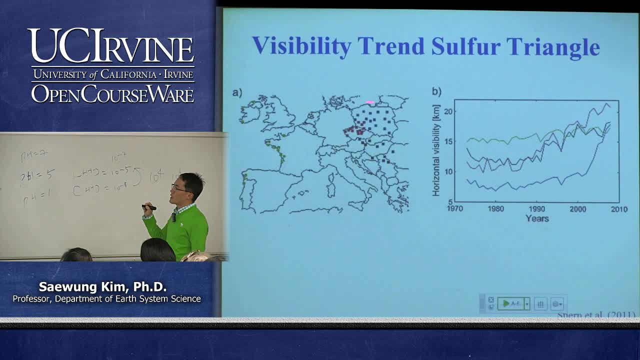 Poland and this is Czech Republic. So a lot of power plants happen to be located in this borderline between Germany and then Czech and Poland. So if you take a look at the red and then blue places, So this is visibility. So we discussed about the visibility. 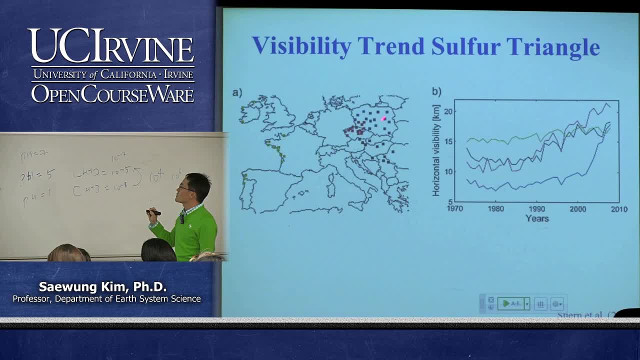 So, as you can see, visibility was really horrible in this blue region in Poland region Out there back in early 70s because of that. all those emission from the power plants produce particle in the atmosphere and then SO2, actual particle, decrease the visibility as you can see here. 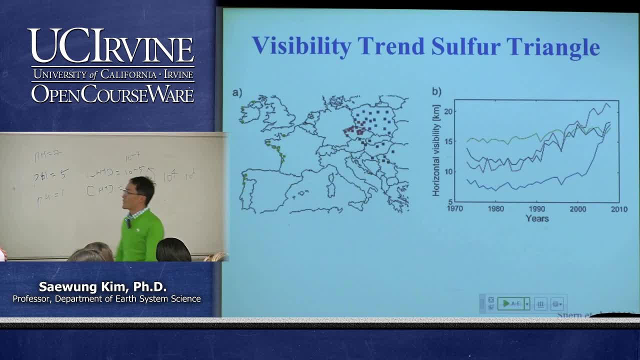 And then also the SO2 can make the sulfuric acid, and then that caused the acid rain problem and then it just killed all the trees in the ecosystem. right, But if you take a look at the visibility trend, actually it gets much better these days by reducing SO2.. 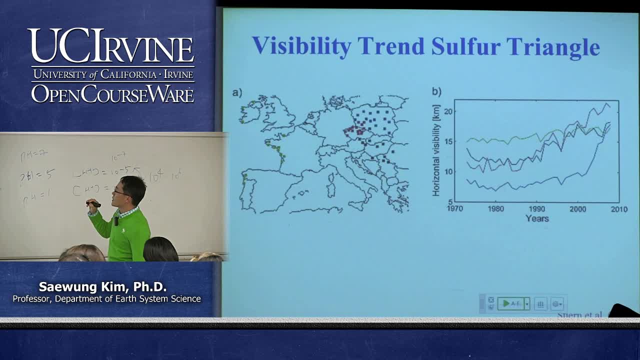 SO2 emission in this area, So in the Czech and then this Germany borderline too. Actually the visibility gets much better. But if you take a look at this nice beach cities in France, there's not much of the power plants beginning, So visibility is about the same right. 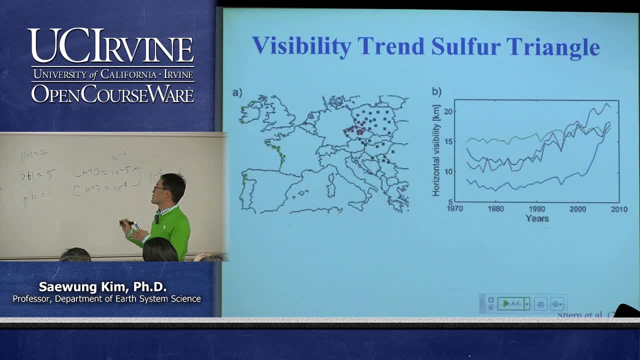 So you can learn this: if you take a look at the different region and different industry and the visibility trend, you can actually take a kind of a guess that what kind of improvement has been done in different region. So this is in the US. 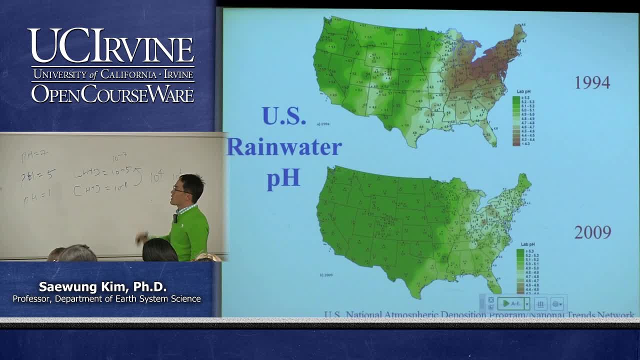 So this is in 1994,, this is 2009,. and then this is pH. Higher pH means that less acidic right. Lower pH means more acidic right. So basically in the western part of the US has been pretty clean. 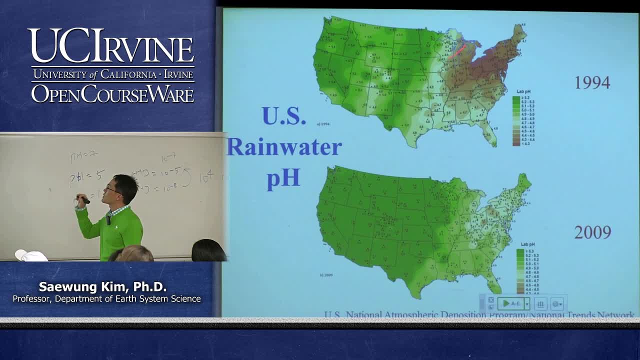 but in terms of acid rain, acid precipitation. But really big problem has been Ohio Valley region, because there's a lot of coal burning power plants happen to be located in this region. So in 1994, the pH level gets down to 4.2,. 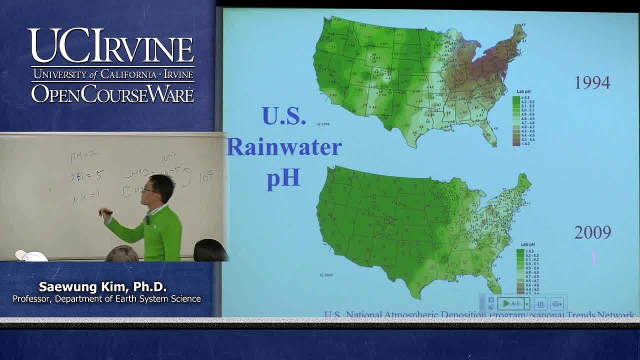 and then we talked about in natural rain has pH level about 5.5, which is about this range. So if it is green, that's natural condition, But if you start to see some faded green and then this red region, that's by definition acid rain, right. 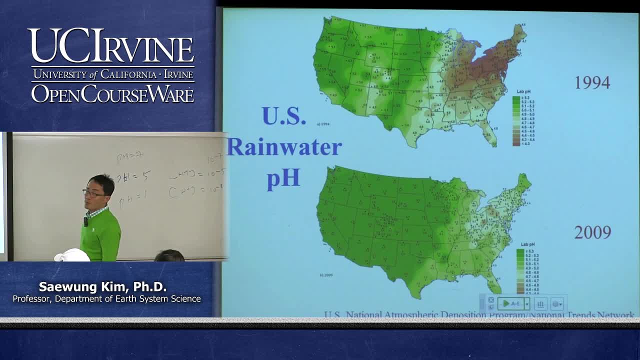 So, as you can see, we improved the acid rain problem quite a bit by removing SOT emission from power plants. So 2009 observation indicate that most of the country, even most of the eastern part of the US, southeast part and then this Ohio Valley region, 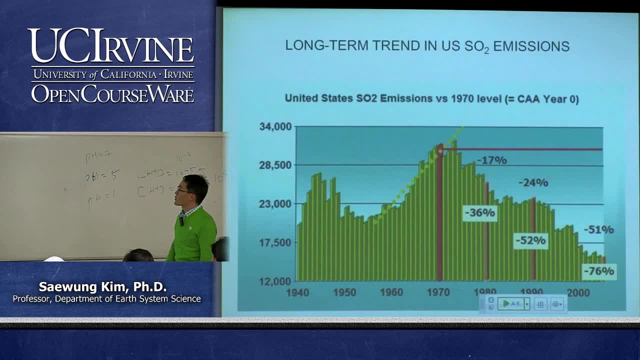 improved quite a bit in terms of the pH level of the rainwater. So how we can achieve it. Then, as I discussed in terms of, if we set the 1970 level of the SOT emission as a reference level, we knocked down SO2 emission by 76 percent by adapting new technology. 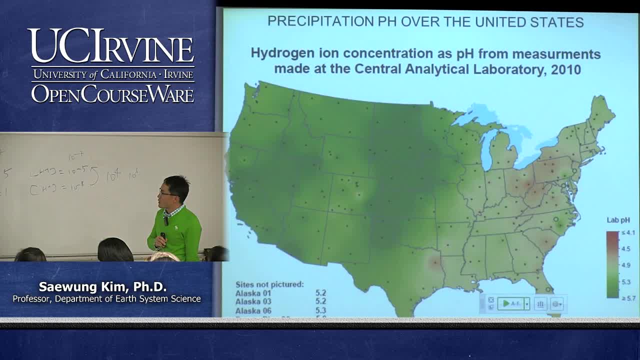 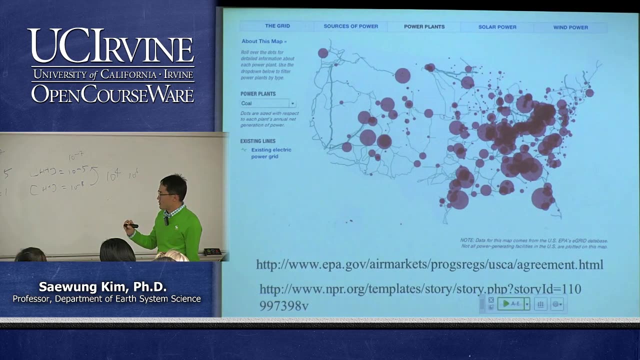 So this is, I think, 2010 most recent observation. So still there's some lower pH observed in the Ohio Valley and then southeast part of the US, but it gets improved quite a bit. So if you compare, still so this is the power plants distribution all over the country. 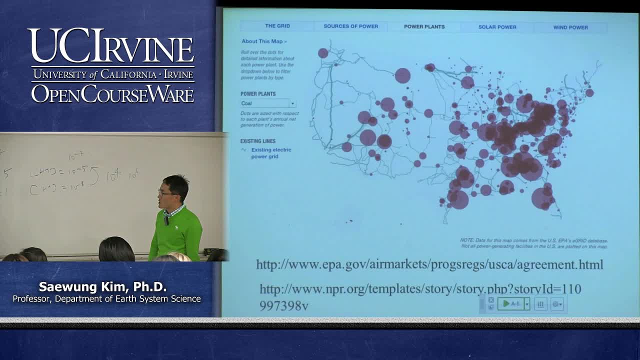 So a different size of this circle means that how much electricity each power plant generated. So you can see that this a lot of power plants- coal burning power plants- located in the Ohio Valley, Ohio Valley region, some in eastern part of Texas, then southeast part of the US. 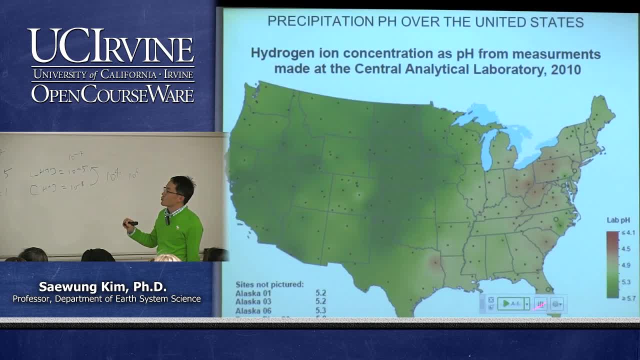 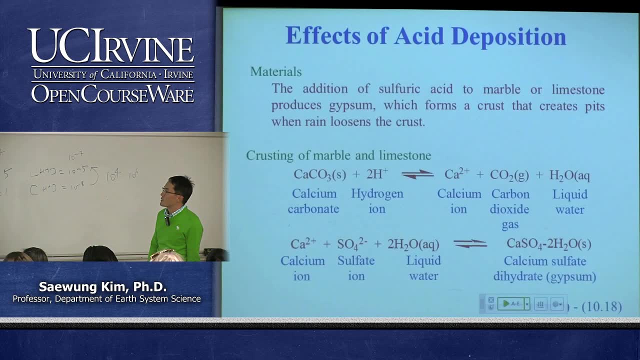 So basically you can see the correlation between lower pH and then higher electricity production from the power plant. So we already discussed about this thing. So a lot of kind of a historic statue, things like that, as made by the marble and limestone. and then, if you take a look at the chemical composition, 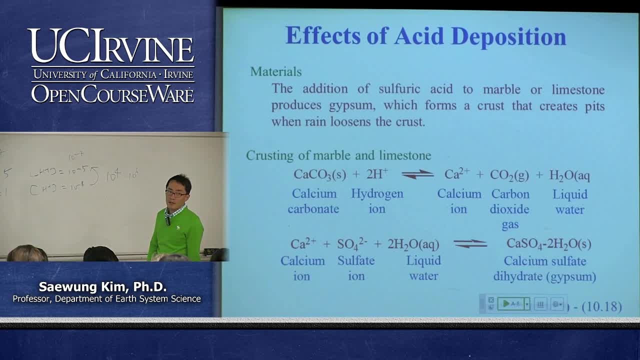 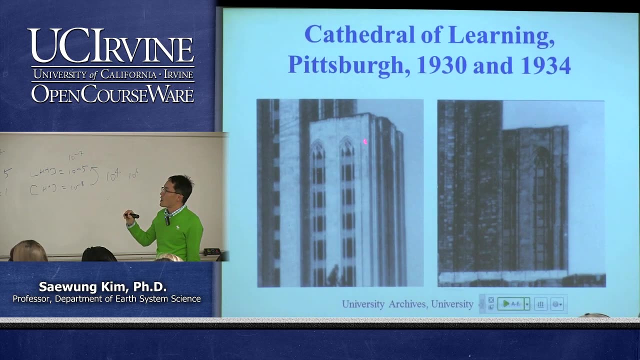 of the marble and limestone. that's all calcium carbonate, and then they can be dissolved by this hydrogen ion. So basically, high pH water, acidic water, can dissolve this calcium carbonate which is marble and limestone. So you can see that outside of the marble and limestone, 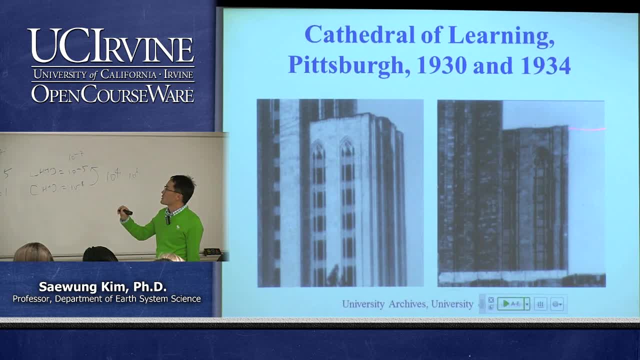 can be eroded by this acid rain. So this is early 1930 in Pittsburgh, when acid rain gets a problem. when acid rain gets a problem, there's more acid rain, that gets more acidic and acidic and acidic. A lot of building material got eroded, as you can see. 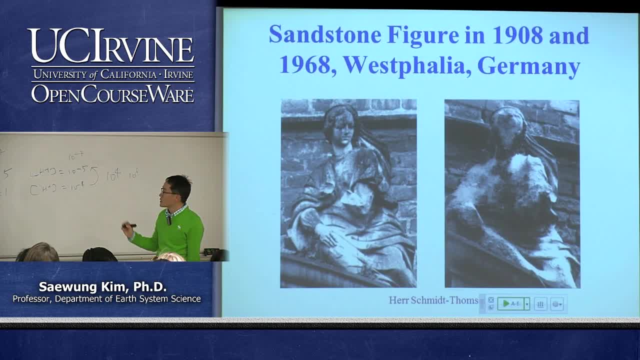 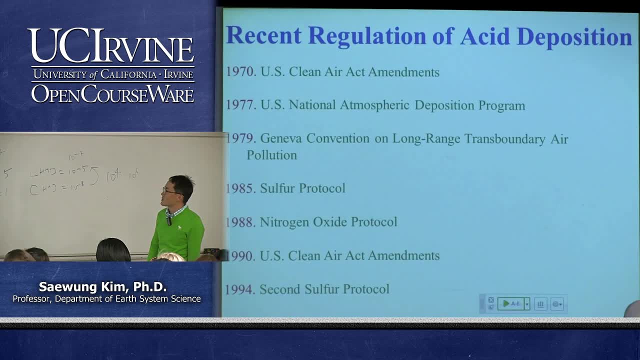 A lot of historic statue, So she basically lost her face because the acid rain. okay, So there's a couple of regulation, things like that, from the 1970s, So that's why we set the reference time point, as still, I have 10 more minutes. 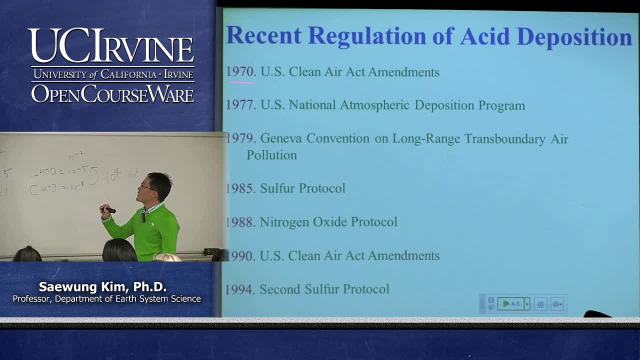 Wake up 1970, because we started regulation in 1970. So that was the highest point. So that was the highest point in terms of SOT emission. And then we achieved quite a bit thanks to that Clean Air Act, things like that. 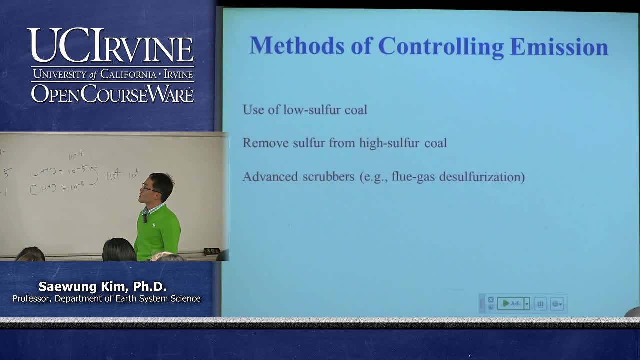 in terms of the reducing pH in the rainwater. So that's the specific method of the controlling emission: Use a low sulfur core And then from the starting material, we're using the core that has less sulfur And then, if there's some residual sulfur in the core, 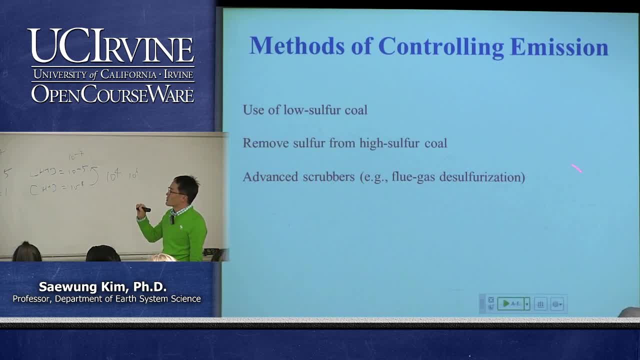 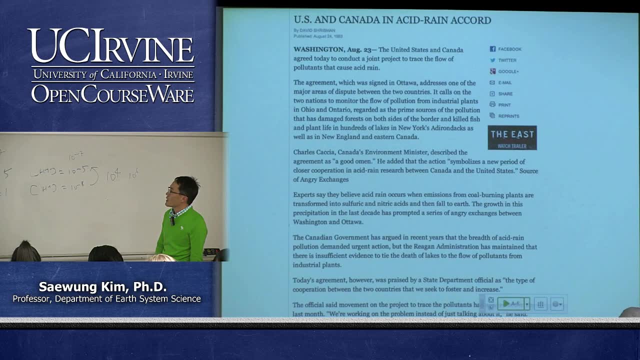 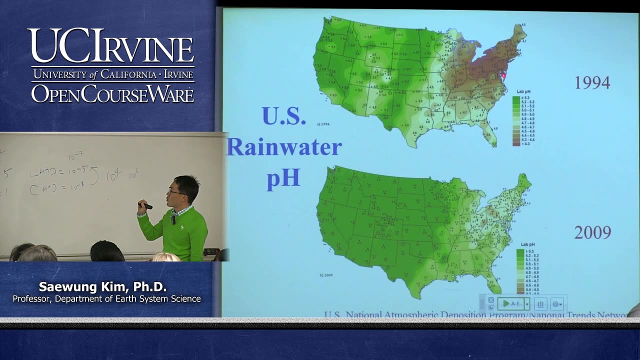 that should be emitted as SO2.. Then we just used some scrubber technology to reduce SO2 from the stack. So actually, if you take a look at this pH distribution in 1994, there's a lot of low pH acidic rain. It's located in a wild valley region, happened to be faced with the Canadian border And then from the early 70s it was a big problem with the US and Canada. So Canada basically is blame, the US side. 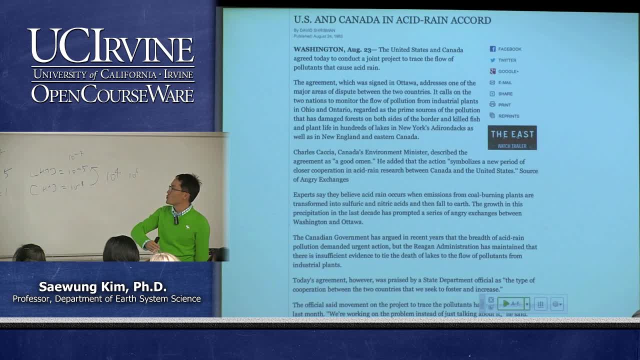 Their acid rain problem actually is transboundary SO2 make their acid rain and then they just fought over over 10 years And then finally, in 1983, they reach an agreement, They got a study together, things like that. So once that problem, that the solution. 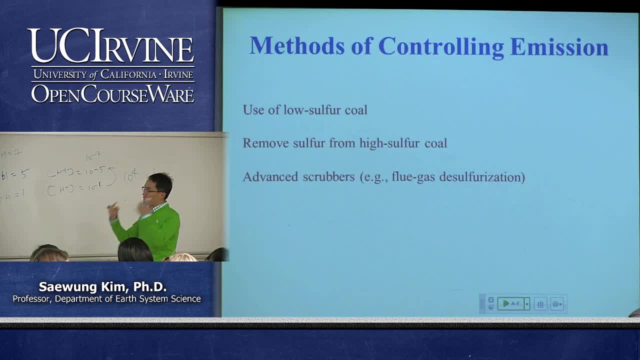 of the SO2 emission control, that the solution of the SO2 emission control, that the solution of the SO2 emission control. this came and then adopted the technology. Then we don't fight about this acid rain anymore, at least US and Canada. 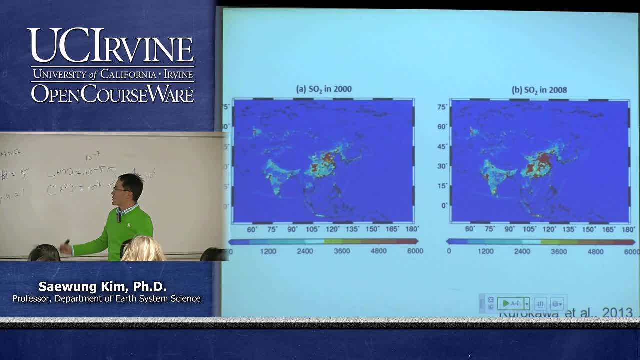 But if you take a look at the wide, larger scope, some part of the world this SO2 emission is still problem. So this is it's hard to see. but basically this is East Asia, So that's China, So that's Korea, tiny country where I'm from.